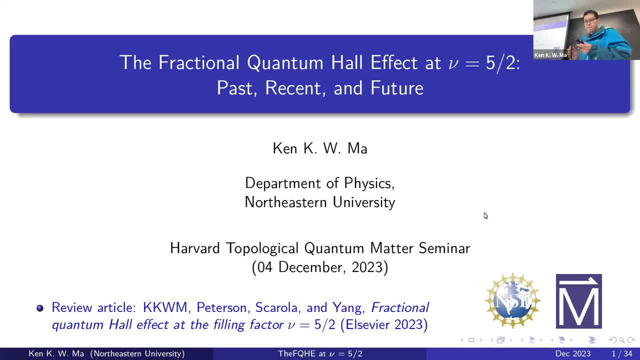 Hi everyone, welcome to the CNMSE topological quantum meta-seminar. So today we are very happy to have Ken Ma from Northeastern University to tell us about practical quantum house data at two-fifths- past, present and future. I can also talk about two-fifths if you want. 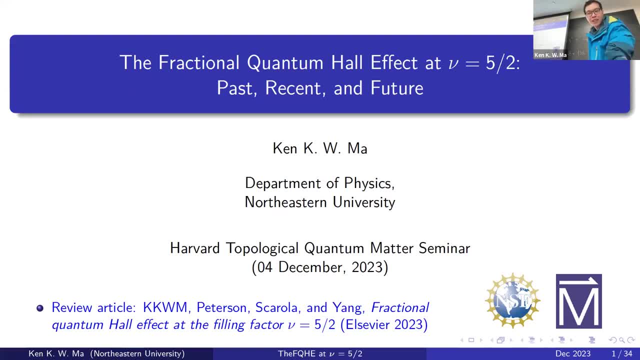 Yeah, the story of five-fifths, but I can also share with you about two-fifths, yeah, if you want. yeah, So, yeah. so, of course, the first thing, I need to thank Jeff for organizing this, and then thanks for inviting me to come here and then give you- I mean, give me- an opportunity. 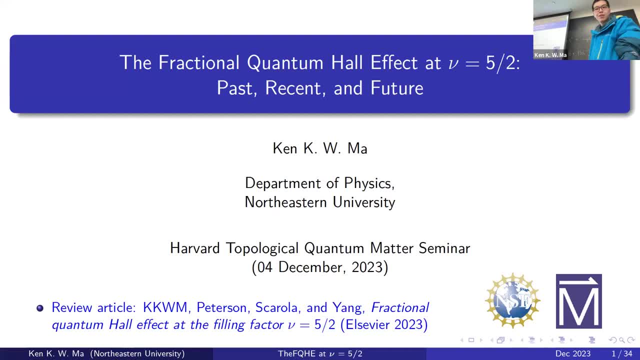 to share with you my limited knowledge on fractional quantum hall physics at the fueling factor five-half. yeah. So I don't know how many of you have a background in fractional quantum hall physics. yeah, so this topic is relatively old because fractional quantum hall effect at five-half, let's say, in gallium arsenide heatwork structure. 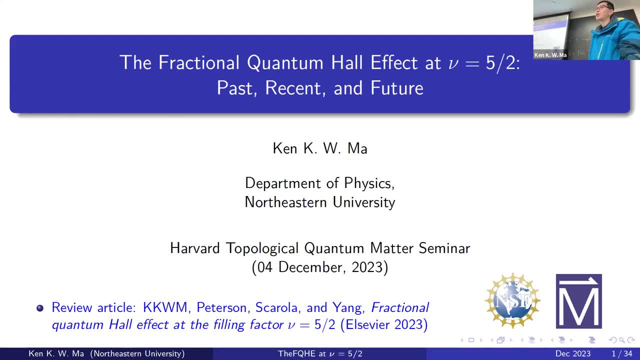 was actually first discovered in 1987, so it's more like 35 years ago. so that's why my sharing today to you may be a little bit different than most of the talks that you have heard about here. It's like an old topic, but I want to bring in some new insights and then 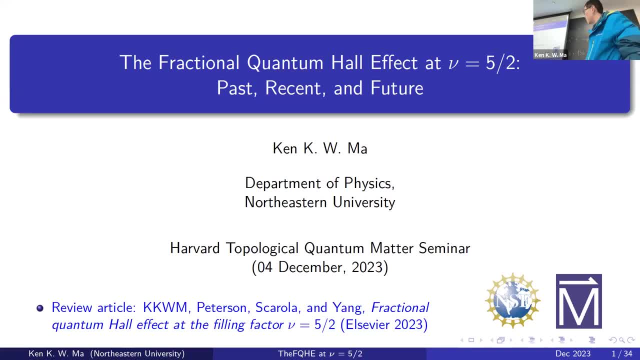 I'll tell you some more recent development. yeah, So, and then, actually, most of the information and most of the details, you can find it in this review article which I wrote with Mike Peterson, Vito Scarola and also Professor Kun Yang. okay. 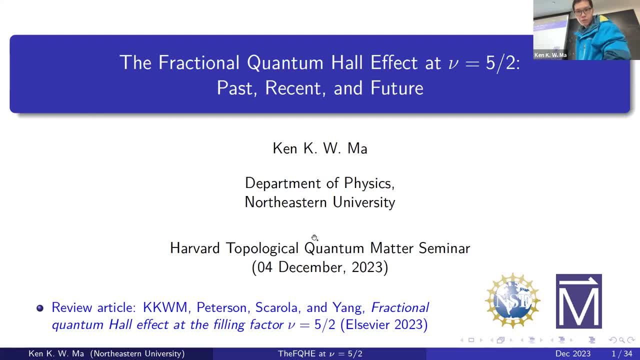 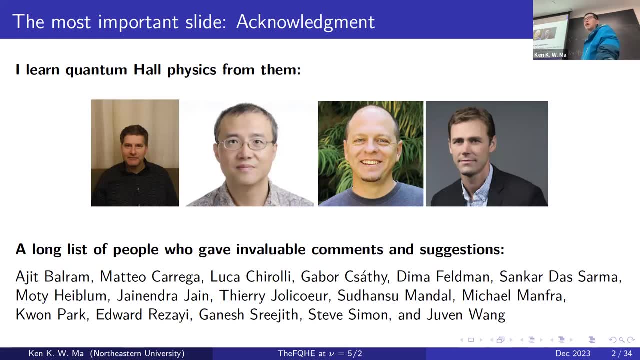 Yeah, yeah. so before talking about physics, so I need to share with you the most important slide here. So do you know actually how to move this bar? move this bar away? Yeah, so, before talking about the five-half state, I need to tell you about 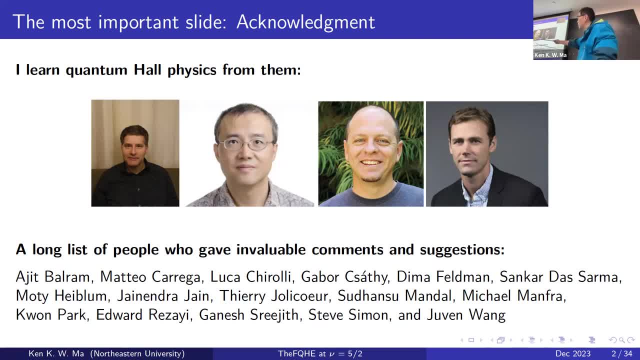 thing is actually, I learned my quantum of physics from these four professors. Then, of course, it was my PhD advisor at Brown University, And then most of the work that I will share with you actually knowledge coming from my PhD studies. And then I also learned a lot of quantum of physics from Professor Cun Yang at the MATLAB. 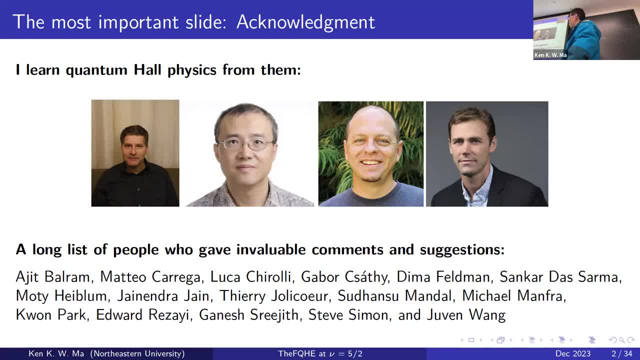 Yeah, And then when we wrote the review article, I also learned different perspectives of the five half state from Mike Peterson and also Vito Scarola. OK, And I also need to find, you know, a long list of people who gave very, very useful comments and suggestions to the review article. 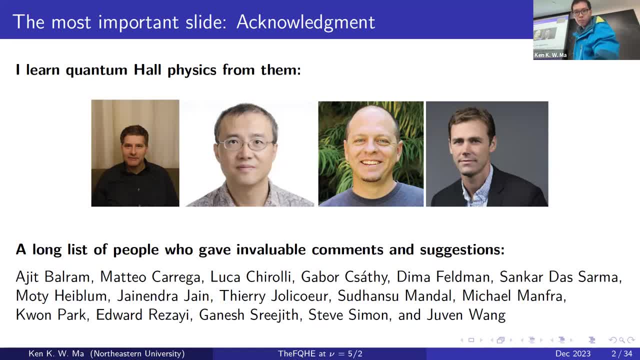 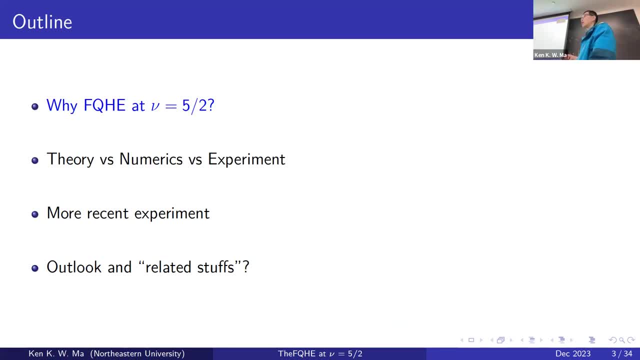 OK, Yeah, so my sharing will be divided Into our four different parts. Yeah, So I will first give you some basic idea why we want to study a fractional quantum state at the fueling factor. five half, Yeah, because nowadays actually more than probably 70 or 80 fractional compost states have been discovered at different fueling factors. 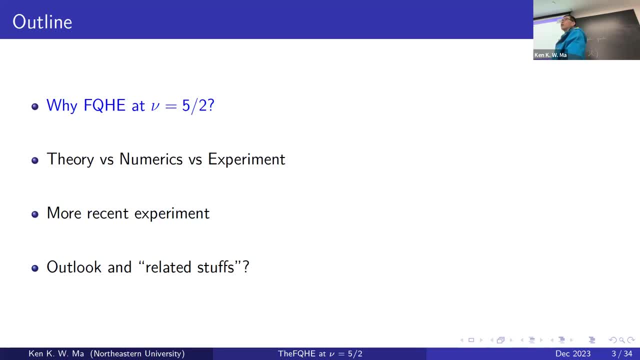 So a natural question to ask is why we care a lot about this particular fueling factor. five half Right. And then, after this basic introduction, I will talk about what we know about this state from theory, from numerics and then also experiments. 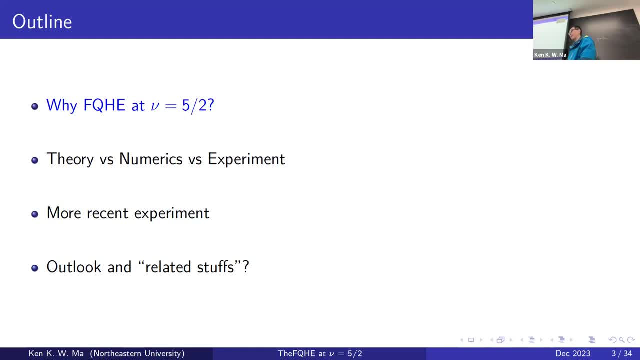 And then I will show you basically there are some discrepancies between them, And then I will tell you about more recent experiments and then which possibility or which topological orders is more favorable, And then I will tell you actually what we can learn about from those more recent experiments. 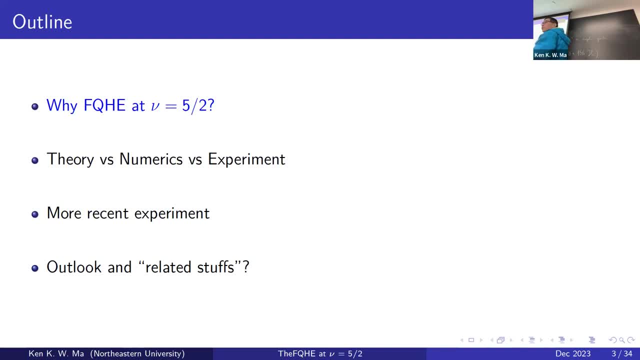 OK, And then at the end, if I have time or if you guys are still alive, not falling asleep, Then I will share with you what are some of the possible open questions and related questions that we can investigate in the future. OK, Sounds good, Yeah. 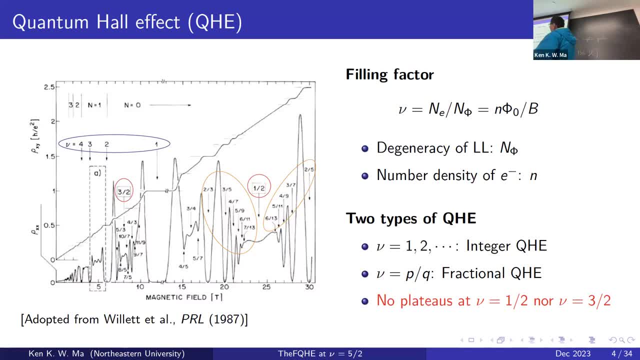 So let me quickly go through with you what happens here. OK, So if I give you, let's say, two dimensional electron gas, And then if you lower the temperature, let's say depending on which fueling factors, let's say to the millikelvin regime or several kelvin, 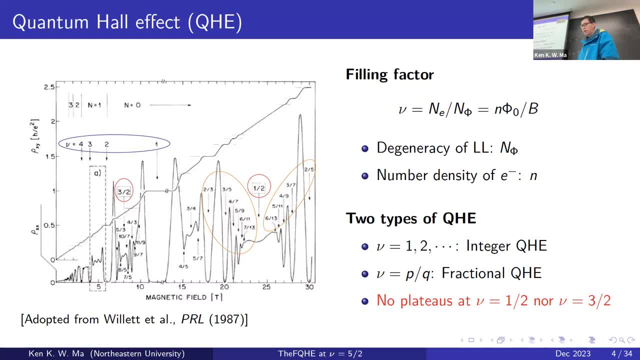 then you know when you have 2D electron gas. and then if you apply a strong perpendicular magnetic field, then the energy levels is quantized into Landau levels. But the important feature is that for each Landau level actually there is a large number of degeneracies. 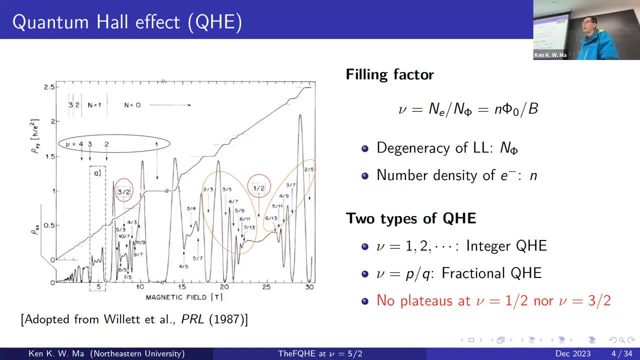 That number of degeneracy equals to the number of magnetic flux quanta passing through the sample. OK, And then the fueling factor is defined by the number of electron divided by the number of magnetic flux quanta passing through the sample. OK, And then on the left, here is actually an experimental result. 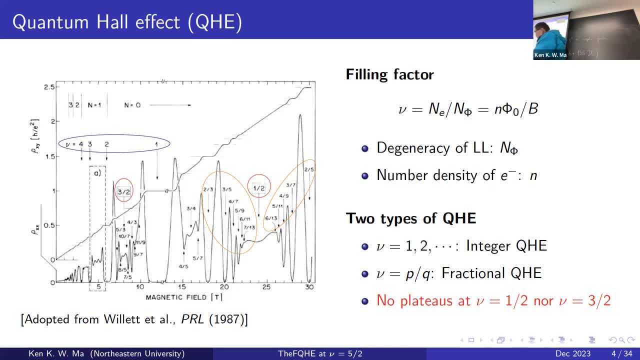 You see, it's from 1987, more than 35 years ago. But if you look at these experimental results you can see two quite interesting features here. First of all, if you look at the Hall-Ris activity, you see that there are several fueling factors here. 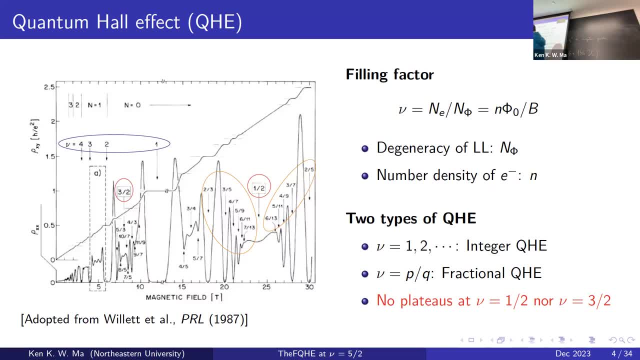 Let's say one, two, three, four. You see a petal here. OK, And then, at the position where you found these petals, if you look at the longitudinal resistance, you see a dip right. And these are the two defining features for observing a quantum-bore state. 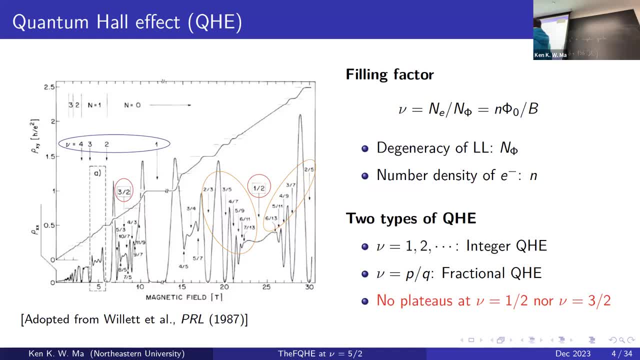 or a fractional quantum-bore state in the experiment. OK, And then, if you are a lot more closer to this figure, you see that the fueling factors actually have two different possibilities. I mean, one of the possibilities is that the fueling factor is integer. 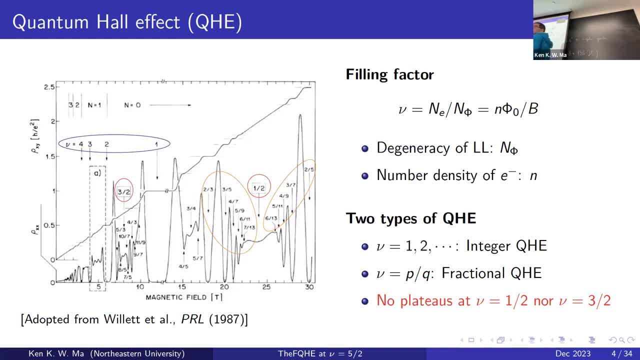 And then for this half-state we call integer quantum-bore state, And then it's much easier to understand that. And then another kind is that the fueling factors are fractions. That's why we call them fractional quantum-bore states. OK, 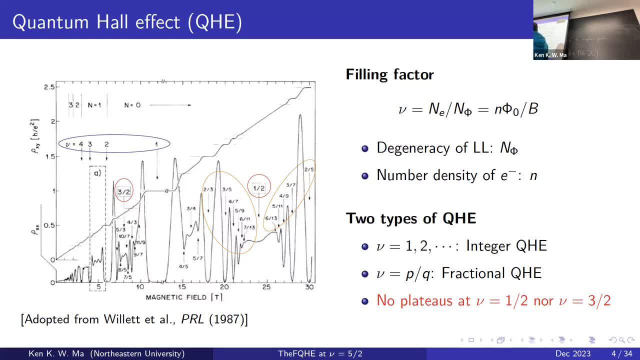 And then if we also look at the fraction more carefully, we see that most of them actually in this figure, basically all of them, OK, have all denominators right. And then at the fueling factor, let's say one-half and three-half. 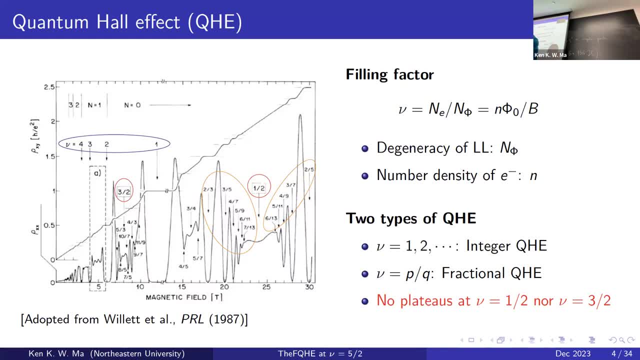 you don't see any petals in the Hall-Ris activity and then you don't see any dip, let's say in the longitudinal resistivity. So in this figure we basically don't see any fractional quantum-bore states. let's say at the fueling factor one-half. 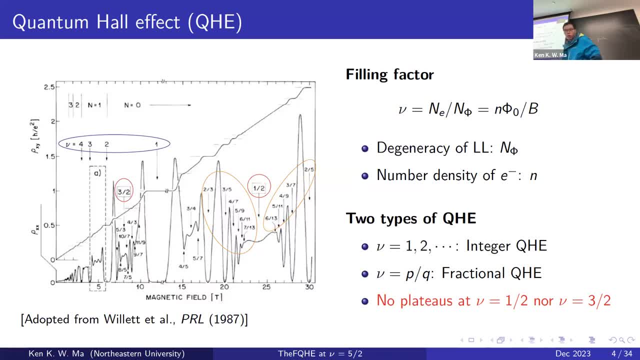 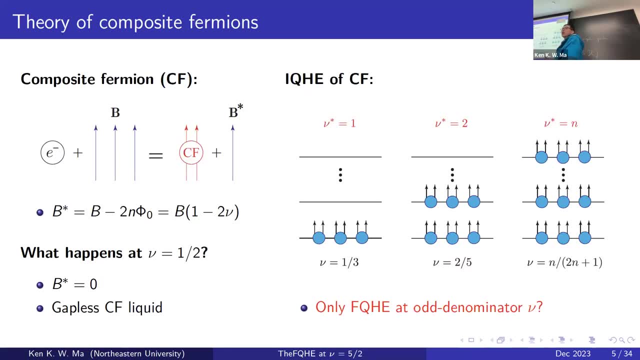 or three-half. OK. So the next general question to ask is: can we have a more systematic understanding of why fractional quantum-bore states exist? And then, if we have that more systematic theory, can we make that theory to predict why we don't see any gap states? 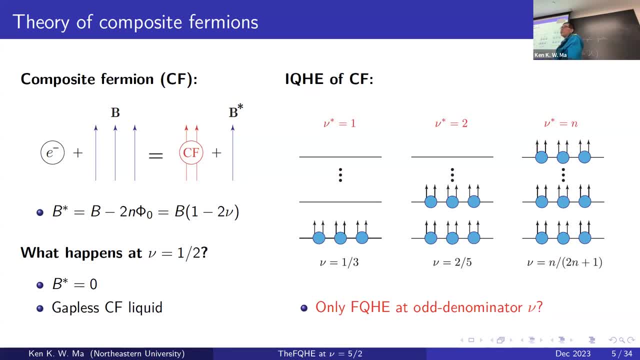 in particular fractional quantum-bore states where we don't see, let's say, at the fueling factor one-half or three-half. OK. So I think from, let's say from a solid-state physics class or many-body physics classes, 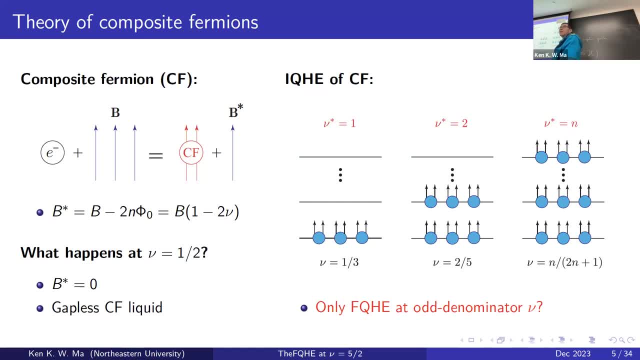 let's say, if I give you an interacting, let's say electronic system, sometimes it's much easier for you to study the system or describe the system if you can find a set of quasi-particles such that they are weakly interacting right. 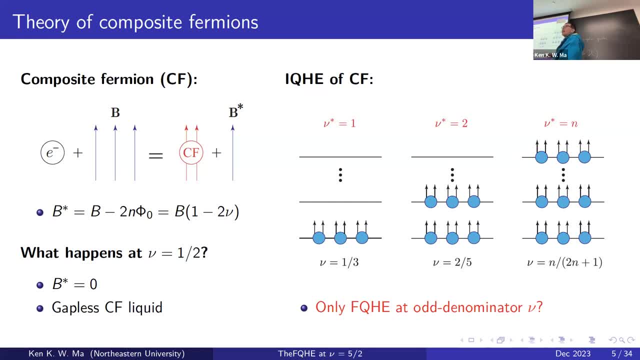 And then in fractional quantum-bore physics we try to think of what kind of particles, instead of the original electrons, that we can use such that we can turn it to a weakly interacting problem. let's say, The reason is that because in the Landau level 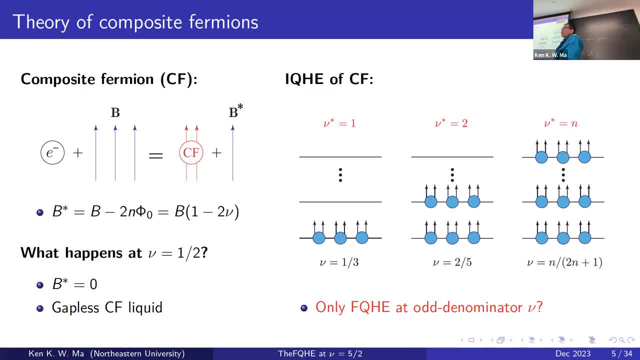 basically all the kinetic energy of the electrons are completely quenched. OK, That's why all the important physics or interesting properties of your physical system actually comes from the Coulomb interaction. But because the kinetic energy is completely quenched, therefore you don't have any small parameter for you to do perturbation theory. let's say: 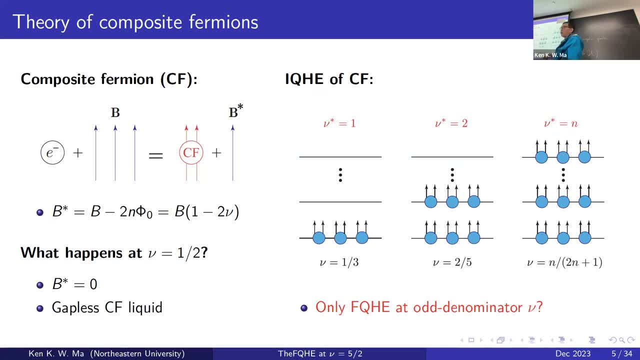 That's why it's a very, very challenging problem to study fractional quantum-bore. That's why we want to identify some sets of particles, so that we can turn this problem to a weakly interacting problem. let's say: And then in fractional quantum-bore physics, 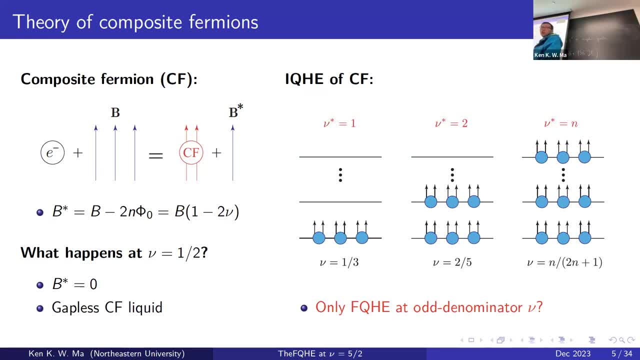 that particle are actually composite fermions. So what is a composite fermion? So, generally speaking, a composite fermion is formed when you attach an even number of magnetic flux points to an electron. OK, And here I show you the example, that you attach two magnetic flux. 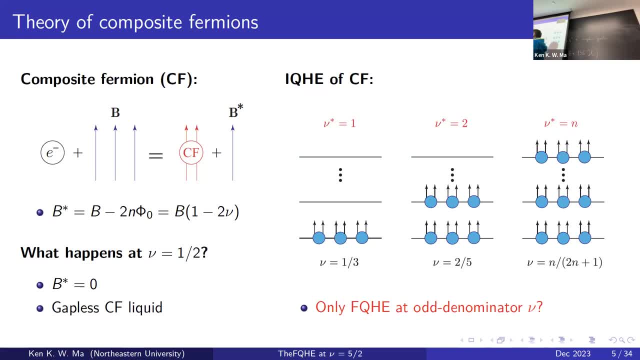 to an electron: OK. And then you turn it to a composite fermion: OK. And then the reason: And then you can't use that because some of the, Because some of the Some of the magnetic field is already being attached, or a magnetic flux point has been attached to the electron- OK. 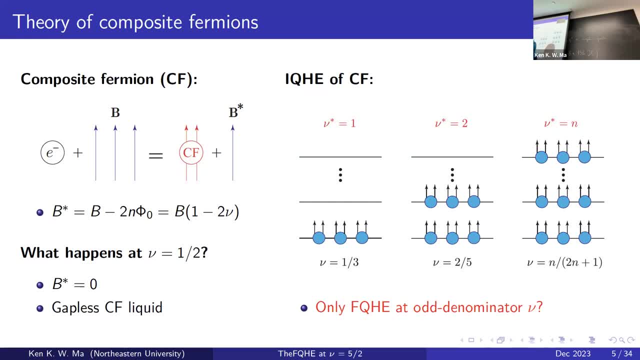 That's why the effective magnetic field experienced by the composite fermion is actually reduced. OK, And then if you go through the mathematics, you see that the effective magnetic field experienced by the composite fermion is actually satisfied. this equation, OK. And then let's say for the Lafley state of fielding, factor one-third. 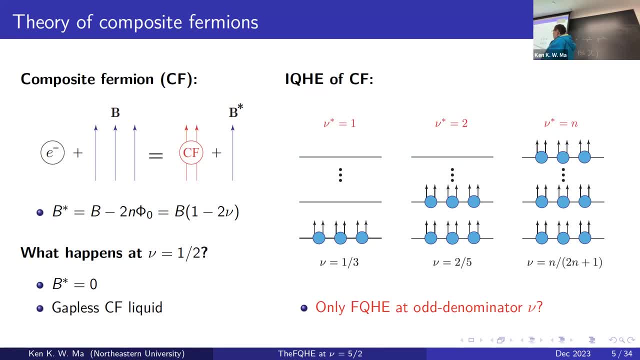 what does it correspond to? It corresponds to You just fill one Landau level for the composite fermion, OK, And then if you fill two, If you completely fill two Landau levels for composite fermion, then you will get actually the threshold quantum loss state. 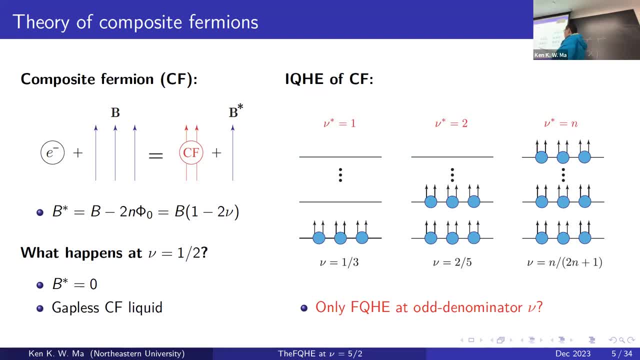 at a two-fifth that you mentioned, right? Two-fifth? OK, Yeah, And then? But if you just, If you just rely on this construction, then basically there's no reason for you to get any even denominator fielding factors here. 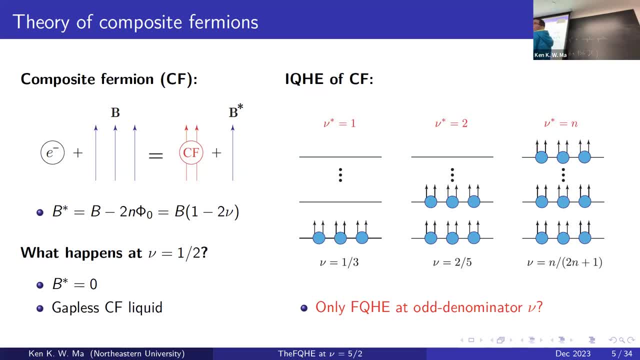 And then if you look at the fielding factor, let's say one-half, the effective magnetic field actually vanishes, because if you put new equals to one-half, then you see d star goes to zero. Then I will ask you a follow-up question. 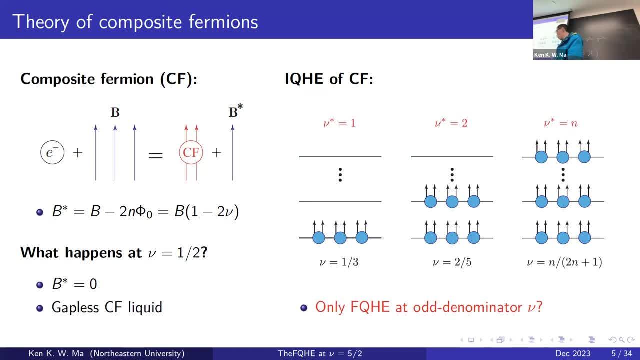 Let's say, if I give you a bunch of fermions, OK, And then if they don't have, And if they don't fill any magnetic field, let's say on average, then what is the lateral ground state, right? And then from basic quantum mechanics, 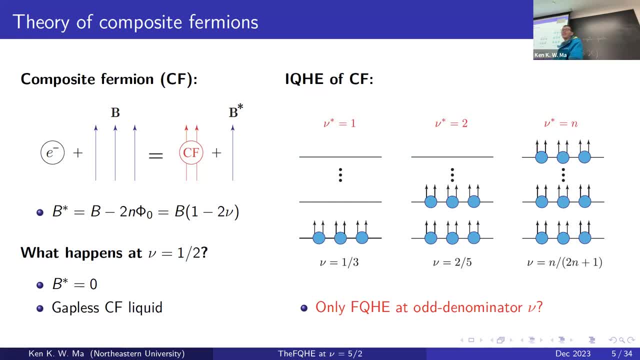 you know that you just want to pile up. you know two-fifth right, Pile up, you know, let's say, a single eigenstate, and then you pile it up and then form a Basically form, a Fermi surface right. 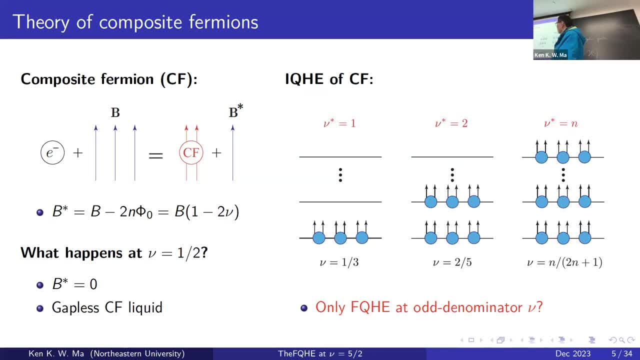 That's why that state is gapless, right. And then this actually explains why the fielding factor nearly equals to one-half. You actually don't see any gap state OK, And this is actually a very strong support to the so-called high-frequency field, OK. 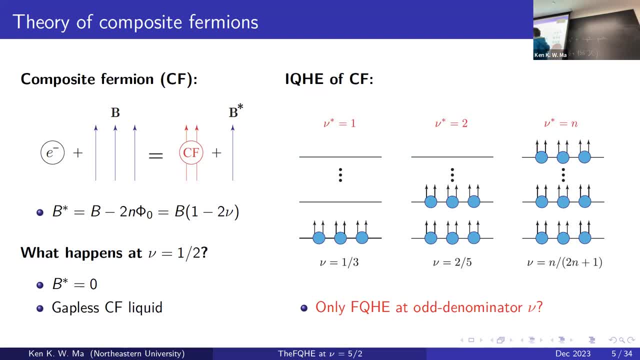 Yeah, But of course I, But of course these composite Fermi network is very different than the usual Fermi network, OK, Which I will not go into details in this talk. OK, So the question is a fractional quantum Hall state. 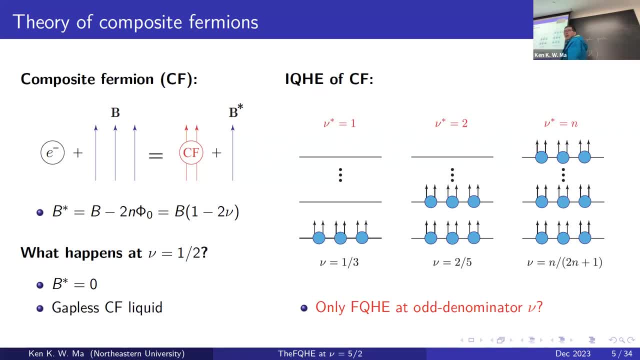 only observed, let's say, at off-delimitator fielding factors. If the answer is yes, then I shouldn't come to this talk, right? Because my topic is fractional quantum Hall effect at fielding factor five-half right? That's why there must be 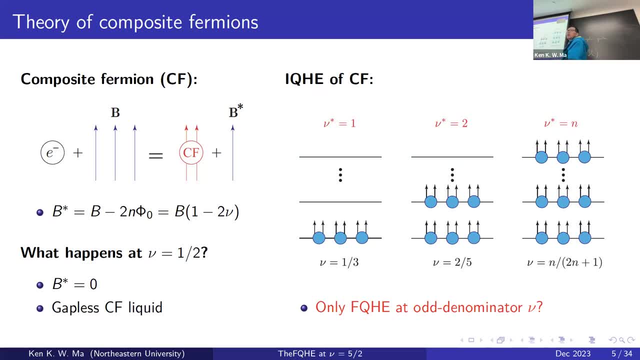 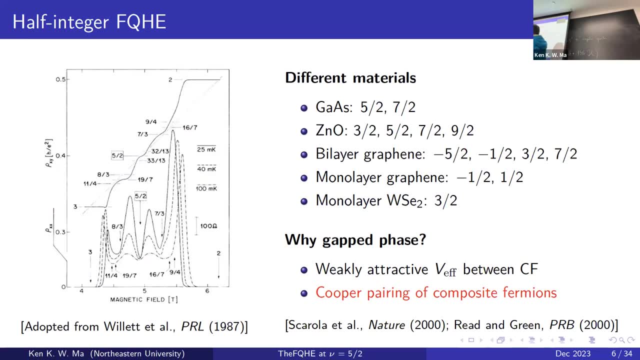 fractional quantum Hall state which can be found at even-delimitator fielding factors. OK, Now if we look at the experimental result here, now if you look at the longitudinal- Sorry this- The Hall resistivity, you see a very, very thin pattern here. 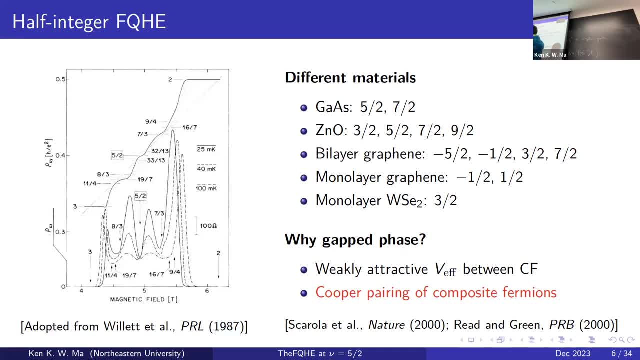 But at the same time, and at the same time you also see a minimum here, right, And, as I said, these are the two defining features of fractional quantum Hall states. OK, That's why this figure really tells you that fractional quantum Hall state. 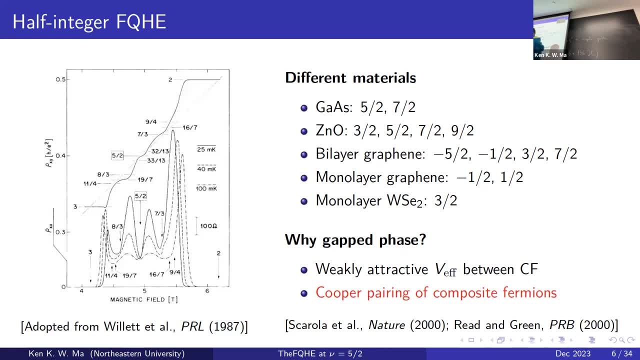 actually exists at the fielding factor five-half right. But in your previous slides I tried to convince you that the defective magnetic field experienced by composite thermon actually vanishes at one-half, And then for five-half it's actually two plus one-half right. 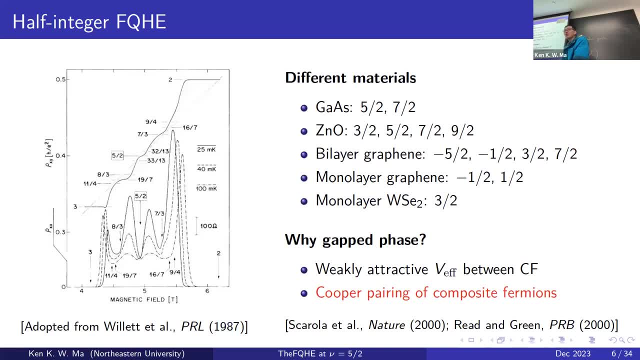 And then in the zero-order approximation, what we usually do is we drop that two completely field-landau levels and then if we just focus on that half-field-landau level, then probably you would still expect it should be a gapless state, right? 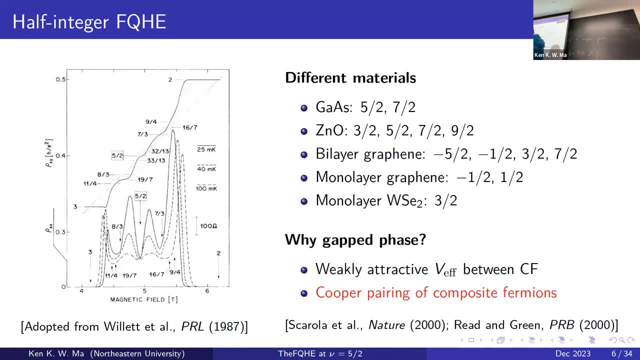 But here experiment tells us that it is a gap state. OK, So how can we explain it? And then, even more strikingly is that after more than 35 years, actually more half-imager fielding factor quantum Hall state have been observed in different materials. 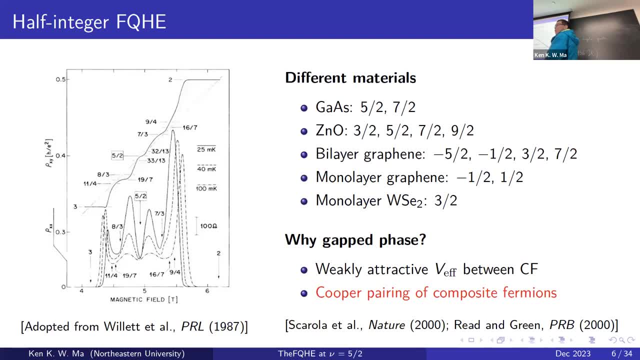 not only in gallium arsenide, that's in zinc oxide and then both von Ohle and baryl graphene, right, And then actually also in transition metal, disorganized. we also see even denominator fractional compound state. So it motivates a very literal question is: 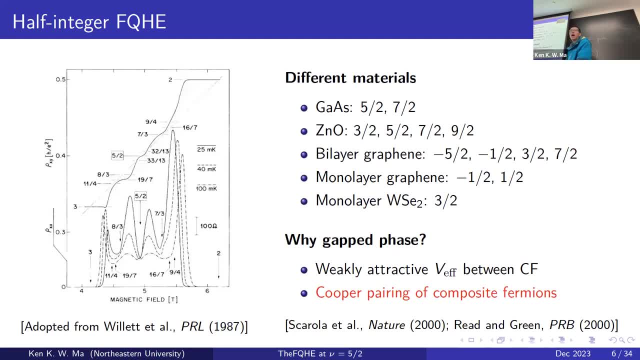 why we actually can have fractional compound state at half integer field-land factors OK. So the key difference here is that in the lowest-landau level, OK, when you really calculate, let's say, the effective interaction between the composite fermions. 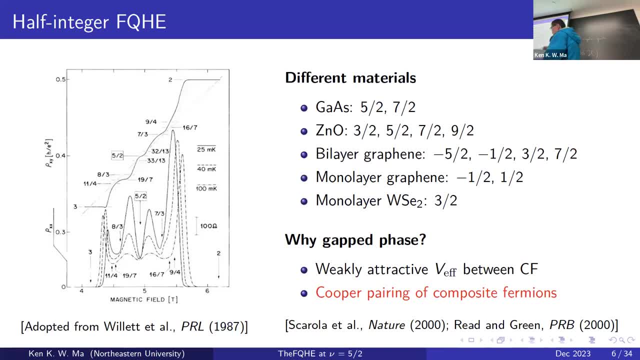 they are always repulsive, OK, But if you already have a Fermi C and then you pile up a composite fermion or electrons in the first-landau level, then actually from numerals people found that the defective interaction between the composite fermion 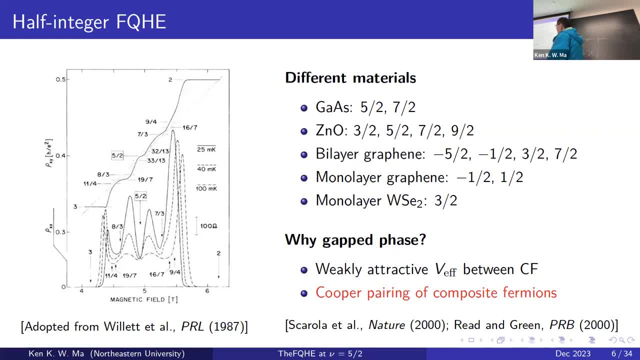 can actually become attractive. OK, And then, due to this weakly attractive, defective interaction between the composite fermion, it can trigger a Cooper instability between the composite fermions. That's why these composite fermions can pair up and then, once they pair up, 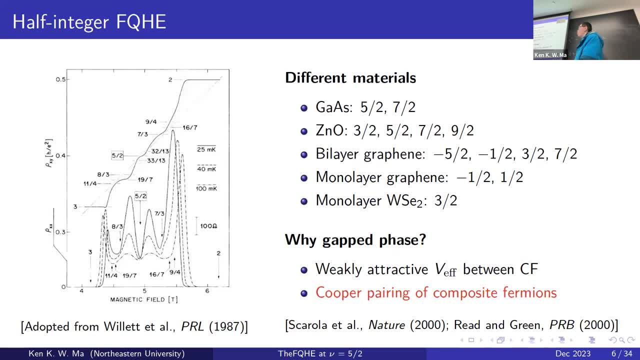 it becomes a gap state and then this explains why fractional compound state at the field-land factor of five-half can happen. OK, And the key is that the effective interaction between the composite fermions in the lowest-landau level and the first-landau level 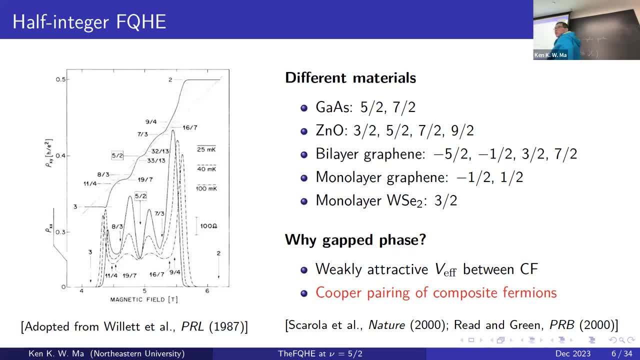 can be different. OK, Yes, so that's all good. So you mentioned the numerical. you say the effective interaction between the compounds are attractive. Yes, How to get this effect? How to get this effective interaction? They probably not really show. 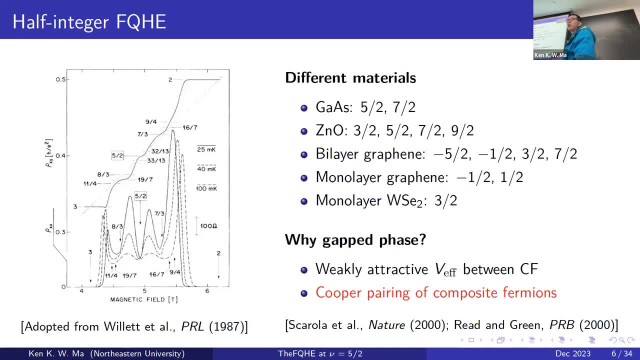 the effective interaction They are calculating by the binding energy when you add two more composite fermions there and then see whether the energy get lower or higher, something like that. Yeah, It's like over-screening. They claim it's like over-screening. 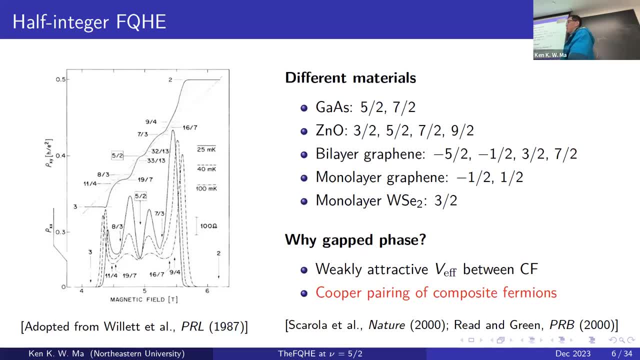 because the landau level wave function, I mean the wave function is different in the lowest-landau level and the first-landau level. So that's why it can trigger, like over-screening of the Coulomb interaction, such that the effective interaction 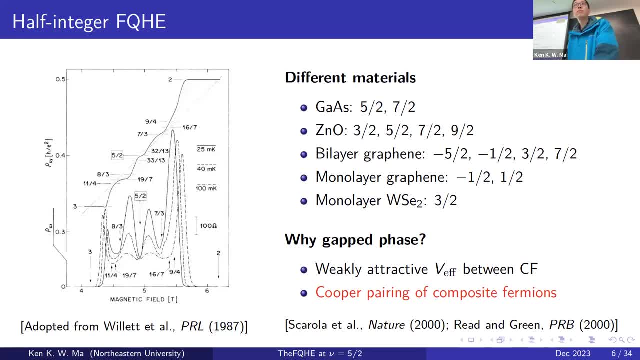 becomes check. Let's see Who's the microphaser Hm. Who's the microphaser By Scarola and then also by John Andrew Trang, I think. Yeah, I think there's also another one. Yeah, I can find it out later. 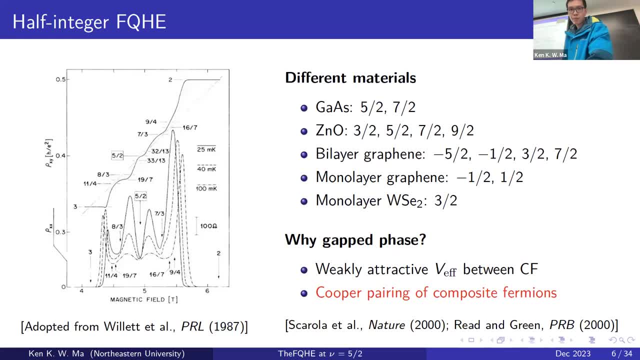 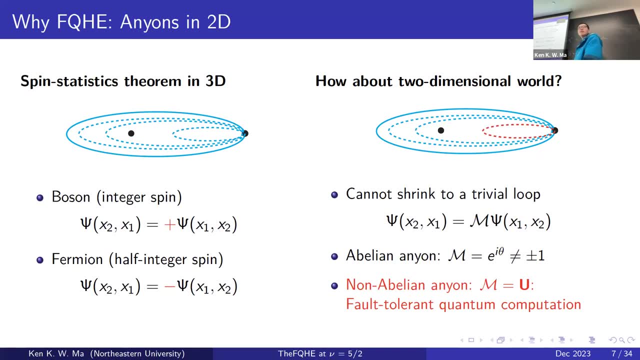 Yes, Yeah. So I tried to convince you that we have a fractional compost stage at the fueling factor 5-half. Then you may ask me, while you're thinking, why we care about it, right, Why we care about fractional compost stage. 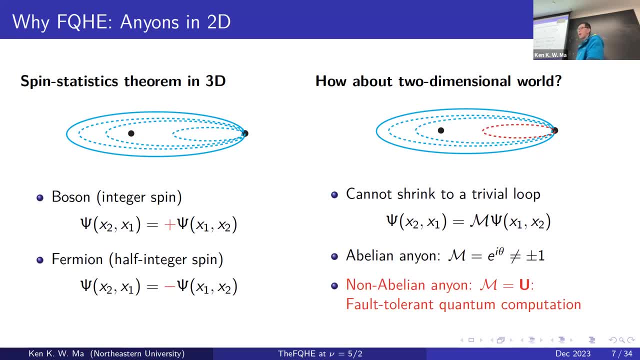 at fueling factor 5-half, Or you can actually go one step backward. Why we care about fractional compost stage at all? right, It's just a phase right. The reason is that because let's say in three dimension, let's say three dimension. 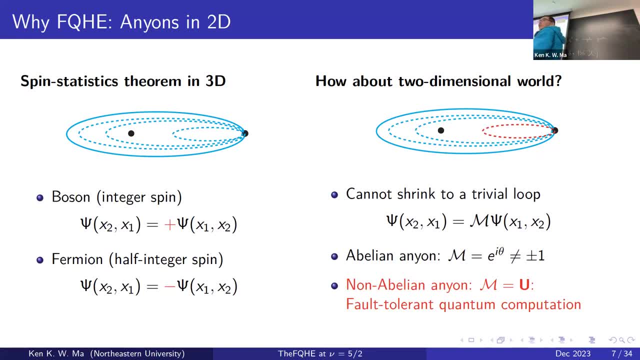 means three dimensional space. okay. If you're a high-energy physics person here it means 3 plus 1d, okay, Space-time okay. And then if you talk about this three-dimensional space, then you only have two kinds of particles, okay. 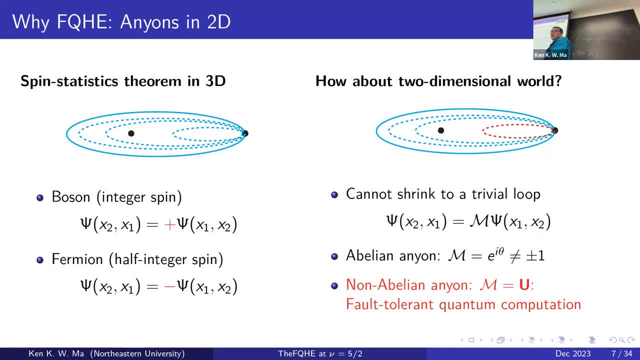 You can only have bosons or fermions, okay. The reason is that when you exchange two identical particles, okay, it will apply a phase factor to the wave function. But this phase factor is more like a topological quantity, The phase factor you make. 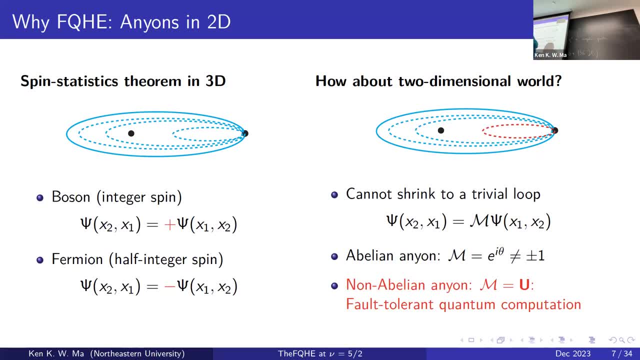 and change, if you can. let's say, deform this loop smoothly, okay, without cutting it, okay. But now, in three dimension, you can always change this loop back to a point. okay, Because let's say, you have two particles. 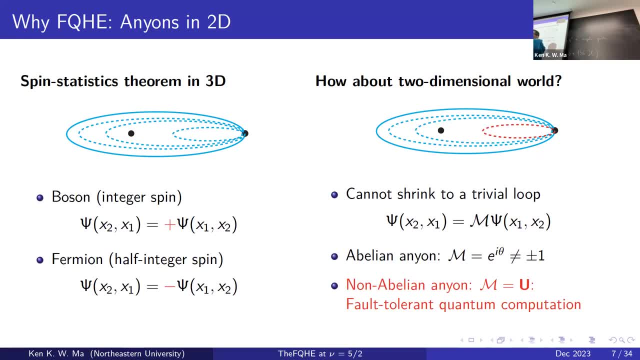 on the x-y plane. okay, You can lift up the loop, let's say in the c-direction, okay, And then lift it away from the x-y plane, and then eventually you can change the loop back to a point okay. 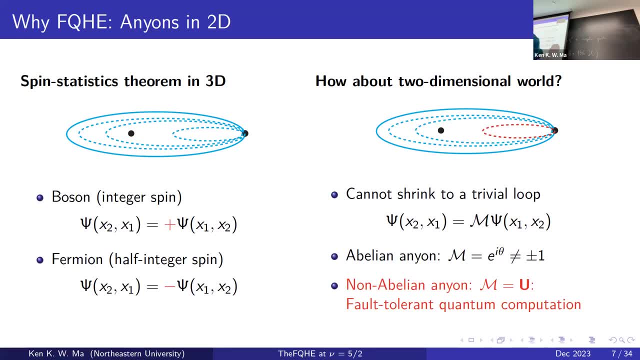 That's why the effect of going around is always at the top one. But if you exchange it, it's more like a half of the phase, something like that. That's why you can have a plus or minus only okay. That's why you only have 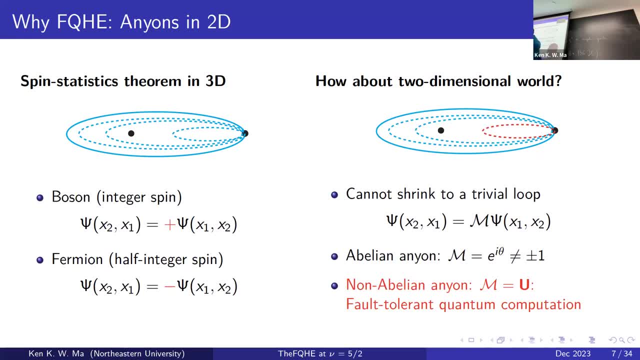 two kinds of particles. They are bosons and fermions, okay, And actually in higher dimension it's also two cases okay. But in 2D the story becomes very different, because now I don't have that c-direction okay. 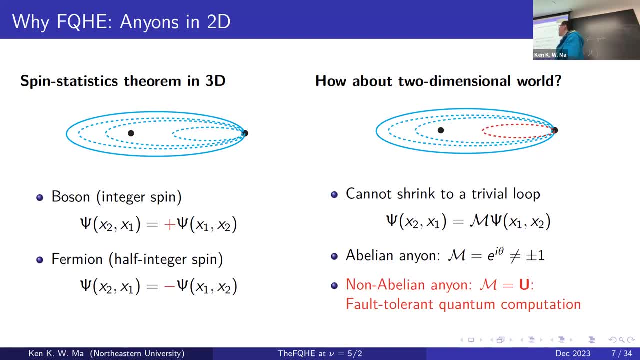 Let's say I want to change this loop. okay, Let's say the original loop is the blue solid, right here. okay, I can deform it, let's say to the blue dash, right here. but I don't want to change it. 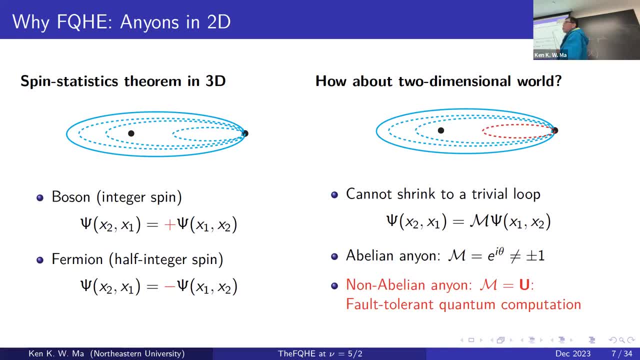 but I cannot pass through this point and then change it to this red dash loop: okay. That's why I cannot follow the argument in the three-dimensional case and then say that I only have two possibilities Now. the phase can be any value. 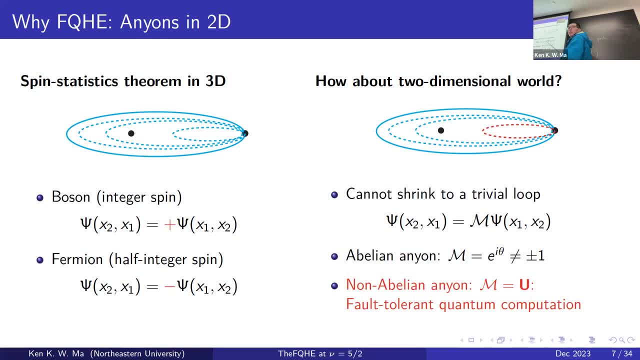 let's say in between zero and pi, And then if it is really a complex number, then we call this one abelian anion. The reason why it's called anion- because it is a phase vector- can be any value in between zero and pi. 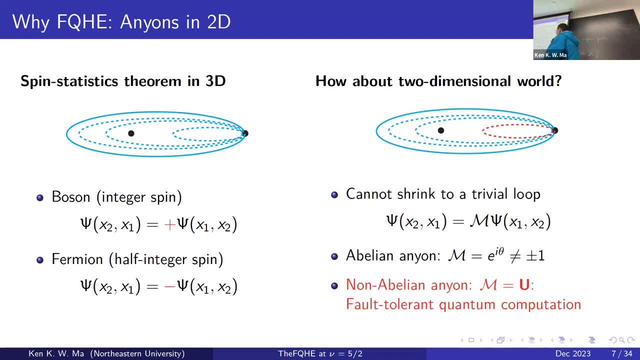 okay, That's why this one is abelian anion. But even more dramatic cases can happen if the ground state of your system has degeneracy. okay, Then, when you exchange two identical anions, what is? the accumulator is not only a C number. 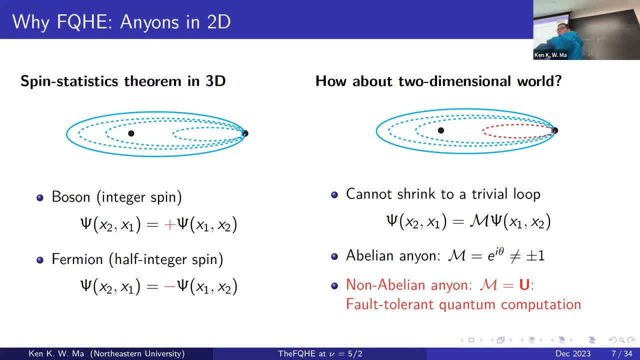 in the wave function. What you can do is a transformation in this ground state subspace, okay, So you can have a three matrix here, okay, And in this case, what you get is something called the non-abelian anions. 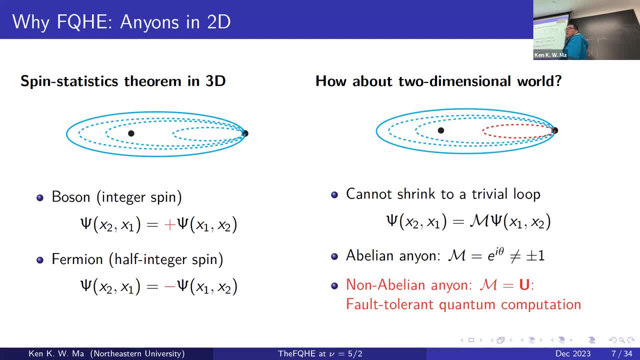 because when you exchange it, let's say more times, or if you have more than two anions, let's say four anions, and then you do the exchange. but you know that the multiplication between matrices they are in general, you know. 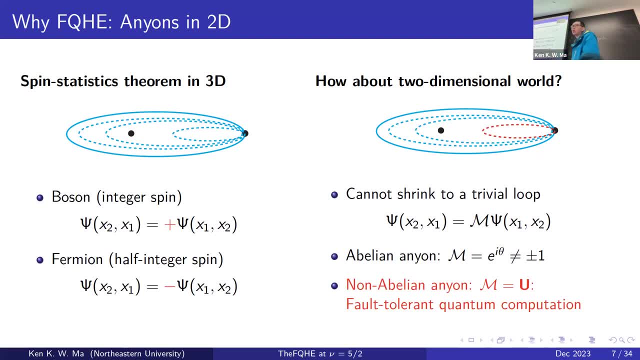 you can give you a fundamental building block of four columns: quantum commutation. okay, Because you know in quantum commutation a very big hurdle is how to avoid, let's say, having error and then try to do all kinds of error corrections. 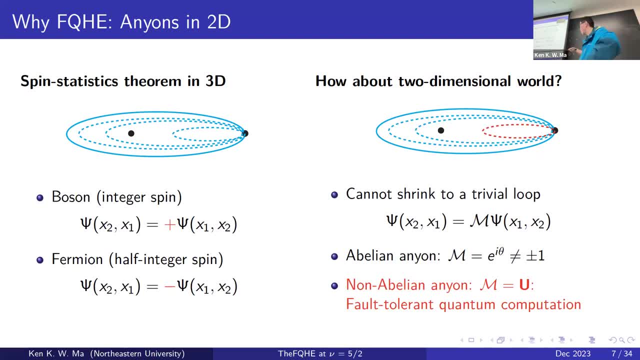 right, But you know it's very costly. You need to have a large number of qubits in order to protect a small number of logical qubits that you want to have. But if your system is already protected intrinsically and then 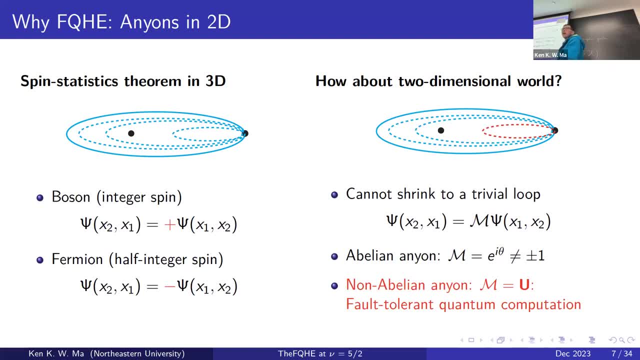 I will show you actually, in fractional quantum state of five, half some of the proposal to describe that state actually can hold non-EBN anions And that explains why we are so interested, let's say, in fractional quantum physics and in particular. 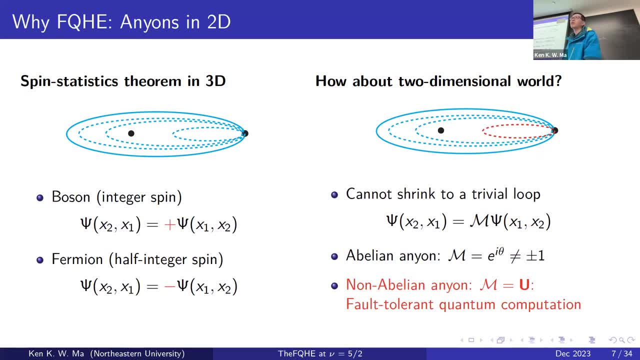 why we are so interested in fractional quantum state at the field of the five half. Is that okay? Yeah, What do you experimentally make of this matrix? What's really cool about what we're going to do in the moment? Good question. 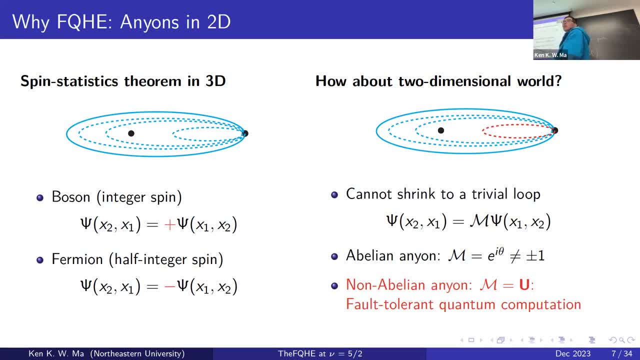 So I don't know actually how you can really measure this matrix. let's say, But if you do some interferometry experiments, probably you can distinguish these two cases. Yeah, But if you really want to map out this matrix, 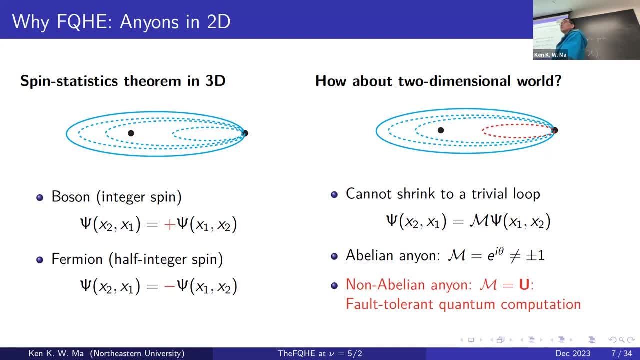 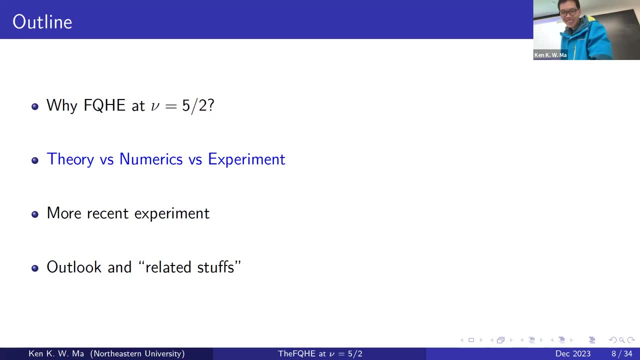 then I don't have any good idea. Yeah, I can think about it more, but I don't know. Yeah, Maybe, Yeah, you can ask him directly. Yeah, This gap, this gap, because it's a quantum state. 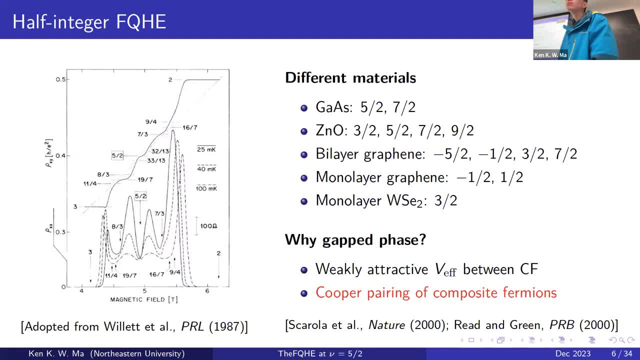 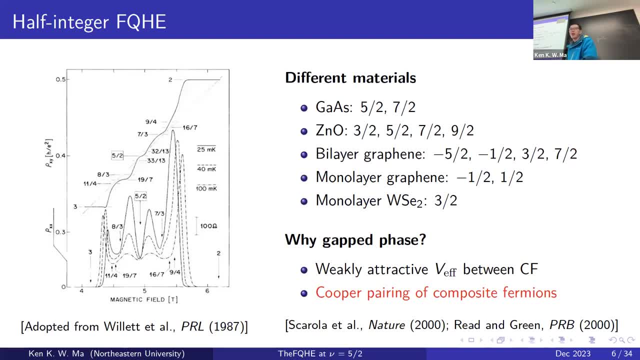 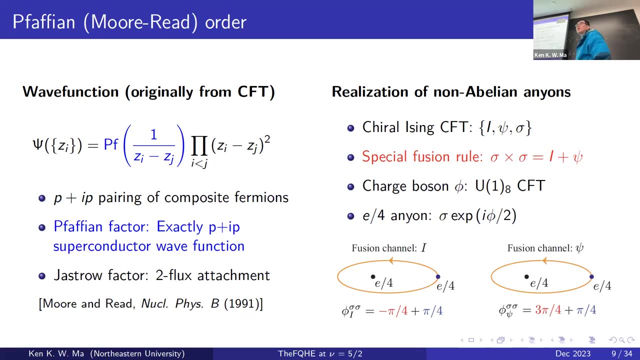 if you really have comments, I see, Yeah, But I'm quite sure that if it is really quantum state and the state should be gap, Yeah, Okay. So Yes, you mentioned that this one is more like the whole, the whole. 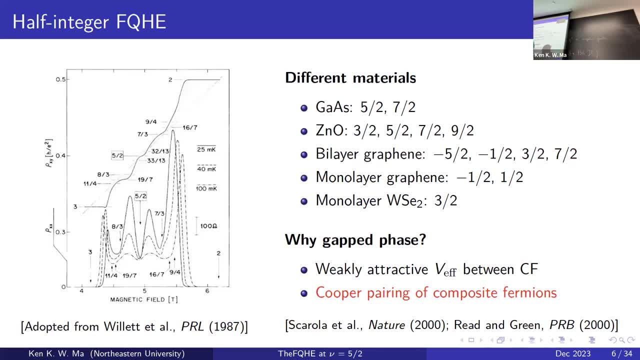 That's why it actually has a is not very strong, because this one is like an experiment from 1987, but having this type of is not. you know, it's not. I would say it's not definitely enough. That's why we also see the. 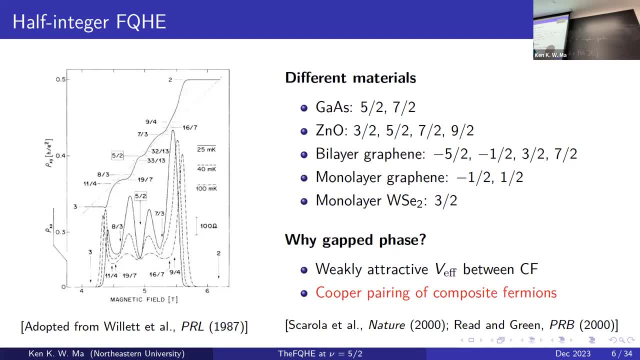 dip here. but you can never go really go to zero, right, Because in realistic sample you cannot really have longitudinal resistance going to zero. But if you compare to something nearby you clearly see a dip here. That's why the combination of these two features suggesting 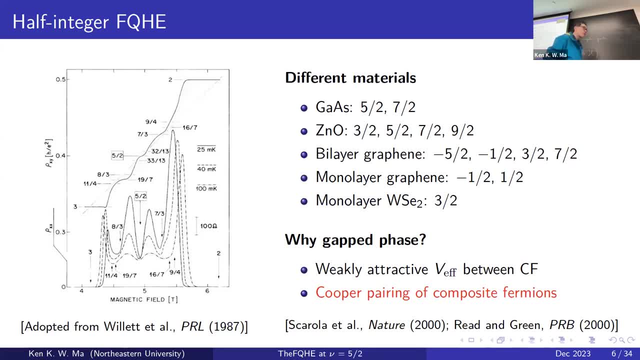 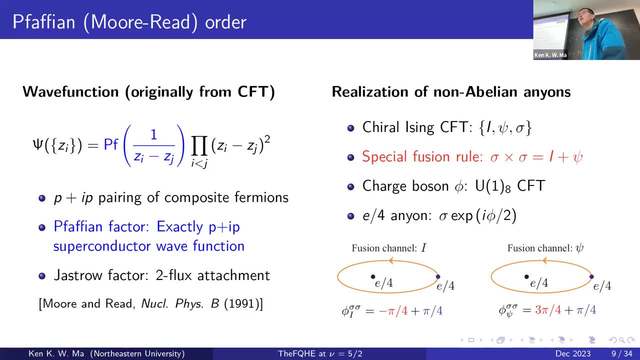 that this one is a quantum phosphate. Yeah, How can you move radials, You mean like experiment, or Ah, good questions, good questions. At this moment, I would say I don't know. Yeah, maybe, maybe you need to have some local, you need to generate some local potential. 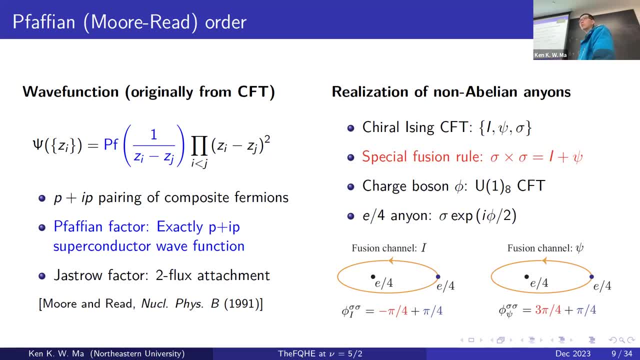 difference move. I don't know. Maybe you need to have some tip or what I don't know. Yeah, good questions. So you have some idea? Zhufeng? Yeah, but you also need to know how to move that composite right. And yeah, yeah. 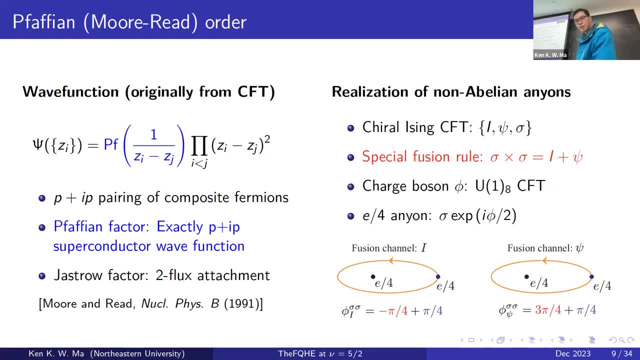 Yeah, I would say I don't have a good answer at this moment. Yeah, Yeah, If the anion is very hard on the electric thing one, then it's easier to move right. It's neutral anion that's probably harder. 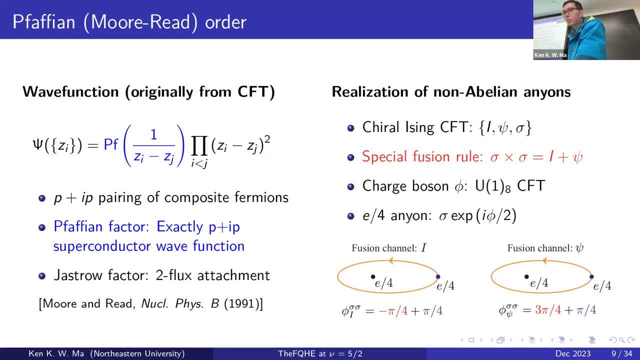 Neutral anion is harder. but that, Yes, yes, yes, But in Morbid state. let's say for Morbid state, or actually all the candidates, I mean all the topological orders that I've shown, the smallest charge is like u over 4,. 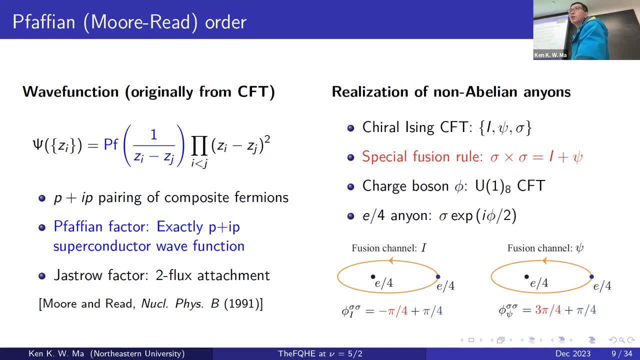 they are charged with particles. yes, That's the question, right, Yeah, why i'm thinking whether you can have, let's say, some local potential, and then you know, yeah, yeah. so because i'm talking about a fractional compost state at five half, and then we also know: 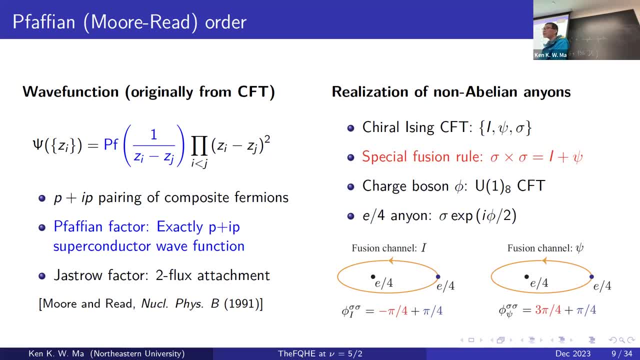 that a threshold compost state is like a topological state. that's why it's a low energy. defective physics should be described by topological order, but i i haven't told you which topological order, right, i only told you that probably it comes from superconducting. 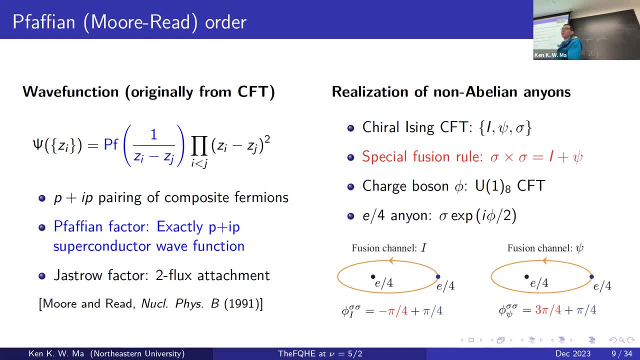 pairing between composite fermions. i even haven't told you actually how to pair up the composite fermions, okay. so let me take more historical woods, okay, and show you some different possibilities, and then, after showing you the different possibilities i want to share with you, is there any like a more uniform description between these possibilities? and then how can we? 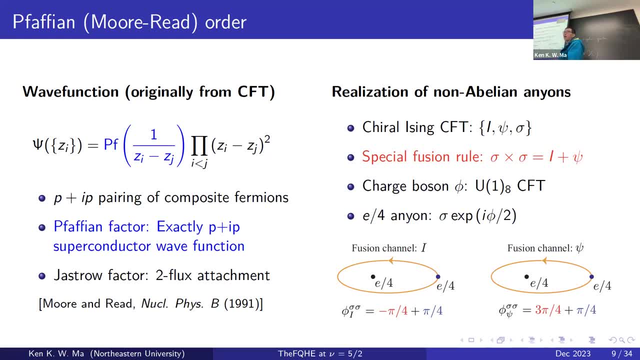 do different types of experiments to try to identify which one is really realized in the realistic sample, and i also will show you what we know about, let's say, from exact ionization, from numerics. okay, so one of the one of the famous possibilities for describing a fractional 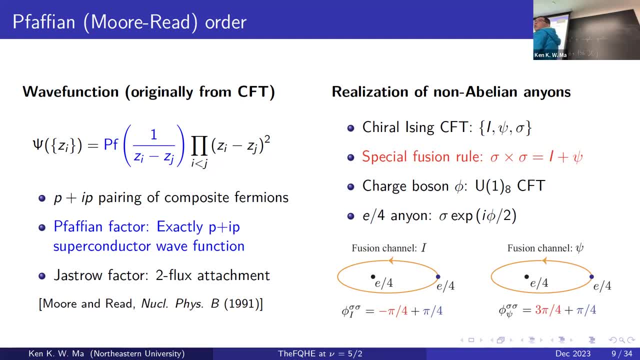 compost state at five half is, uh, so called the farfian state or the morris state, because it was first proposed by gradmore and then we. okay, that's why it's also called morris state. uh, here, what what this wave function actually describes is the half field and down level for 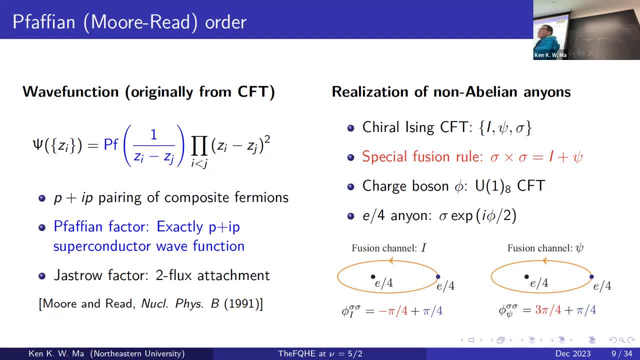 the first, first, first level, okay, i already neglect the two competitive field and our levels, okay, i only focus on that. uh, half field, uh, first, and rf, okay, and then this, uh, more risk state: uh, it has a great function in this form, okay, and then, if you, if you first, okay, you first at law this uh. 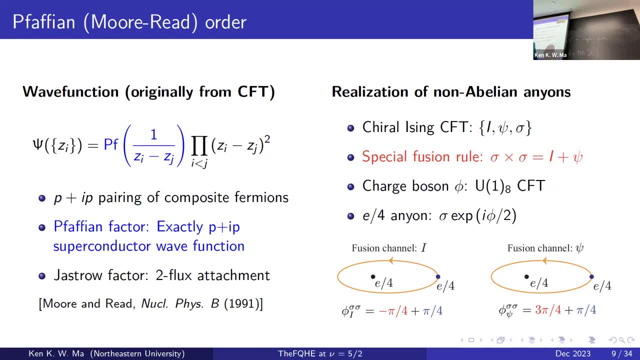 factor, factor. if you just focus on this, uh, gradual factor, it looks like very similar to the lafflin state. right in lafflin state, let's say fielding factor one third and the exponent is three, okay. that's why, in that case, when you exchange ci and cj, where ci is like the position of electrons, okay, and then if you exchange them, 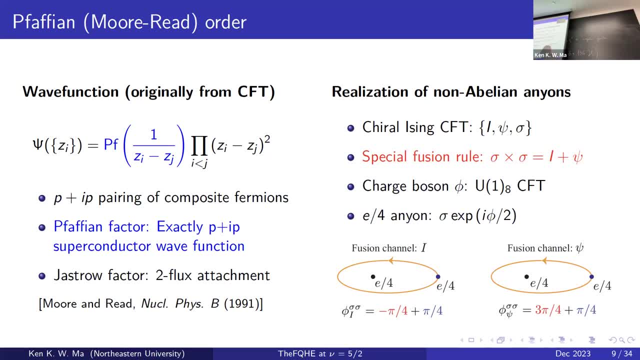 you get a minus sign, no problem at all. but here, if you don't include this, uh, factor, factor, okay. if you don't include it and then you exchange ci and cj, what you get is actually plus one. okay, then it will be problematic. okay, that gives you one of the handling items why i 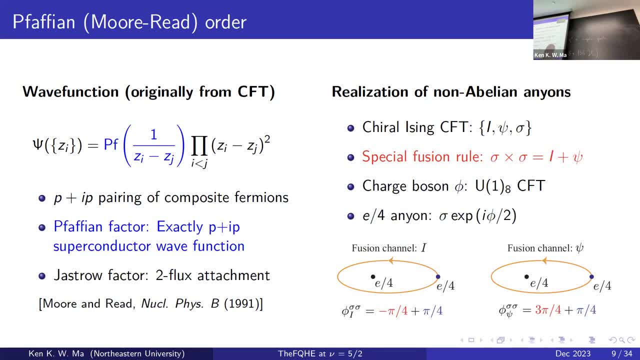 need to have something extra in front of this uh gradual factor. okay, the reason why i get two here is uh coming from the fielding factor. one half for my uh first level. okay, and then what does this uh factor factor actually means? is that, uh, this farbian uh vector is actually coming from a? 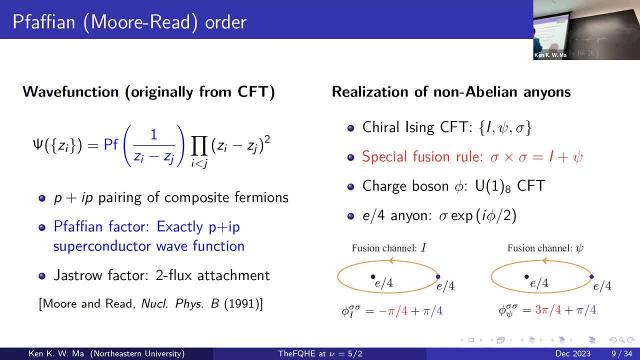 t plus ip, uh, parent between composite fermions. okay, because, uh, this gradual factor already implements a plus attachment. okay, that's why what i'm talking about is more like composite fermion. and then, um, uh, this farbian factor actually is a p plus ip. the dcs wave function you can treat as okay. okay, yeah, it really depends. i mean some literature we call. 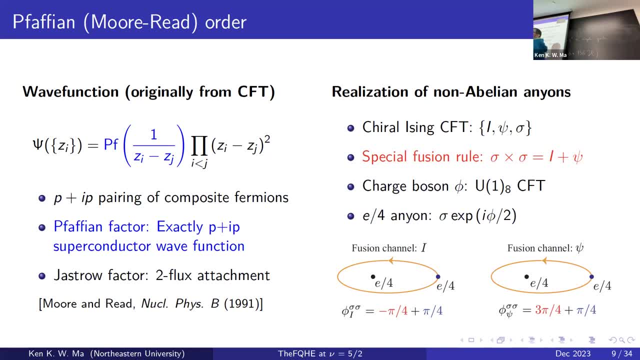 for this like minus ip, but yeah, it's just a convention. okay, i usually call p plus ip, okay, yeah, and then uh, this is uh from the perspective of wave function and then from the field theory perspective. then i want to understand what kind of anions that i may have right in in this topological state, and then 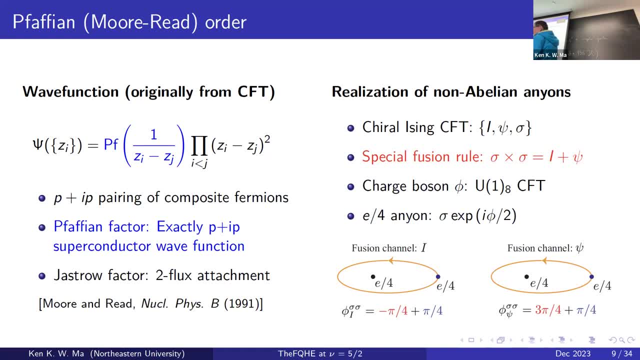 actually, this wave function was initially proposed by the conformal field theory construction. okay, the field. the conformal field theory is uh, is actually the ising cft, which have our three primary fields, that is, the identity, the uh by runner fermion, and then this field. okay. 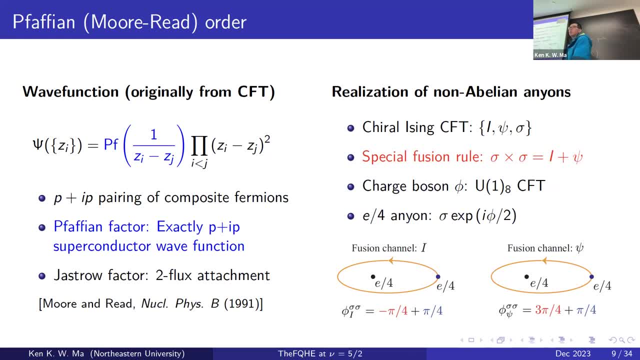 and then actually, i will say, all the interesting properties, let's say of the annuals in the more state, actually comes from this segment. okay, because this sigma, when you, when you fuse them, okay, you have two possible outcomes. okay, and these two possible outcomes basically tells you that 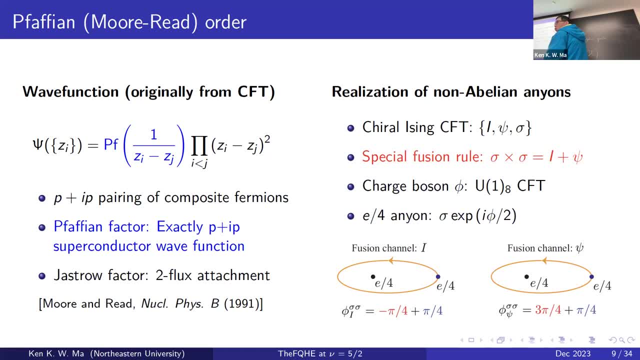 uh, any anyons uh with this sigma attached, then is uh non-abelian. basically, yeah, due to this uh interesting fusion group, okay, but we also know that, okay, uh, this is not good enough because, uh, here i don't have any charge here, but we know we really have a quantized electrical hall conductance, okay, that's why we must have. 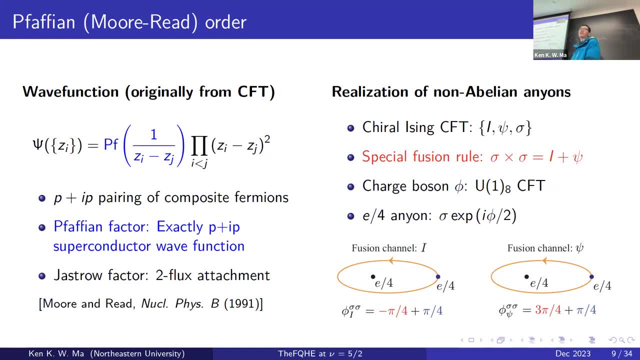 additional degree of freedom that gives you the correct electrical hall conductance and that that one actually comes from the chiral bosmo. okay, that chiral bosmo is just the, uh, simple, ab1 cft, okay, and then this age is just, uh, you, you calculate like the radius of quantification. 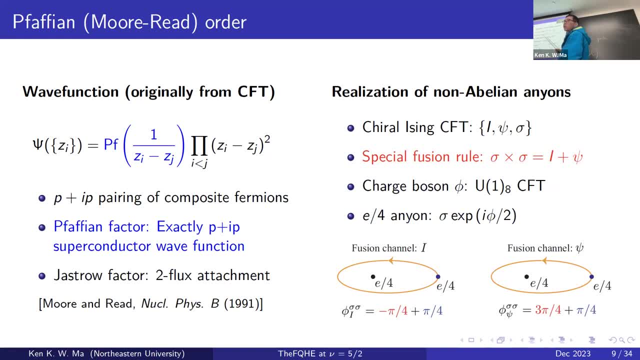 doesn't matter. the keep on is that now you actually need to have two kinds of degree of freedom. one is the usual u1 chiral bosmo, and then the non-abelian part actually come from the icing cft. is that okay? yeah, and then why it's so interesting? because, uh, now if i have a two, 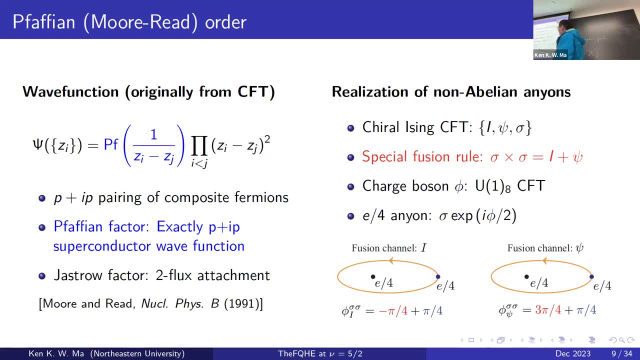 new before. let's say a proceed host, and then if you want to um move one of them around another, let's say in the full loop, then the phase factor that you will accumulate- I mean not you, but I mean the wave function- will accumulate. 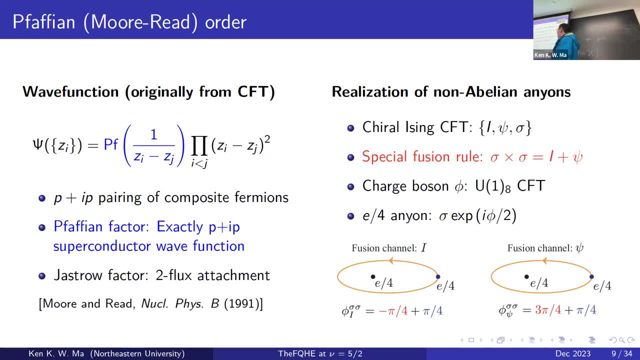 will depend on the fusion channel between these two quasi-particles. okay, Because sigma cross, sigma can be I and psi. okay, Let's say, if the fusion channel is identity, then it turns out the phase that you get is actually zero. okay, This red part actually. 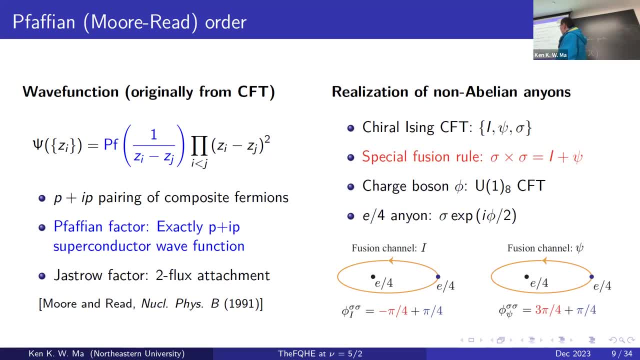 comes from the Ising-Cfd part and then this blue one actually comes from the U one. okay, The reason why I need to separate them is that I will, in the next slide, I will introduce you another possible candidate, that is, the anti-Fafian- the anti-Fafian. Then you will see the red part. 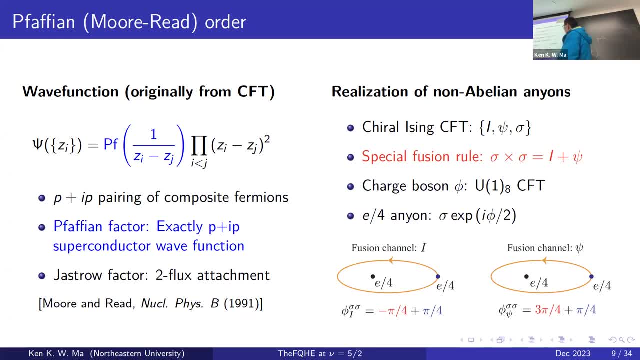 actually different from the Fafian. okay, And then let's say we go back to the Morse state. if the fusion channel between these two quasi-particles- let's say it's a fermion- then actually the phase factor, the wave function will accumulate, is actually different from this one. yeah, 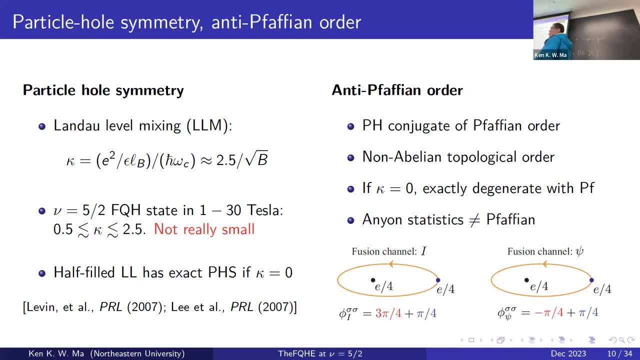 Okay now I just told you one of the possibilities, that is, the Morse state. and then let's say, in the half-field Landau level, let's say you don't have any Landau level mixing, which is defined as the ratio between the Coulomb interaction, and then 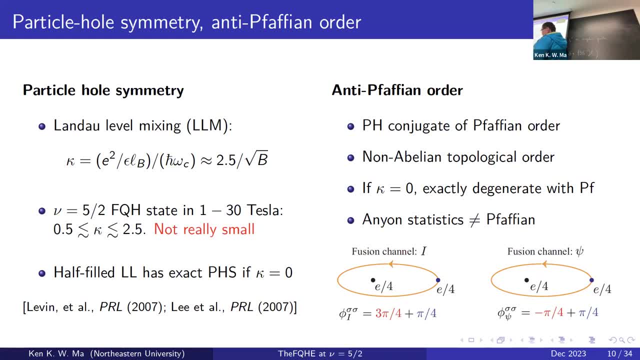 the cycle-joint gap. okay, Suppose that Landau level mixing parameter is exactly zero. okay, Then for the depth half-field Landau level you have an exact particle hole symmetry. You just imagine, let's say I have a half cup of water. you may say it's like 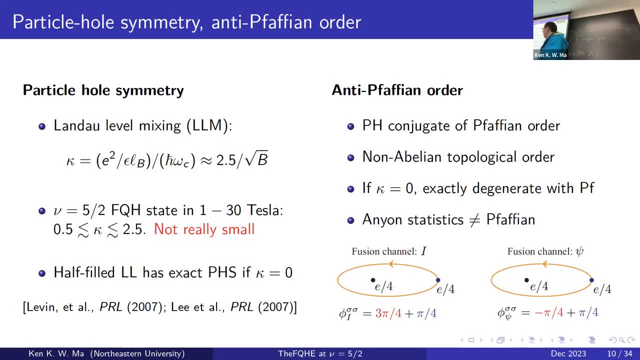 half-field or half-empty. okay, The same story here. So that's why, if we really consider this extreme case- let's say the Landau mixing parameter is strictly zero- then particle hole symmetry is an exact symmetry. If it appears the case, then the 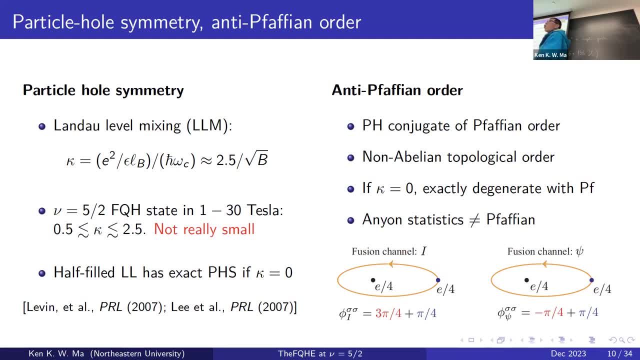 Morse state is a possible candidate. It also means that this particle hole conjugate should be another promising or is another possible candidate. okay, And this motivates people. let's say, in 2007, they considered another possibility called the anti-Farfian. 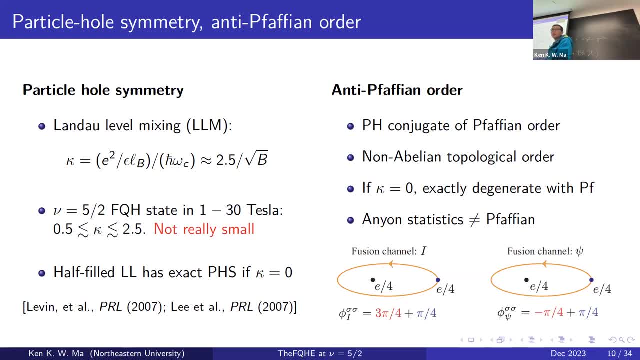 which is the particle hole conjugate of the Farfian state. yeah, But I also want to tell you that actually, what is the actual range of the Landau level mixing parameter? let's say experiment, okay, In experiment, actually, that Kappa is somewhere in between 0.5 and 2.5, okay. 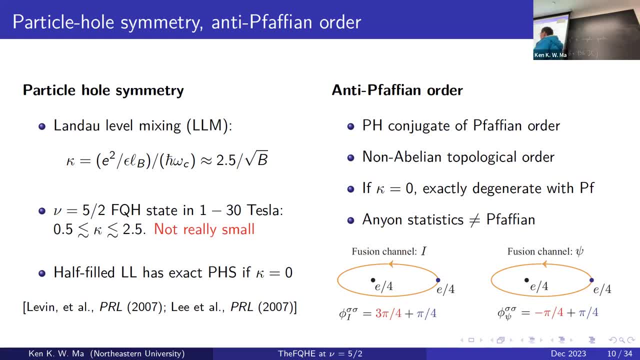 That's why it's not that small in this sense. okay, But we can still treat this one, this anti-Farfian state or anti-Farfian order, as a possible candidate. okay, So which one is favorable, I cannot tell you. okay, It's God chooses it or the nature chooses it, okay. 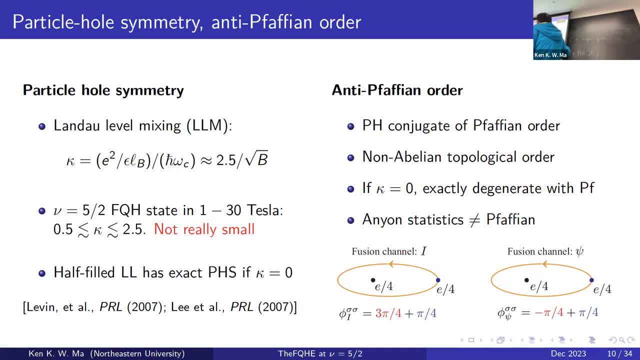 Okay, And then I also told you that when I consider anti-Farfian and then if I consider the U over 4 quasi-particles or quasi-holes when you move one of them around another, I told you that actually the U1 part, the phase, the contribution to the phase vector, to the wave, 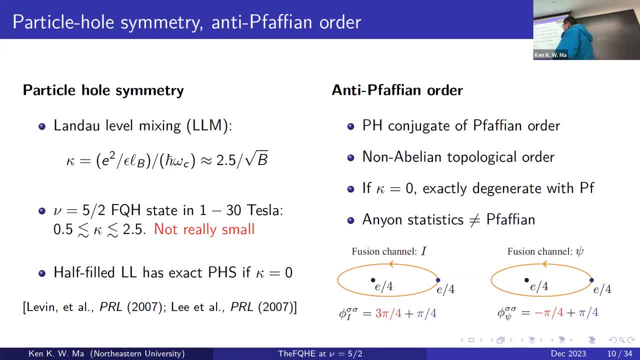 function is exactly the same as in the Farfian state, But the phase vector coming from the non-Eubedian part actually is different from the Farfian. okay, So that's why this is another, another way or another evidence that this anti-Farfian order is actually not the same as the. 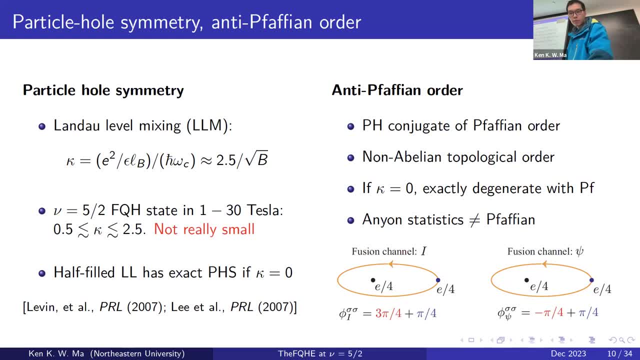 Farfian one. Is it possible that the sample of Farfian kite depends on Poroson's from the temple other than Mmm? yes, yes, yes, yes, yes, yes, exactly Yes, it's possible. Yeah, it's possible, yes. 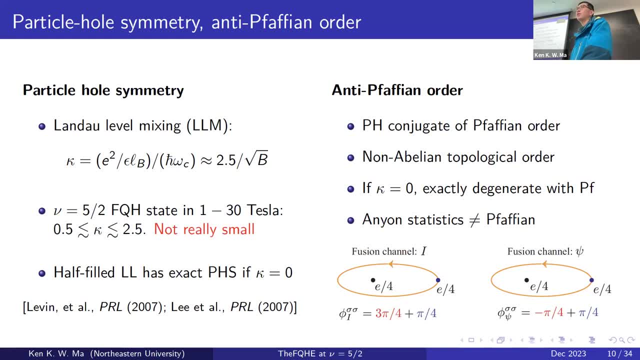 possible, yes, and actually actually both landau level mixing and disorder. i think both of them are important if you really let's say, when it comes down, which one is more like an energetic, pretty favorable. yes, you're right, yeah, you can do so. yes, and i will also tell you probably a more systematic way to do it. 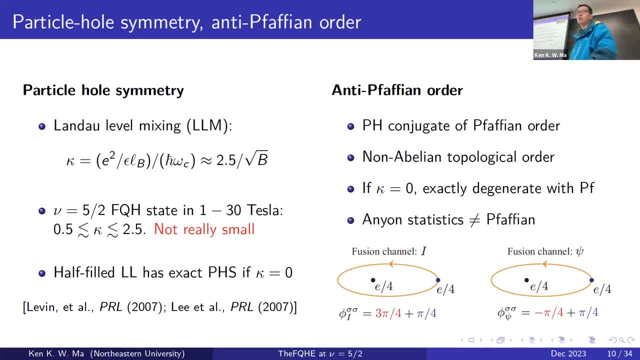 yeah, maybe i didn't really put down mathematics, but i will try to introduce you, let's say, formula some, and then actually, if you go to paper you can find more systematic way to do it. okay, now i tell you like, uh, fafian, antifafian, and i need to introduce you the third. 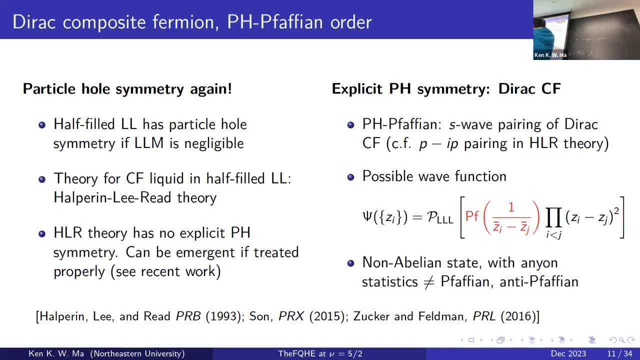 fabian type of state. okay, which is called ph- fabian, and ph5 instead of particle whole- fabian. okay, so here i want to uh make a statement like, actually, the ph5 does not require particle whole symmetry to stabilize it. okay, this one is important. okay, this one is important, okay, and then why? why was this, uh, ph5? 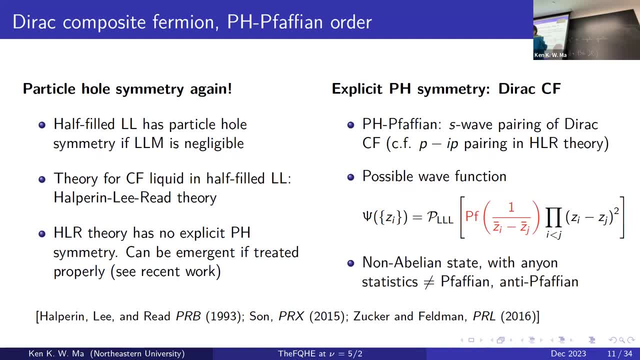 being introduced is that people reconsider the questions of half field and area level. okay, as i said, if we don't have a demand level, mixing the half field and the level have has an acceptable symmetry. but, uh, but, but if you look at the famous uh hyden d rich theory, describing the cf liquid and how the extracts. a high d risk theory of the cf liquid in half field and the half level have as an accept, a pf symmetry, but uh, but if you look at the famous high d risk theory describing your cf liquid in half field and non-d, 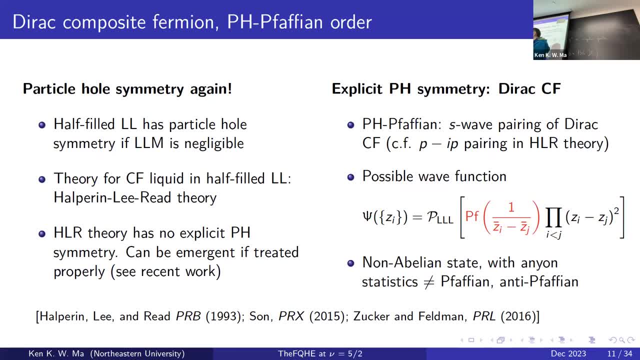 Landa level. what they are doing is that they attach a magnetic flux pointer to an electron. okay, That's why they don't have an explicit particle symmetry in the construction. okay, So that's why Damson, in 2015,, tried to reformulate, let's say, or introduce another. 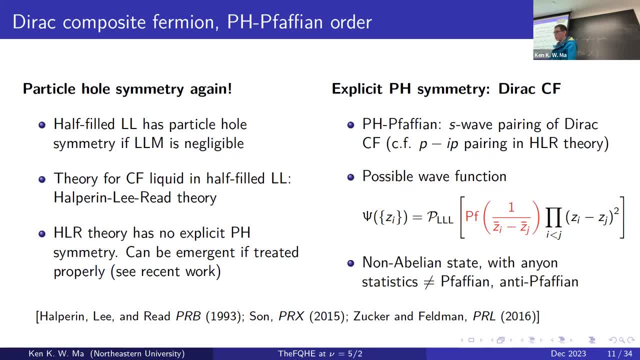 theory to see whether one can incorporate that particle symmetry explicitly. okay, That's why it leads to the theory called Dirac composite fermions. okay, And then. ah, after introducing this Dirac composite fermion, then the lecture question, of course. 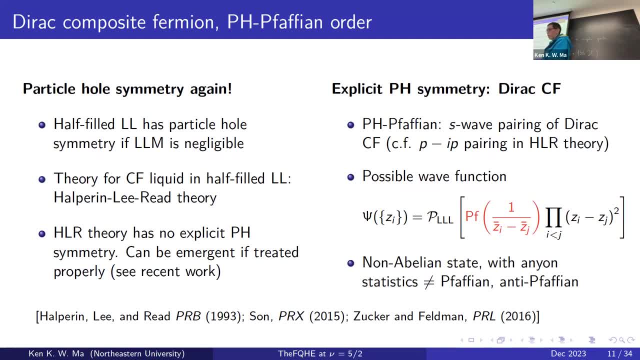 is also asked what kind of pairing stage or pairing flexible, compulsive state that one can get. okay, And it turns out if you pair them to the lowest angular momentum channel, that is the S-way pairing, what you get is actually lock the farfion, lock the anti-farfion. 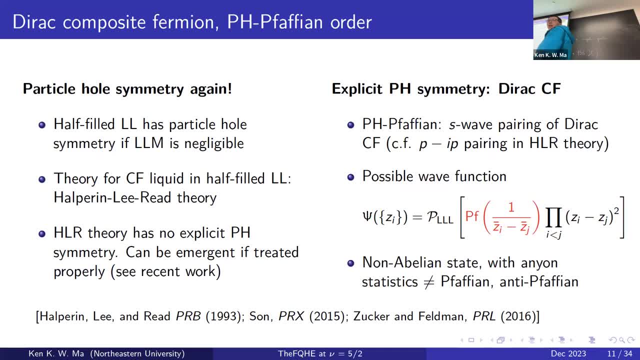 What you get is actually something called a pH barrier, And this is basically historically why people also consider this pH barrier. And then, if you ask me to give you, let's say, wave function, because let's say you do a numerical simulation, I tell you all the field theory description. 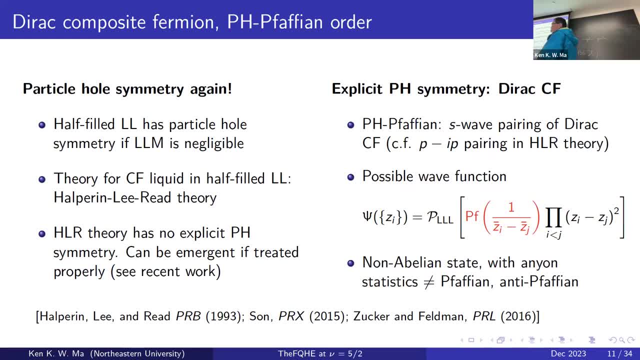 basically, I basically tell you nothing. What you really do is, let's say, after accept ionization, you want to do some overlap between your result. and then let's say, a model wave function. That's why I need to tell you a possible wave function. And then for this, pH Fafn. 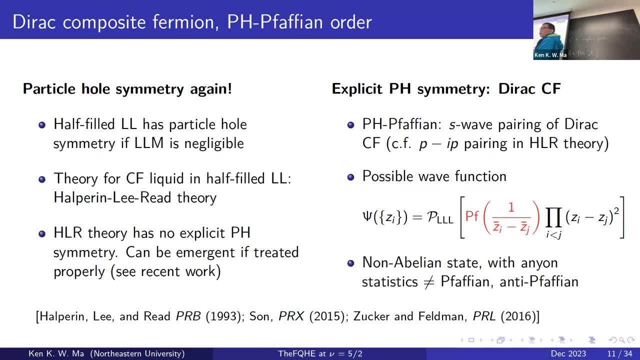 if you use the HLR theory description or the ordinary composite fermion theory, then it corresponds to P minus IP, para actually. But for the Fafn that I told you like two slides before, it's a P plus IP. So the difference actually is inside the Fafn. 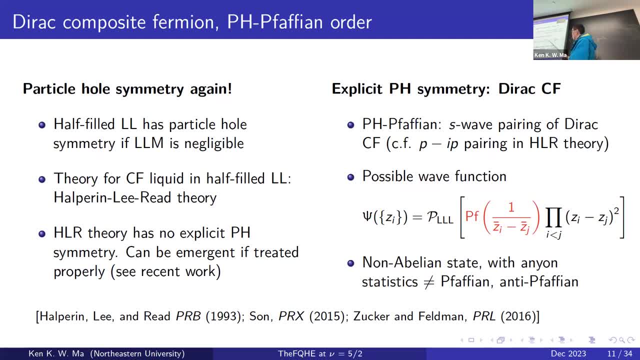 So for the Fafn state, this Fafn factor is like one over Ci minus Cj, which is a holomorphic. That's why I describe a wave function in the lowest Landau level, But here it's like one over Ci bar minus Cj bar, where bar basically means complex conjugation. That's why this part. 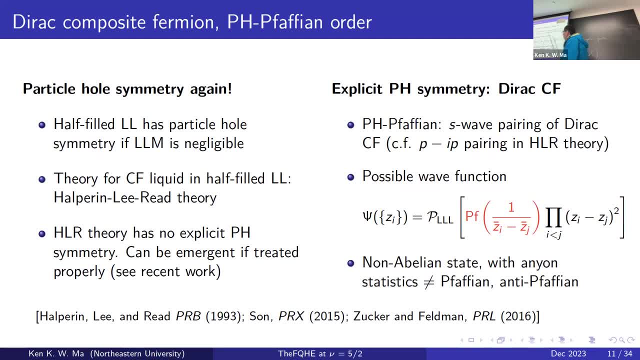 is anti-holomorphic. That's why we load this wave function before. this projection is actually not describing any wave function in a single Landau level or in the lowest Landau level. That's why you need to do so. So you need to do the lowest Landau level projection here, And this is one of the 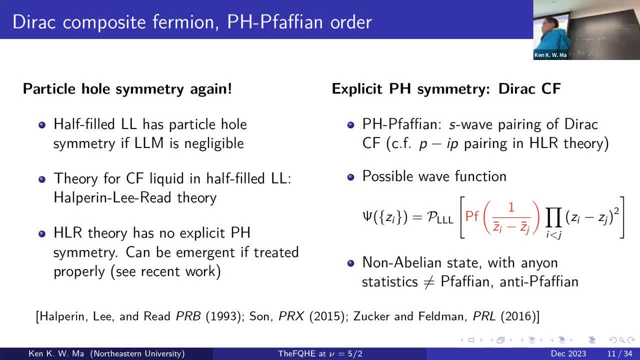 possible wave functions for this pH Fafn And then similar to Fafn and anti-Fafn. this pH Fafn order is also non-Appelian, But here I don't have space, And then I think I can just tell you that the annual statistics is actually different from both. 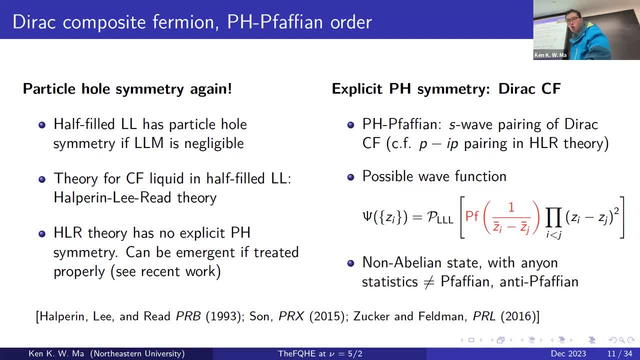 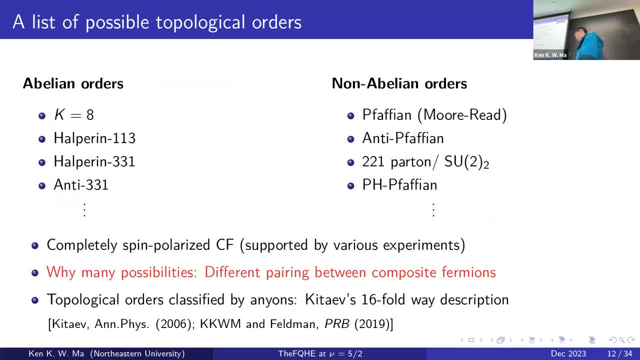 Fafn and anti-Fafn. So these are the three Fafn states We usually focus on. Well, is it just the n of the possibilities? Actually, no, I just tell you about Fafn, anti-Fafn and pH Fafn. So actually, let's say, if you look at the historical development, 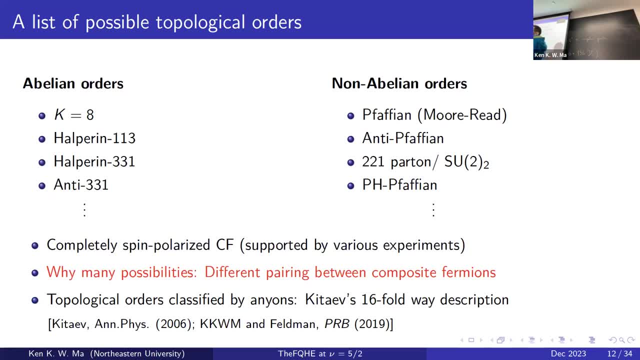 actually you also have a billion orders for the possibilities. Let's say K equals to 8, it's hyphen 51, it's a particle conjugate or hyphen 1 minus 3.. All these four are actually describing a fractional composite state. 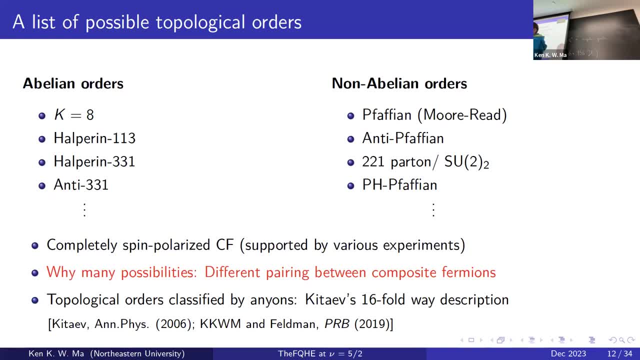 It may describe a fractional composite state as a fielding factor, one-half or five-half. But even in the non-Appelian sector this does not only end at Fafn, anti-Fafn or pH Fafn. So you may ask me. so, given that there are so many possibilities, can you suggest, let's say, 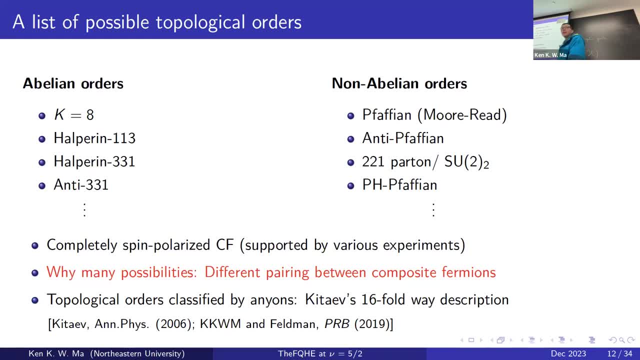 a more uniform theoretical description among them. And then, if you can find that description, can you tell me what is the, let's say, more universal or more common feature, let's say, for the bulk physics and also the edge physics? And these questions actually motivate us to look at. 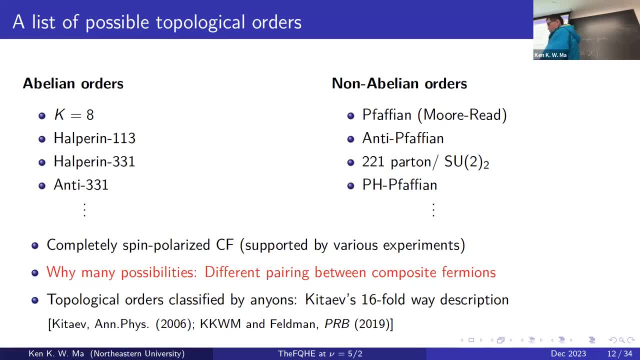 this more uniform description. And then we eventually find out that actually if you assume the composite fermions are completely spin polarized and then if you assume the five-half state actually comes from a chiral BCS pairing, then if you look at the Hamiltonian you see that actually that Hamiltonian is exactly the same. 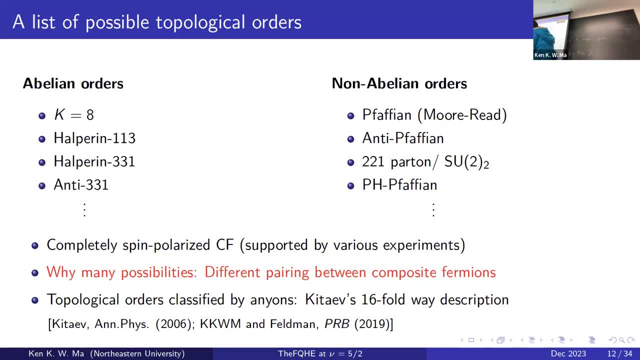 as what Kepp has studied. That's why it motivates us whether those these possibilities also satisfy the something called 16-fold wave description, And then I will tell you what it means. okay, and then more information you can find in this paper. 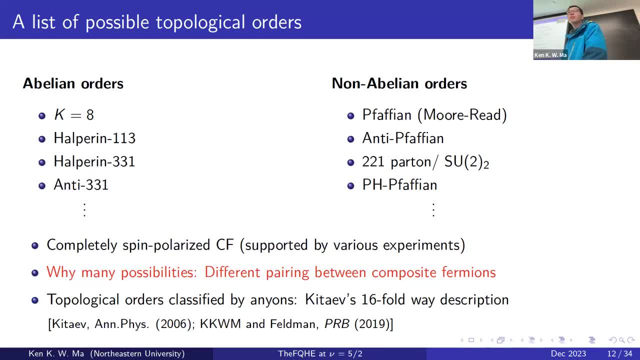 This 16-fold wave doesn't mean you can find a composite diagram picture. It doesn't require. it doesn't require. But it's like if you so the original, the original one is actually in the Kepp model right. It's like has second and then you have different spin. 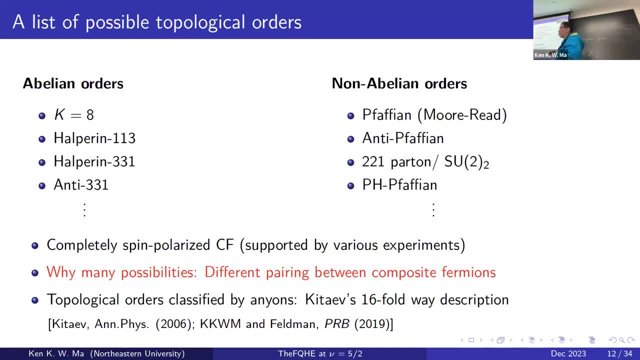 interaction, different spin interaction. Actually, in this original proposal it's not composite fermions thing, right, But if you believe that composite fermions, that they are completely improvised, and then if you want to describe what are the possibilities of those chiral pairing state, 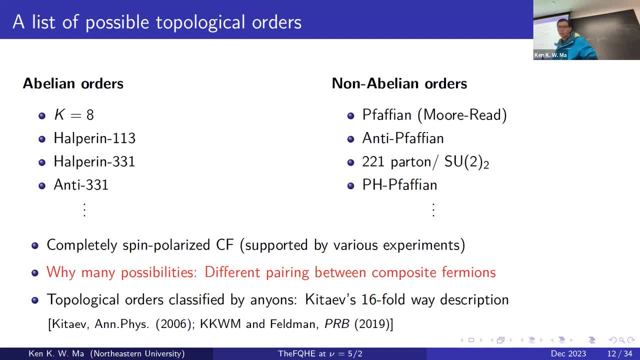 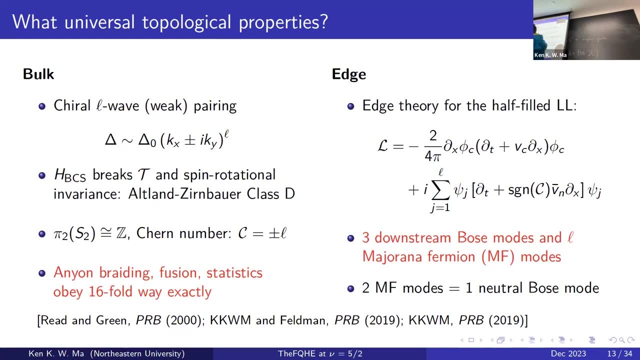 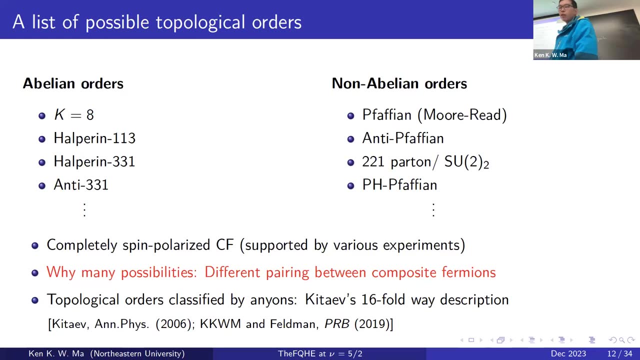 then it turns out the structure is the same. Yeah, so so let's say, let's say I look at both different possibilities, as that's right. I mean, if you, if you assume, if you assume the, if you assume the 5-hop state is from BCS pairing. 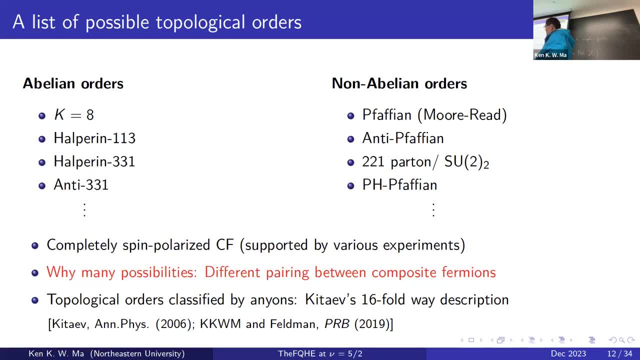 but at the same time it's chiral L-wave pairing and then you write down that BCS hematomian and then you express it the same way. Yeah, I can't. I can't remember the exact details, but there is some way that you can compare it. 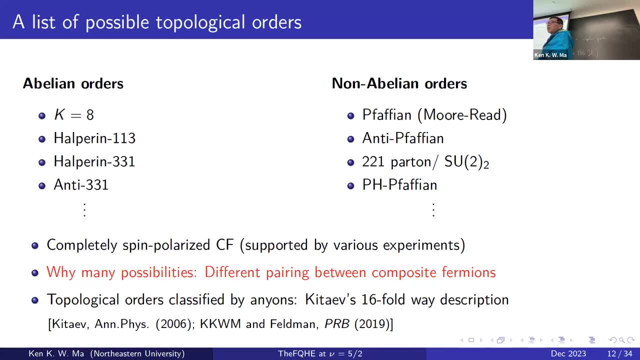 with the, with the model that Kepp constructed, and then this: I think the mathematics is, I mean the mathematical structure is the same, Yeah, yeah. So this can I say? can I say it's out of order? No, no, just no. I mean it's like there are some assumptions there, It's just like class, class only. 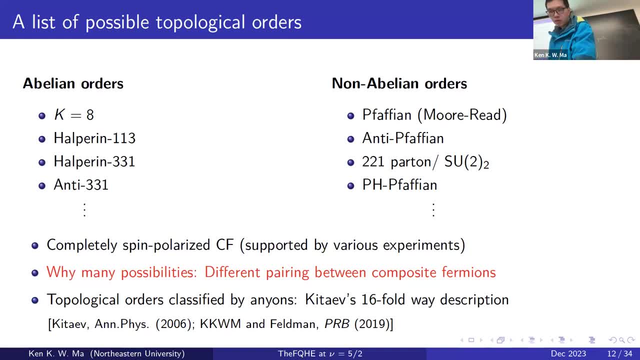 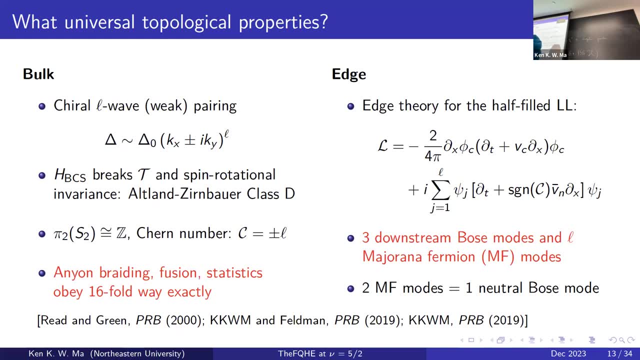 Yeah, okay. so so let's say, let's say, I only focus on this chiral L-wave pairing. What does it mean? is that the superconducting order parameter takes this form? okay, and then, and then, if we really study, let's say: because we know, we know from previous. 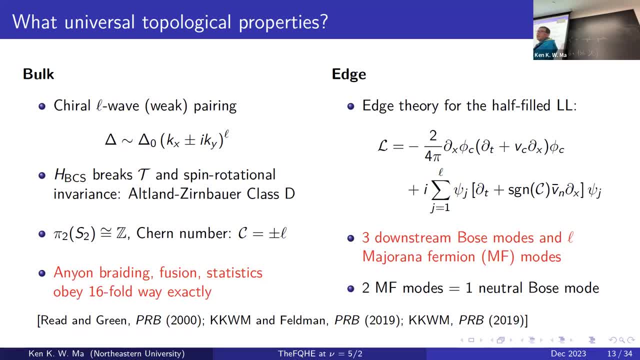 literally what are the annual statistics? let's say for Fafian, NF-Fafian. we also know what are the statistics. let's say for high-frequency 51 states. okay, and then it turns out the neutral sector. okay, as I said, you always have a U1 set up for the charged one. okay. but if you only focus, 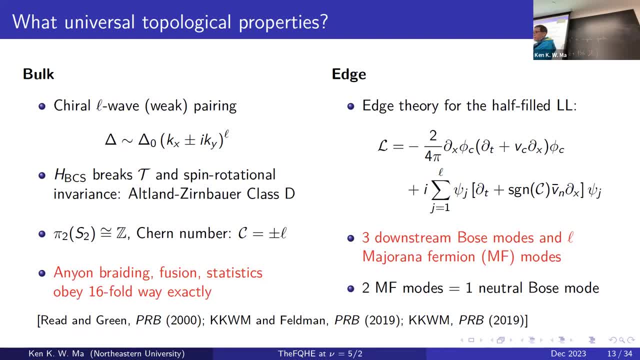 on that neutral sector. it turns out that braiding statistics, the fusion rules and the types of annual actually all of them agree with the 16-point wave. That's that motivates us to see whether there is this 16-point wave also possible in other possibilities. okay, 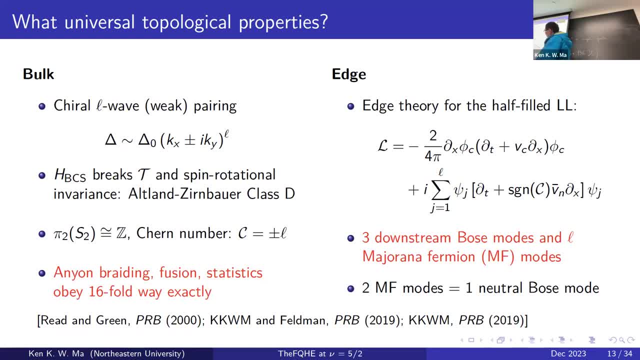 And then this one is more like: what is the, what are some of the common features, let's say for the bulk? then the next question to ask is: what? what are the common features, or more universal features for the edge right and then actually for the edge, as I said, you always have a U1. 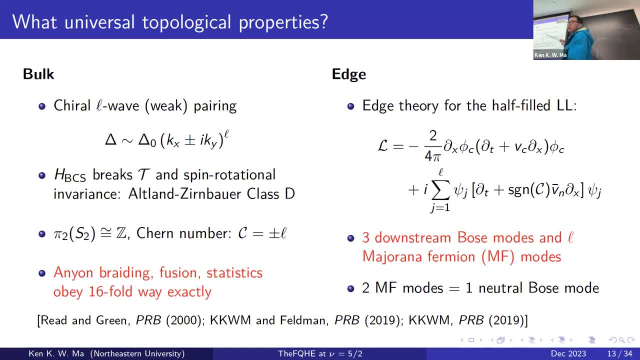 that chiral bounce pattern that turns into a new weak current consensus. Yavore, might you talk a little more about the original measurement and if there are any other management elements to your analysis that gives you the correct electrical hall conductance? 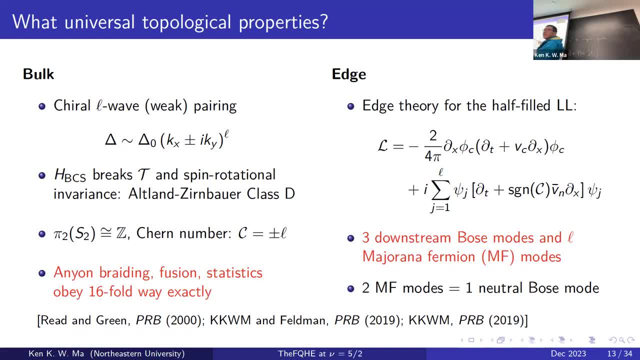 And then, depending on which parent channel you select, okay, for the possibility, it generates a different number of Majorana fermions on the edge. okay, And then these Majorana fermions, they may actually travel in the same direction as the Bose mode. 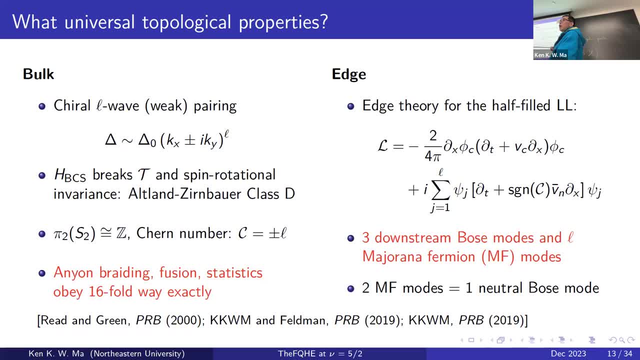 or they can move in the opposite directions. okay, So let's say, for the five-in state, I will probably show you in the next slide the Bose mode and the Majorana fermion modes. they are actually moving in the same direction. 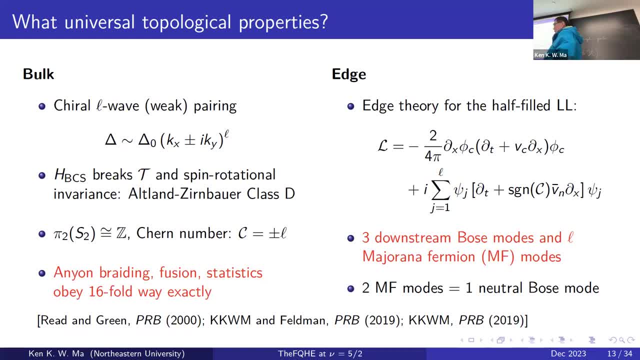 Another feature that I will use is like for two Majorana fermions moving in the same direction, I can combine it to a usual fermion and then I can Bose on it, okay. That's why, for two Majorana fermion modes in the same direction, 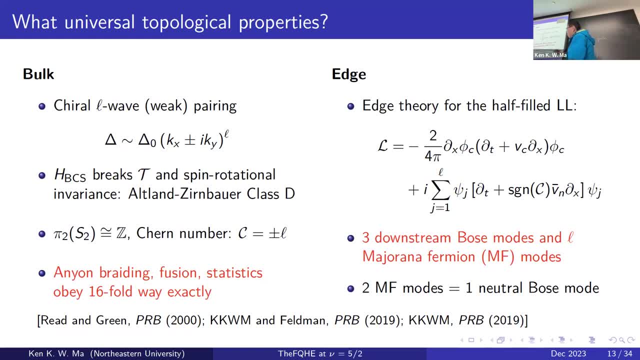 you can just replace it to one neutral Bose mode. That's a Majorana fermion here it's neutral, okay, That's why, when you combine them to a corresponding Bose mode, that Bose mode is neutral. Yeah, so what I'm trying to say here is that 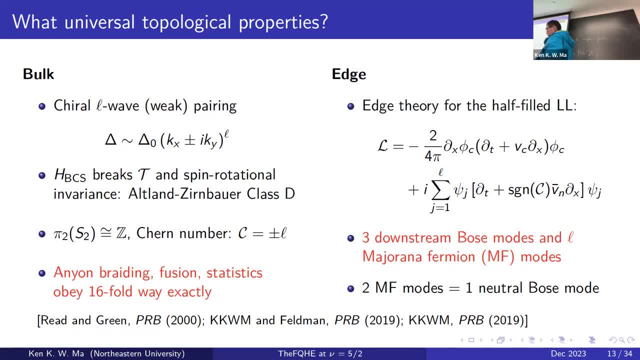 the more universal feature is that for all the- I mean for the possibilities that I've shown you in the last slide. you may understand it is like coming from the chiral airway, pairing between composite fermions and then for the bulk, yeah, the anion types. 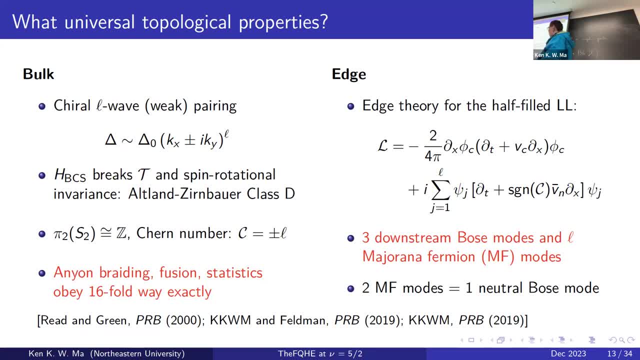 the braiding rules, fusion rules, the statistics- you can predict them from the 16-fold wave results- and then for the edge, the common feature is that you must have like a single charge mode, let's say moving downstream, and then depending on which channel you have. 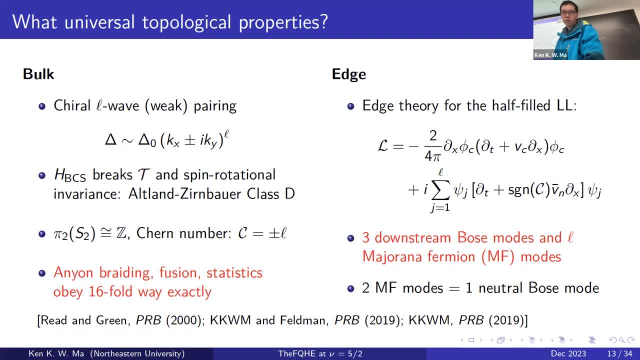 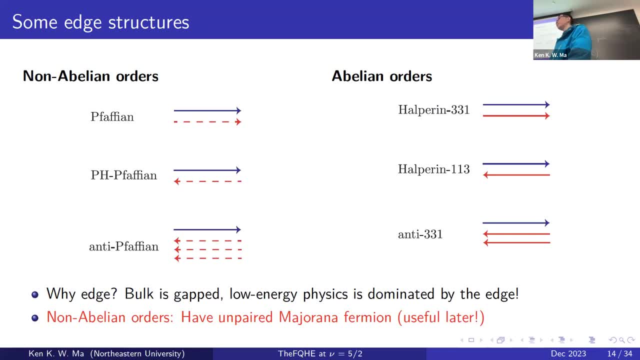 then you have a different number of Majoranas, okay, Okay, So is there an integrated way to understand the number 16?? So maybe, Zhu Fen, you can answer that, or more mathematical questions. Yes, And then it's one of the other key of Никola Varela's. 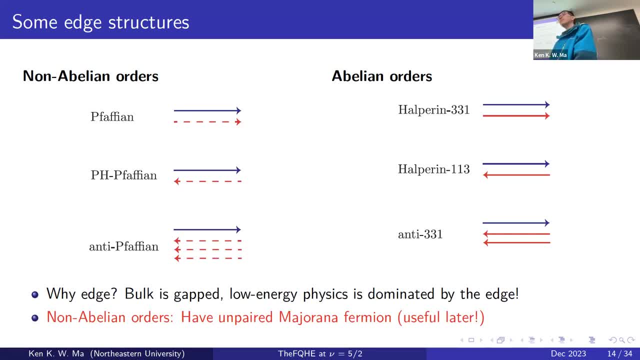 method of inverting the field theory On the other hand, the one. there's an inverting field theory and so on. So you don't have the in this inverting theory, the way to determine the. yeah, we can also share this too. yeah, and also one more. yeah and also one. sorry. 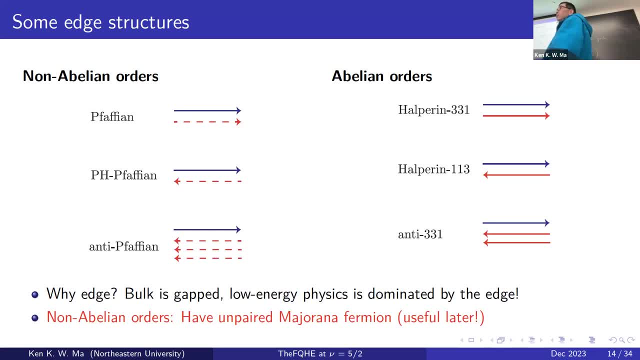 now depends on what kind of quasi particles you are talking about. yeah, let's say for five, half state, and then for those possibilities that i showed you, the smallest charge of quasi particles that you can have is e over four or minus e over four, and for these kind of things they are non-abelian because, uh, that that neutral sector i mean not. 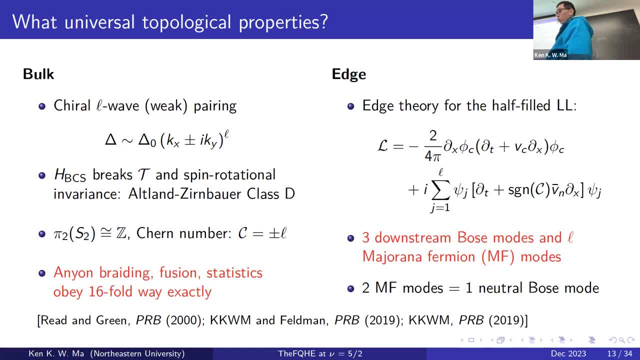 neutral sector. but you can, because in quantum physics, when you want to, let's say, create a quasi particle, what you have is actually a conformal field theory operators. okay, so the charge part is described by vertex operator, but you also have this ising cft, that is isi or sigma. 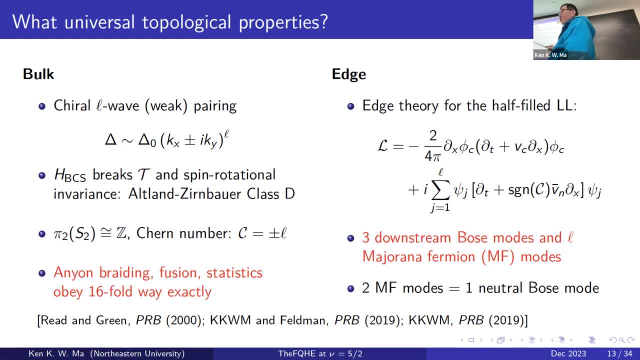 but for e over four, that ising cft part, is that sigma. that's why that u over four quasi particles are non-abelian. but if you talk about, let's say, quasi particle with charge u over two, then that charge u over two anions are actually abelian. so it really depends. you may also think of like: 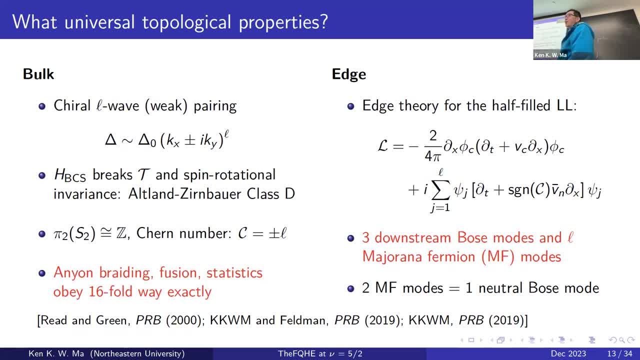 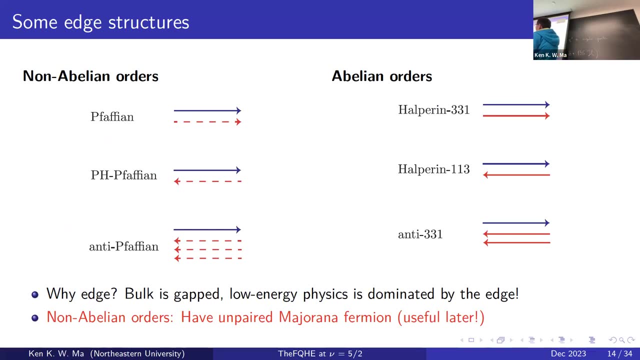 electron. electron you can also treat as like one of the anions, right, but but electron must be abelian. yeah, so it really depends on what kind of quasi particles you're talking about. yeah, so, as i promised. uh, so if you look at our different probabilities, their edge structures, 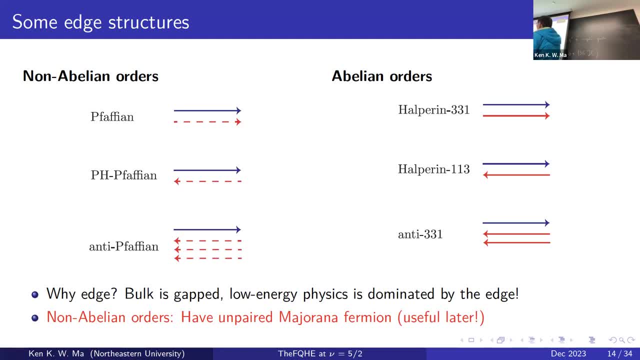 are different depending on which apparent channel you want to have, let's say, for the. this is, uh, the edge structure. the reason why i show you this? because it will be useful when i discuss our experiment. okay, and then here i just show you actually the s structure for that, uh. 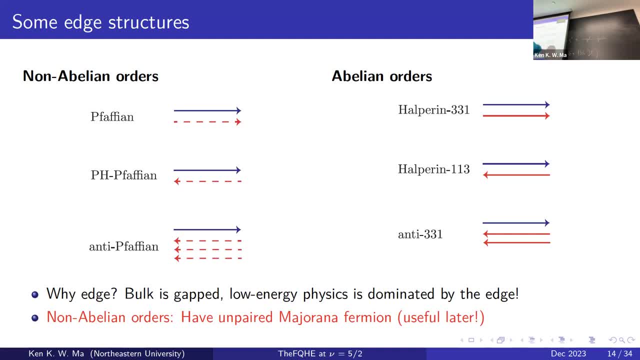 half-structure, and then here i just show you actually the s structure for that half-structure. and then here i just show you actually the s structure for that half-structure and down level: okay, there are actually additional two full charge modes. okay, uh, coming from that two completely. 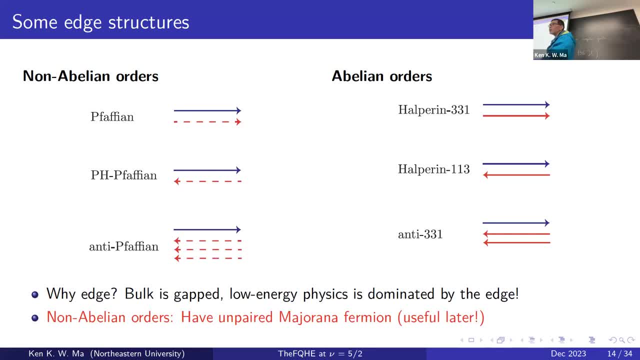 few and our levels okay. but i just don't care about that. okay, i just think about that half billion level. that's why for the fabian i only have uh, one, uh, both mode and one mirana. they move in the same direction. but for ph-fabian i also have one bosmo, one marana, but loudon by running. 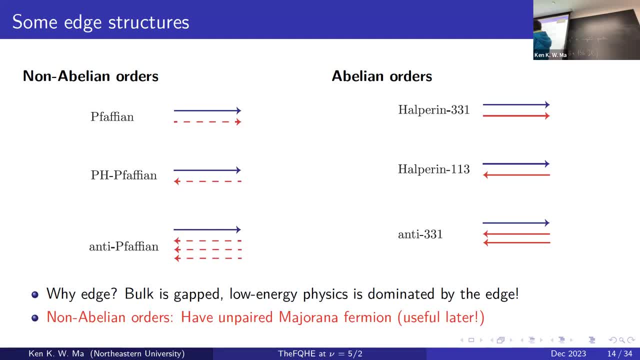 or upstream. upstream means that, uh, it is uh in the opposite direction as the uh charge point. yeah, so if you go back anti-fabian here, actually i jump steps okay. uh, actually it's like a one, one charge mode actually going to the right, uh, there is an other charge mode going to the left, and then 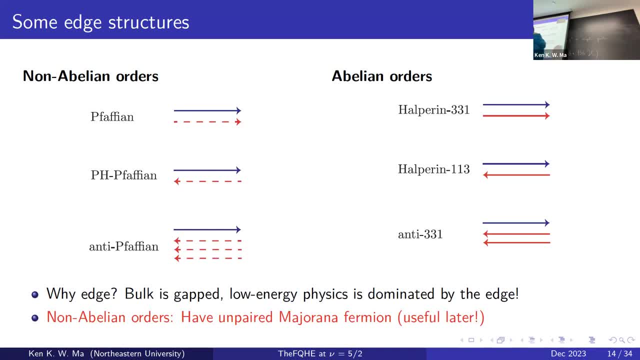 the marijuana going to the left. but you know, in relics, in realistic sample, you also have disorder and then this disorder couple, that two kind of propagating edge, depending on, uh, which fixed point you are talking about, let's say, in the disorder dominated fixed points, then a better description is like you just have one single. 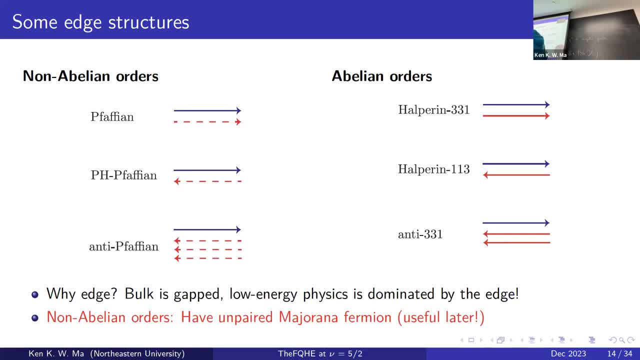 charge mode: uh, going downstream, and then that the remaining one will become neutral, and then you can realize three in my right, moving to the left. so that's that, that's basically. i'll show you some examples of the edge, uh, the action of the edge that i showed you in the previous slide. 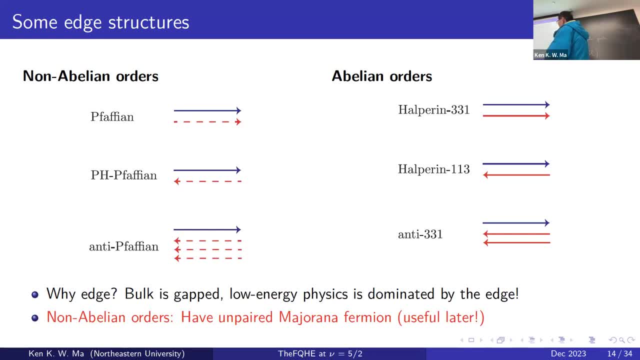 but for a brilliant order as well. it's the biggest difference that there there is low unpaired marijuana here. so let's say, for the high point 51, then i only have one uh charge mode and one uh one neutral mode. okay, but this neutral mode actually is a whole song, okay. that's why i don't 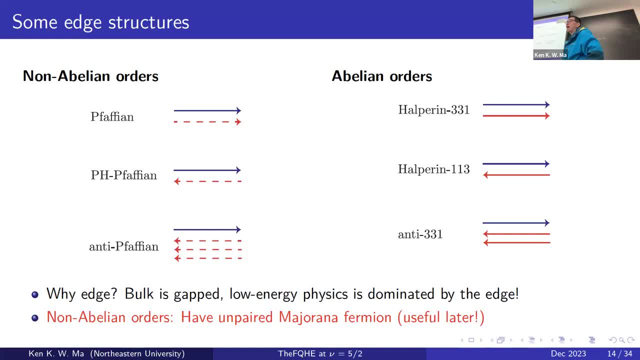 have any unpaired my runner here- and this one is very important- when i discuss a thermal hall conductance experiment, okay, a billion states have also existed in monolayer system. uh, it depends, right. i mean, let's say, if you talk about, uh, fractional quantum state of fielding factor one half, okay, uh, let's say, in monolayer system we usually don't see any. 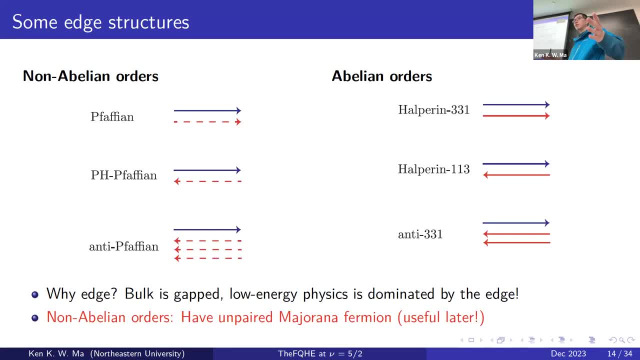 gap state. but let's say, if you have a very wide gallium s and i quantum, well, actually you see fractional composite of one half, and then there are some proposals trying to, you know, a little bit debate whether the high point 51 is favorable, or the five is favorable, or actually long of the 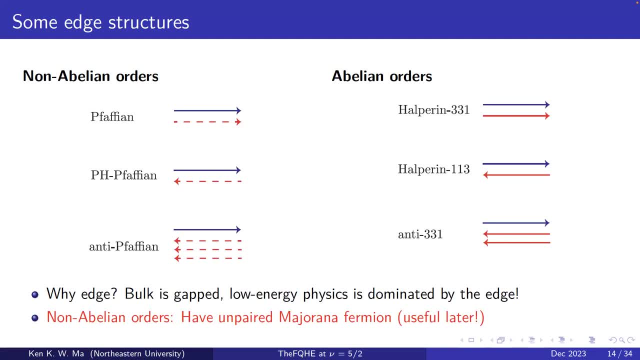 favorable and then it's: uh, it's like from numerical simulation it really depends on the competition between interlayer tunneling and the interlayer interaction. so it's possible, it's possible that this hybrid 51 state can be realized. that's seen by the assistant. yes, 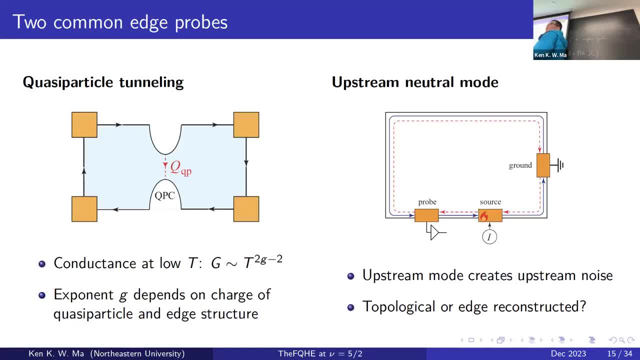 okay, so i show you different uh structures, but all are mathematics or a theory. okay, but we do physics. okay, so we know physics is more like uh can only be checked from experiments. right, and then what is the nature of the materials? the only way that you can answer is do an experiment. okay, so what kind of experiment that uh one usually do to distinguish? 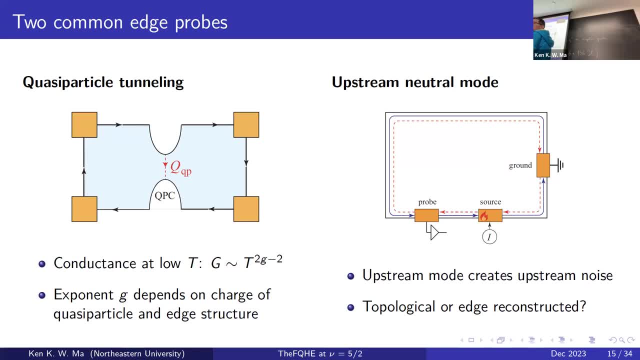 uh, different topological orders. right here i just show you two of them, okay. uh, later i will show you the third one. okay, but just focus on these two first. the first one is the so-called quasi-particle tunneling. it's like. this one is my uh quantum for sample. 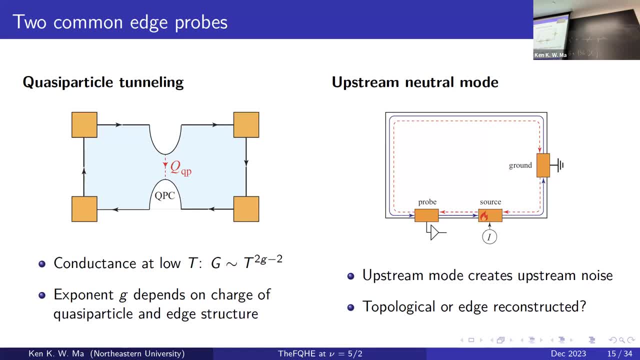 and then i make a level construction here which is called a quantum point contact here, and then, uh, at this quantum point contact quasi-particle can tunnel uh from one edge to another edge. okay, and then it will generate a uh tunneling current. okay, and then at low temperature, okay, if you. 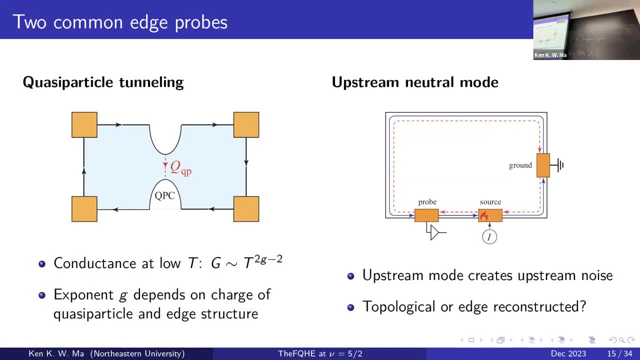 calculate the, or you measure tunneling conductance, then actually scale with the temperature in this this way: okay, 2g minus two, and then in the experiment you actually measure two things at the same time. you want to measure this: the charge of your positive particle participating in this tunneling, and also what is sorry, and also what is the tunneling exponent g. 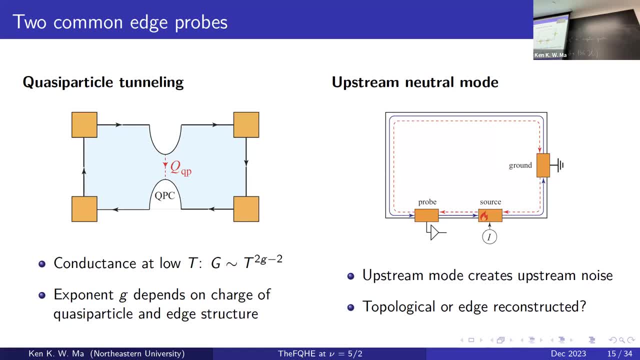 the. the reason why people measure this um underlying exponent g is that this exponent g actually depends on the charge of positive particles and also the edge structure. okay, let's say. okay, let's say, let's say if, if this quasi-particle is e over 4, then a general argument is that if your edge structure has more, 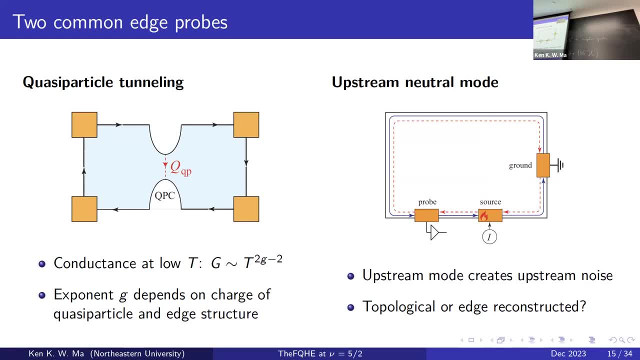 edge more okay. let's say, if i compare fathom and anti-fathom, okay and the fusion, i have like one charge today, pre-mark runners before 5 characters, 1 charge mode and one block. So in general, if the edge has more energy modes, then this way of g will be larger. if, if in both cases, you're over four is. 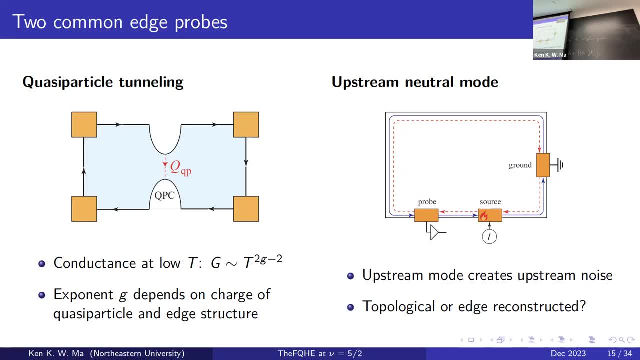 participating in the tunnel. okay, But there is some subtlety because you also have, like U over two, quasi-particle And in some cases actually the quasi-particle participate. I mean that quasi-particle tunneling here probably is not U over four, maybe U over two. 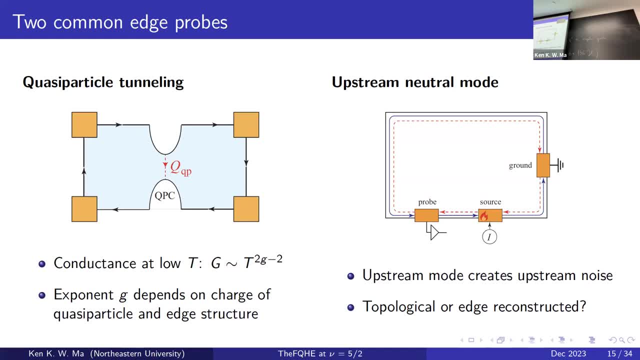 then the story will change and then become more complicated, But there is still some hope for you to use this one and then to see actually what edge structure is more promising. And then other experiment that people do is something called the upstream neutral mode. 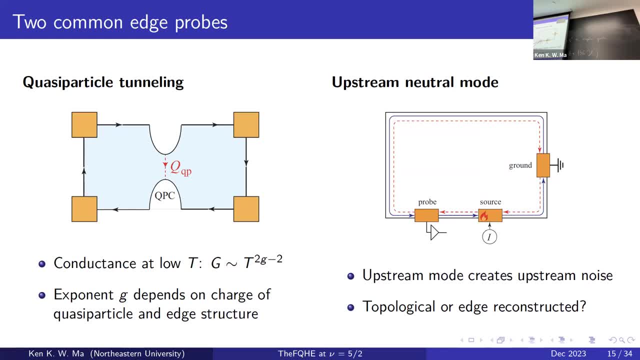 What they are doing is like I have a source and then I have a probe, and then I have a amplifier. here. Let's say, this blue line is the downstream charge mode, okay, And then from experiment people know that there is a hotspot. 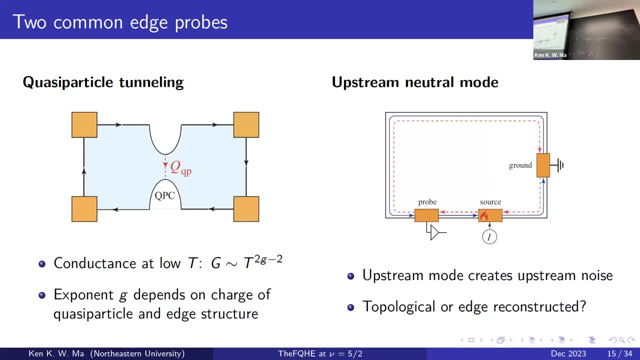 at the back of source. Let's say, if your edge structure have some upstream mode, then this upstream mode will be hit up by this hot source and then it will propagate. But this upstream mode, let's say it's neutral, then it doesn't carry electrical current. 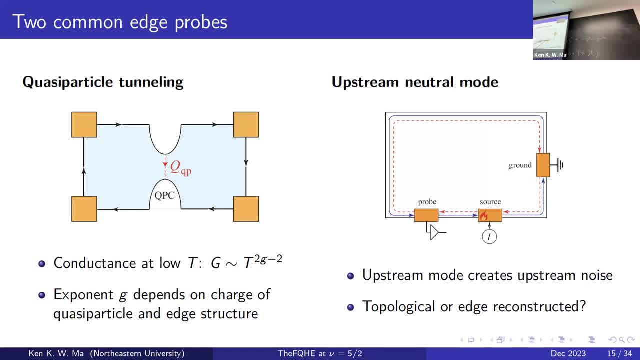 but it still carry energy. okay. So let's say, if this upstream mode exist, then it is being hit up by this hotspot and then when it propagate to the probe, then it will generate excess source noise here compared to the case with no upstream mode. okay, 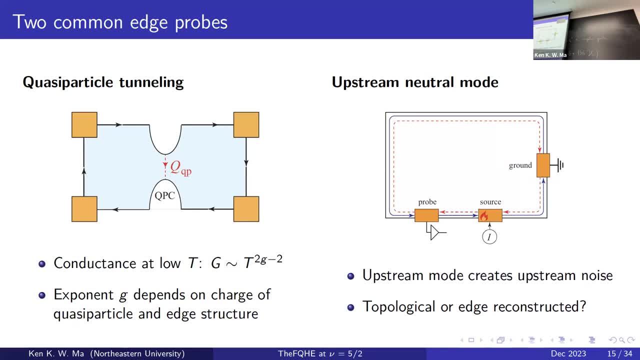 That's why, if you see excess noise here and then if you can do some control experiment showing that that upstream mode is actually topological, is not actually constructed one, then you can see okay, then you can differentiate. let's say: 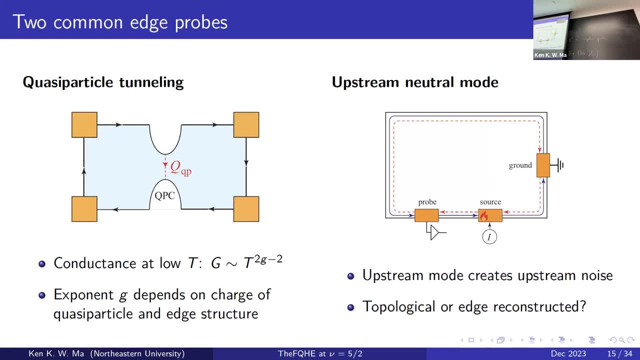 for farfetched and anti-farfetched: okay. For farfetched, they don't have. it does not have any upstream mode. let's say, For anti-farfetched, it has. okay. That's why this upstream neutral mode experiment. 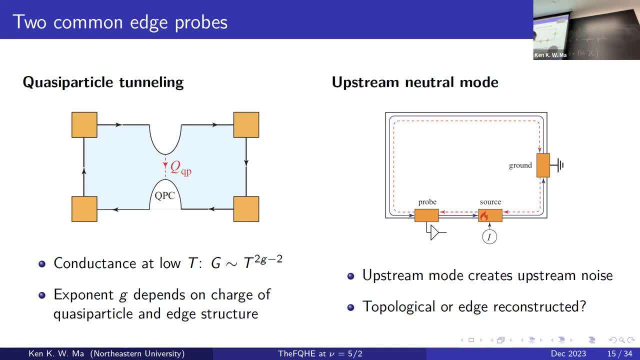 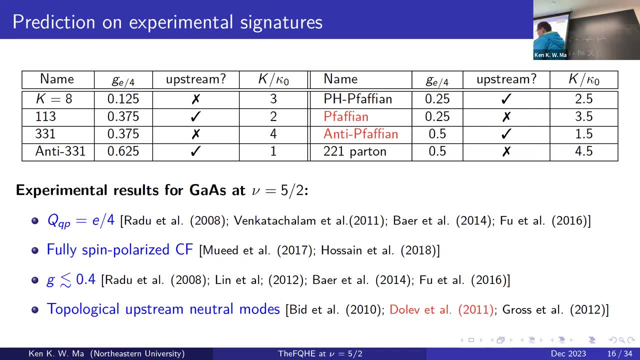 may also give you useful information. yeah, Yeah. and then we also list out what are the experimental signatures for different possibilities, because we we identify a more unified description of different possibilities here. So let's say, if we calculate that tunneling exponent, 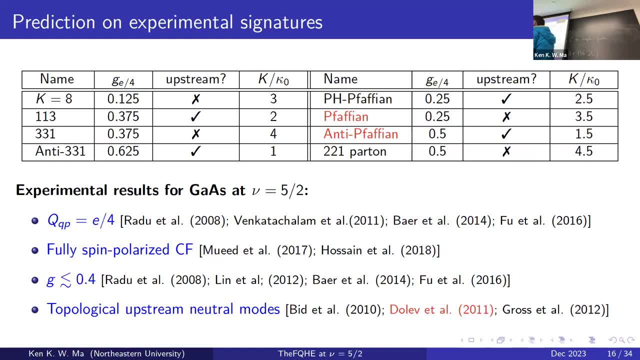 by assuming that the quasi-particle that tunnel actually has charge U before. okay, We can find this result. This is a theoretical prediction. okay, And then whether that edge has upstream mode. okay, Quasi means that it doesn't have upstream mode. 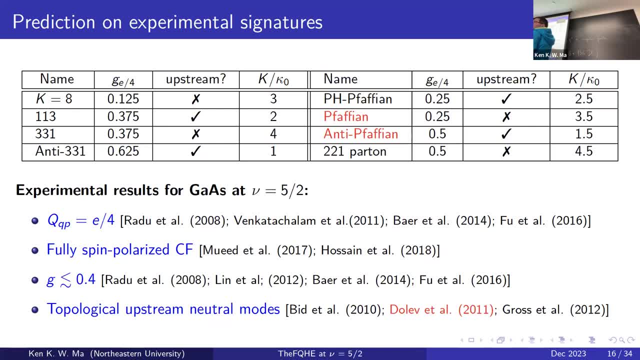 And then this one. I will talk more about that. It's the thermal bond conductance. okay, Yeah, so let me tell you, let's say, for gallium acetylene, a fueling factor, five-part electron density around three times 10 to the power 11. 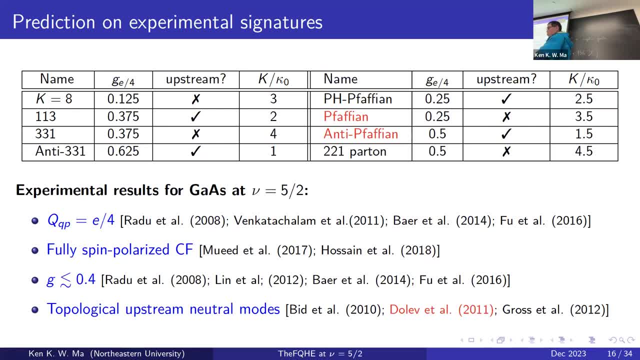 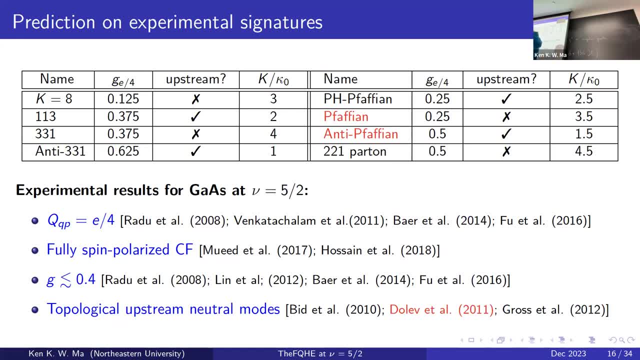 Which one is being realized. But it's very important check, okay. Then people also find that the composite fermion spin polarized, Yeah, And other information is that when they measure the value of g, they found that it's actually 0.4.. 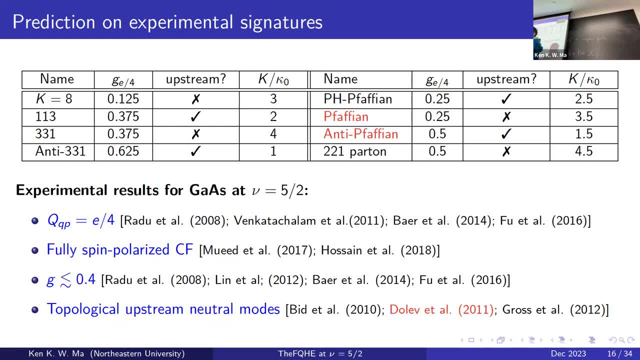 But the experimental value is like an upper bound, because in that level of constriction you also have like cooling direction and probably you may also have edge reconstruction. All that, in fact, will increases the value of g that will measure. That's why the g that you measure in experiment, 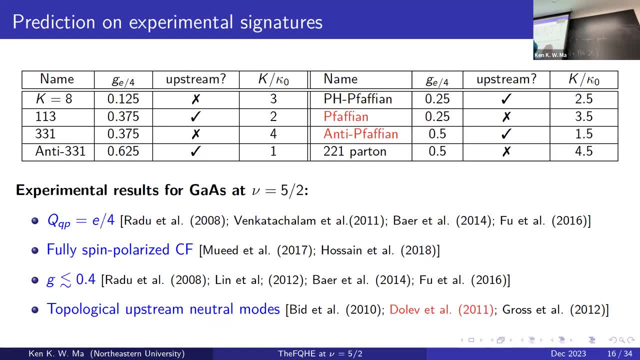 is like an upper bound, okay. And then they have an upper bound, what we like- 0.4, okay. And then when they do a neutral mode experiment, they actually see topological option, neutral modes Now. so from numerics, okay. 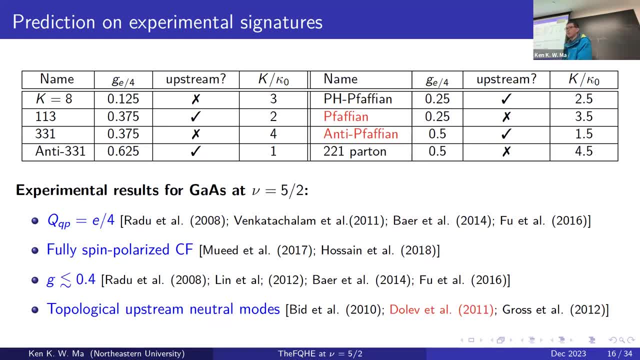 From numerics. farfian and antifarfian are usually favor. okay, But let's say, let's say we want to to interpret this experiment. let's see what happens. I told you that this g is an upper bound right. 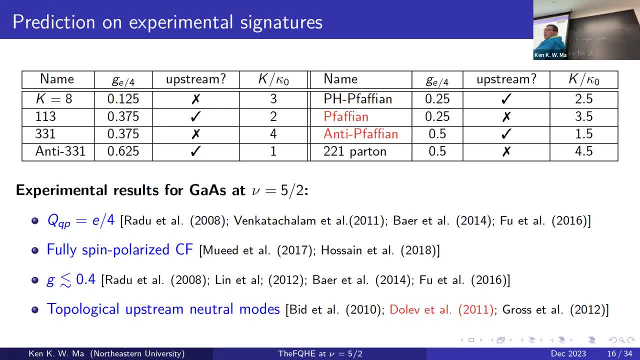 0.4.. If you look at farfian, okay, right, But if we look at antifarfian, seems that too large. right, It's 0.5, seems to be too large, But now then you may say, okay, no problem. 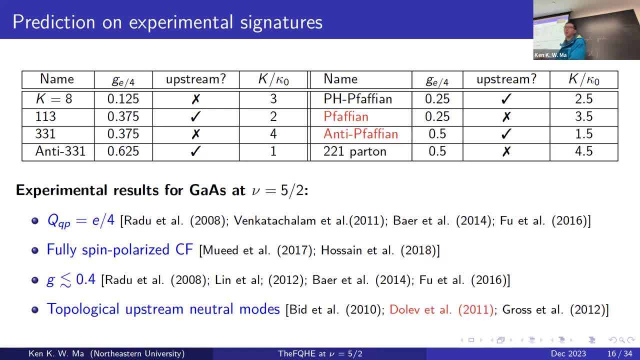 Then I just say: okay, the farfian state is probably described as farfian state, No problem. But now we also see that there are topological option, neutral modes. but if you look at farfian, there are low, there are low, there are low. 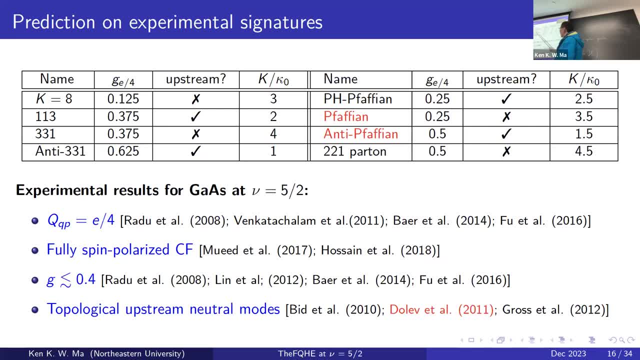 there is no upstream neutral modes. Farfian cannot explain both experiment. naturally, You can always find some, you know, more hand-waving or I mean more complicated arguments to explain any type of experiments. right, I mean more more complicated arguments to explain. 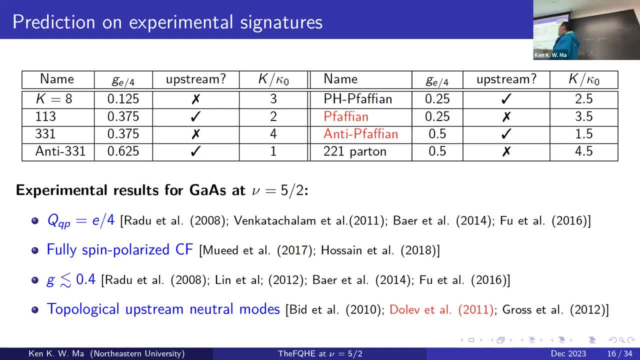 any type of experiment. but if you want to explain it as in naturally at the same time, it is true, It seems like farfian or antifarfian cannot explain. Yeah, So what happens? Can you briefly summarize Like particle charge and scalarization here? 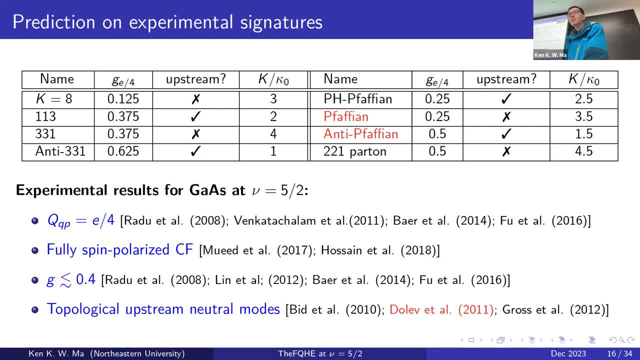 and the upstream modes. which of them are coming from the quantum of fine tunneling? Yeah, sure, So for quantum, for the tunneling, it's like this one and then this one. Yeah, actually, in the tunneling they also measure short noise. 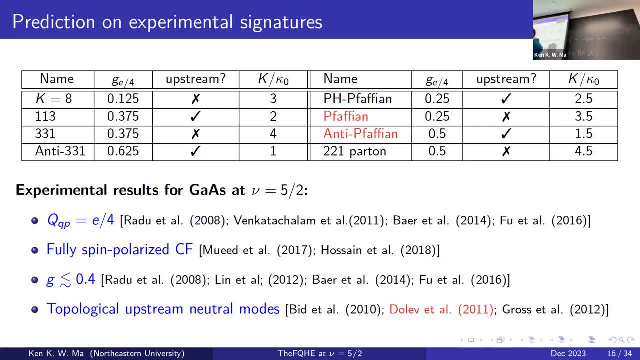 but they actually did some fitting and then when they do the fitting, they actually fit this Q and T at the same time, If I remember correctly. yeah, That's why these tools- and you can see they- come from the same reference. 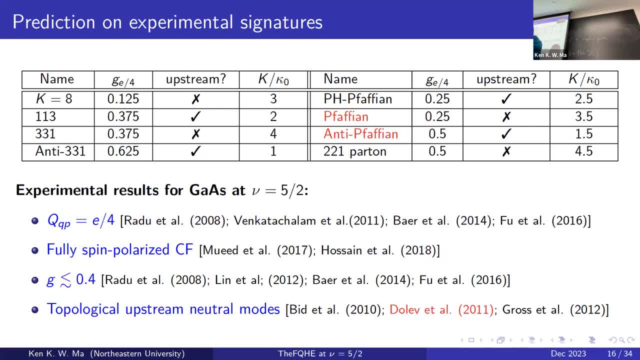 This one are more from fossil particle tunneling experiments. And then this one, I think it's to measure geometric resonance of that Fermi C, something like that. yeah, And then for this one is the upstream short noise experiment that I showed you in the previous slide. yeah, 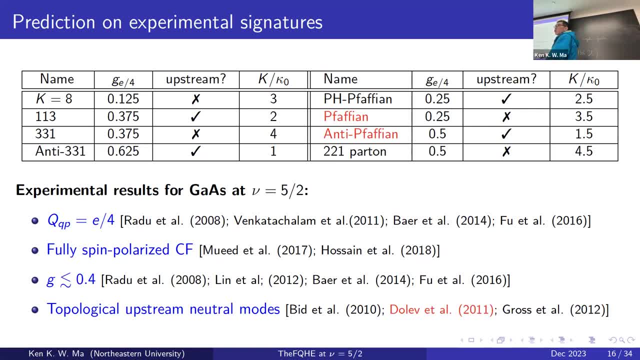 And then they also compare it to seven over three, the fielding factor, because that fielding factor it's a strong belief that there should be low upstream mode, and then they can compare, like the noise spectrum, and see whether that noise that's observed at five half is whether it's 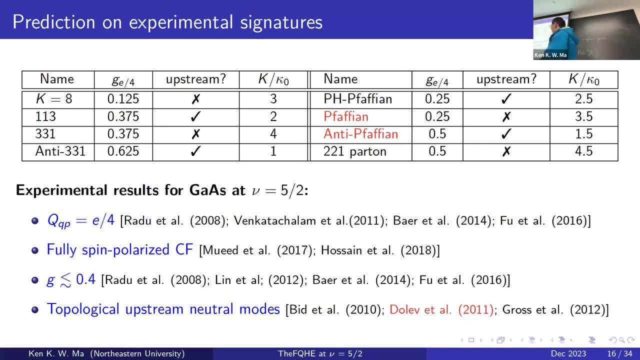 from edge reconstruction or from topological origin, And they claim that it's really topological. That's why it seems like light or dark or anti-farking can explain both. laterally okay, But of course, as I said, you can always. 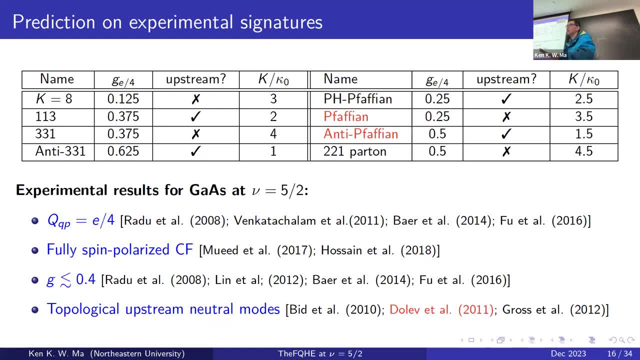 always make more complicated argument to explain any type of experiment, right? So the leader will discuss how to differentiate exactly edge reconstruction and topological origin. I will not go into the detail, but this reference- yeah, the slide- they need to compare it. 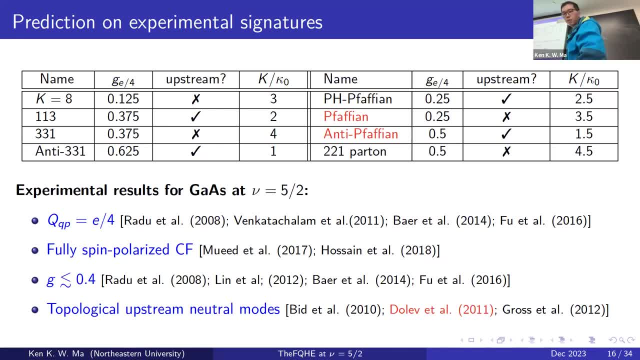 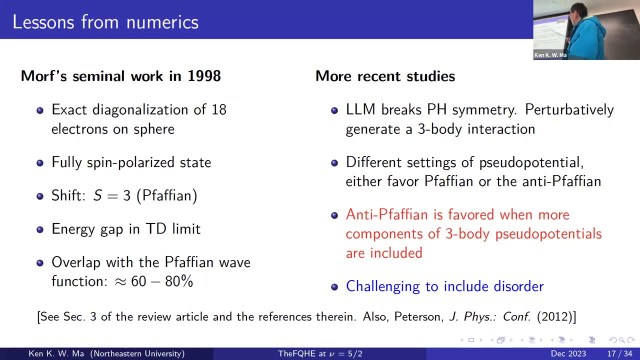 to other quantum post states. yeah, So so far I just tell you what happens if I just focus on fossil particle tunneling, I just focus on upstream neutral mode, Yeah, and then I also need to tell you about a little bit about what numerical 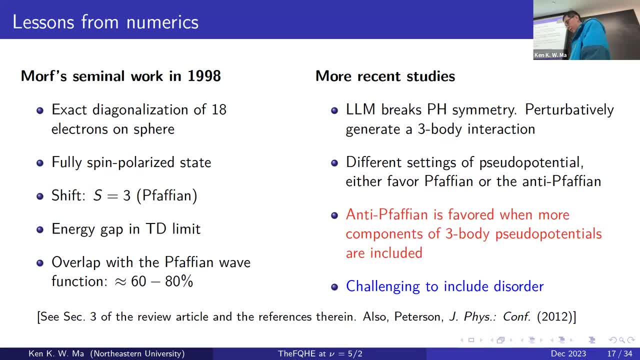 not what numerical simulation tells us. Actually, actually, at the beginning, people are very- how do you say? a little bit skeptical about Mori state, because it's too good to be true. okay, But in 1998, Morf published a very, very important work. 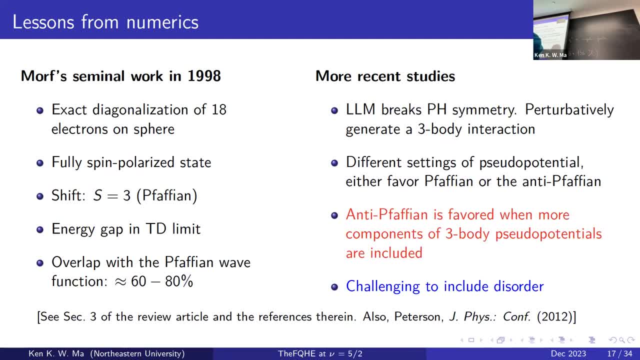 is really showing that. let's say, at least in spherical geometry he observed the current state of factor state. yeah, That's why it motivate a lot of numerical study afterwards to see whether it's this depends. yeah, And then more recent numerical works. 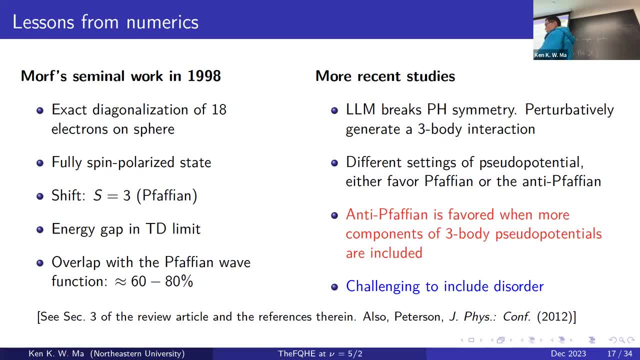 are actually try to have a more realistic, let's say, pseudo potential, because if you also include, let's say, lambda level mixing effect, the pseudo potential, not only two body, you also have three body, but though you cannot include even that many pseudo potential. 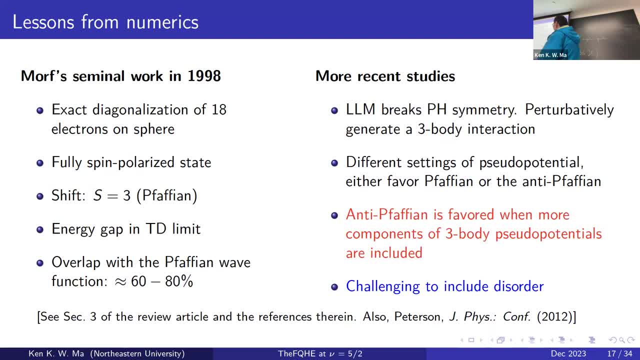 you need to stop at some point. But people find that if you, let's say, include more three body pseudo potentials, then the anti-Fafnian state is actually favorable. let's say, in numerics, okay, Yeah, but the message here is that 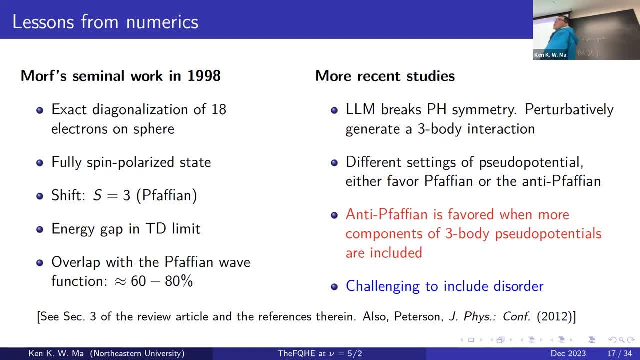 it seems like, in numerics, either the Fafnian or anti-Fafnian is favorable. yeah, That's the main message that I want to convey to you this night. So, yeah, probably I need to speed up. I mean, yeah, sorry about that. yeah. 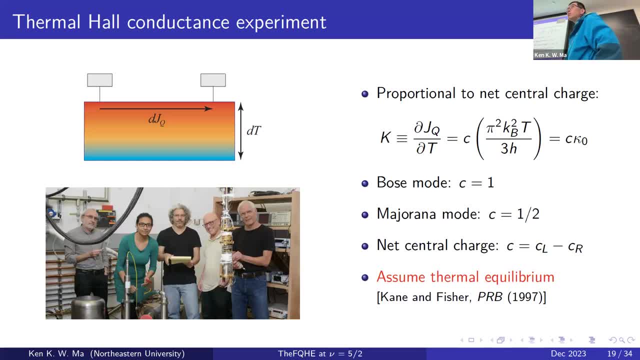 Yeah, okay, so Sorry. So externa people now consider P-H-Pafnian is of most, yeah, like realizable. So can you repeat The P-H-Pafnian is so externa people consider P-H-Pafnian. 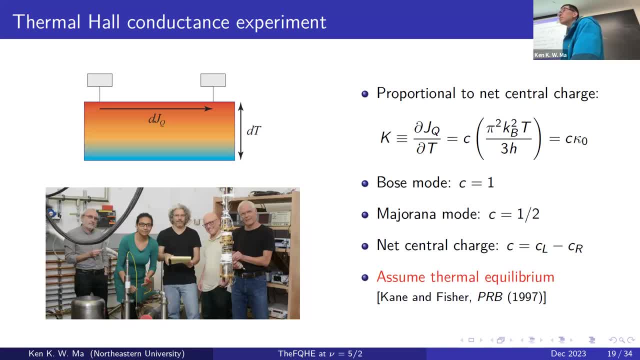 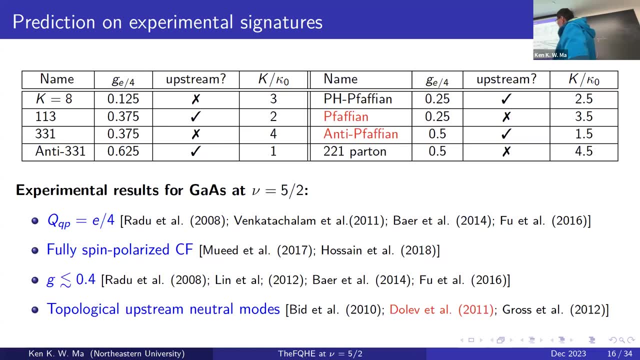 is most realized state. Yeah, I will actually discuss why. I can repeat once more here. If you want to combine, let's say, these four findings: numerically people think that the Fafian or anti-Fafian are probably the two most promising candidates. let's say: 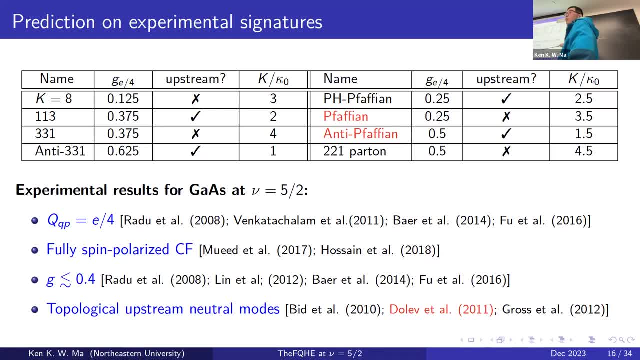 But if you really want to explain this, for let's say at the same time, naturally, it seems like neither of them can do that. That's why they want to come up with other proposals. But here I just tell you two types of experiments. 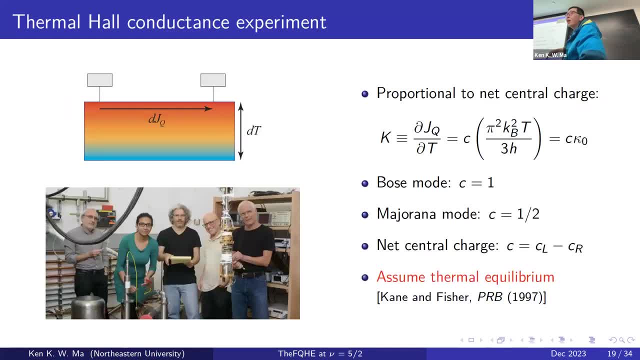 That's why now I want to show you the third type, that is, the thermal hole inductance, And why people nowadays- a group of people- think that PH-Fafian is probably favorable is actually coming from this experiment. So, besides doing quasi-variable tunneling and upstream neutral mode experiment, another 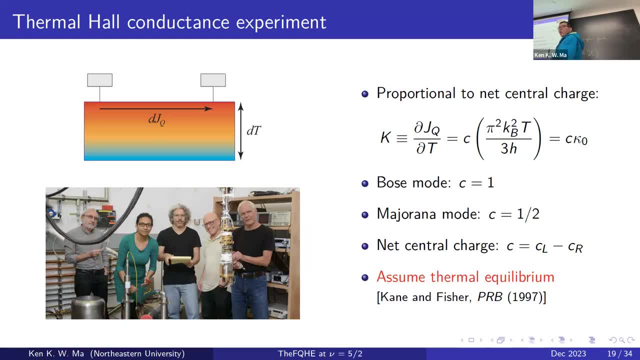 thing that people can do is thermal hole inductance. Of course, it's very difficult to do, but in 2018, the Weizmann Institute group succeeded. Okay, And then let me try to let me remind you what it is. 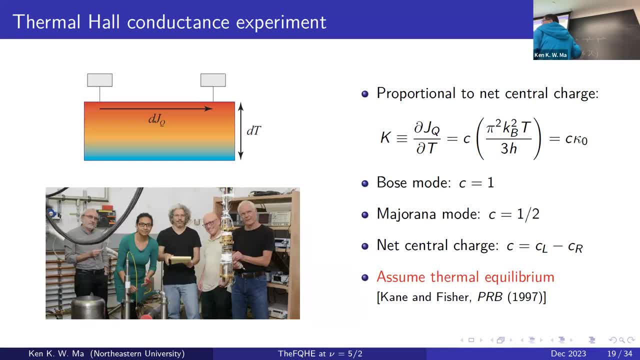 So the thermal hole inductance will take this form: okay, or it means it's like if you send a. if you send, I mean if you have a temperature gradient here, then you generate heat current and then the ratio between these two quantities, the so-called thermal hole inductance, and 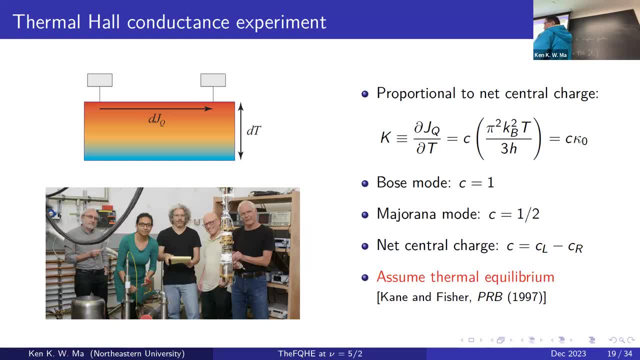 then this. So for this thermal hole inductance, the important thing is that it is proportional to the central charge of the edge of your sample. This C is the central charge. okay, This one is a. let's say probably I should put a T here. sorry about that, yeah. 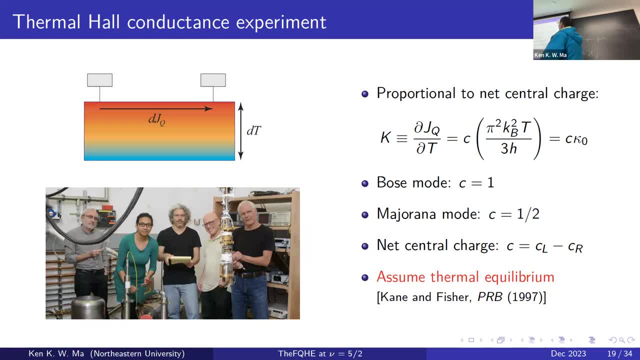 But the important point here is that it depends on the central charge. And then for each Bose mode, okay, the central charge is one. And then for each Mairana mode, the central charge is one, half, Okay, Okay. And then if you have more than one H-mode, then how do you see you do addition and subtraction. 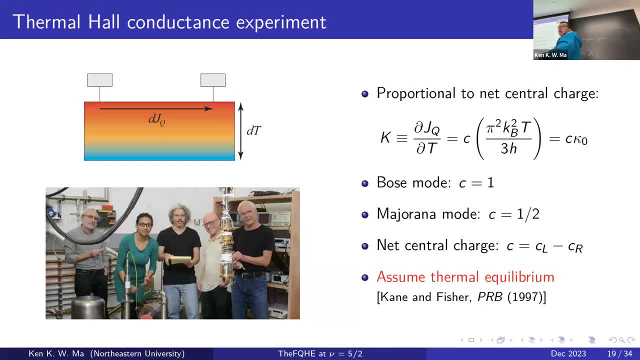 If these modes move in the same direction, then you add them up. If they move in opposite direction you do the subtraction. okay, But here there is an assumption. I assume that two modes in opposite direction they already firmly degraded, okay. 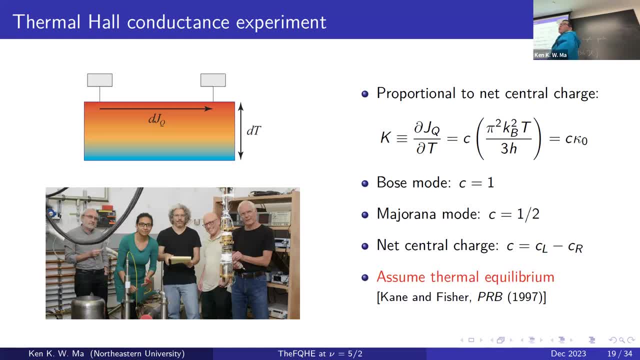 That's why I can't do the subtraction. okay, This is a strong assumption. okay, And I will explain to you why this assumption- Okay, This assumption probably- is important if you want to really understand the nature of the state. Yeah, 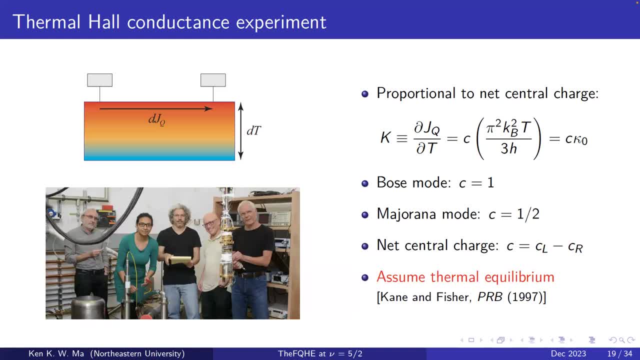 So let's see what the result is. This Bose mode: the central charge is one On the photo. it's the Weizmann Institute group. Yeah, Yeah, I should also actually add that Dimmer-Fellman here. Yeah. 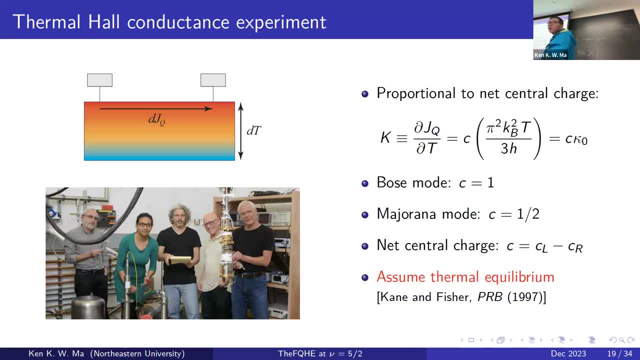 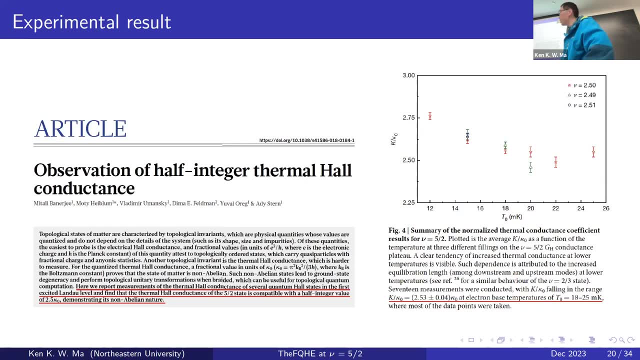 Yeah, It's a- I think it's a literature paper in 2018.. Yeah, It's the Weizmann Institute group. Yeah, Yeah, Yeah, Yeah, Yeah, Okay, Yeah. So it's this paper. It's this paper. 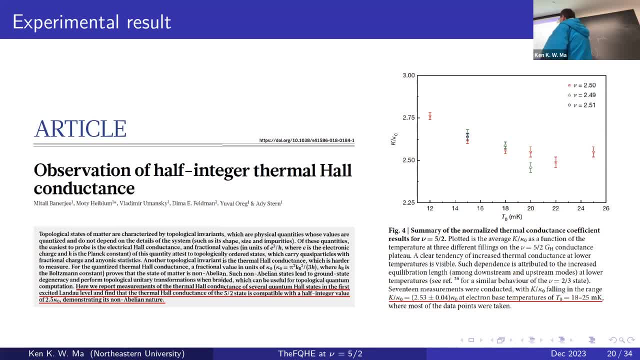 Yeah, Okay. So what we observe is actually 2.5.. Let's say around 20 milliKelvin, Right, It's 2.5.. So let me go back. Let's say several slides before 2.5.. 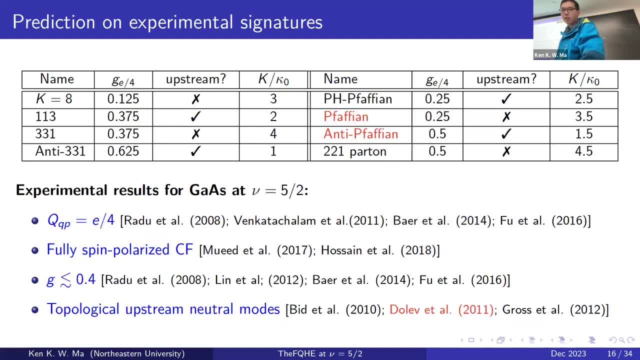 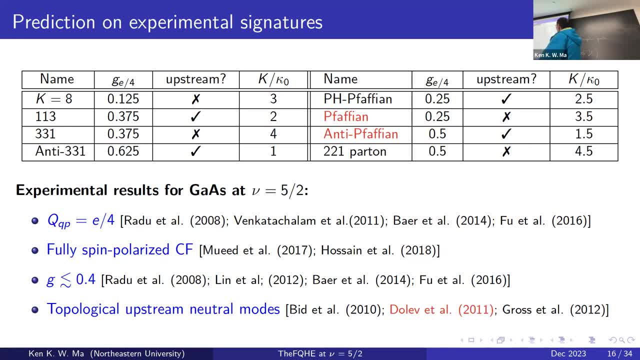 Right acao: 2.5, Smile, 2.5.. The remaining now female sample is already fully equilibrated, firmly equilibrated: Yes And 1.5.. Upstream models: Yes, Where there it is smaller than 0.4, but G. 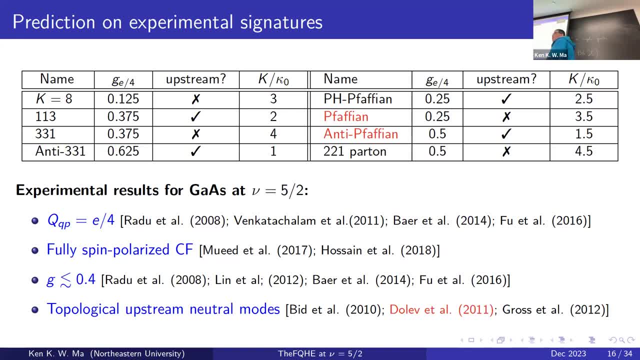 Yes, These helicopter, if it's not only economy calibrated, Does this tell you upper bound, and I will also talk about that. Yes, That's why people also questions about Whether that formal current experiment, But I will certainly talk about. 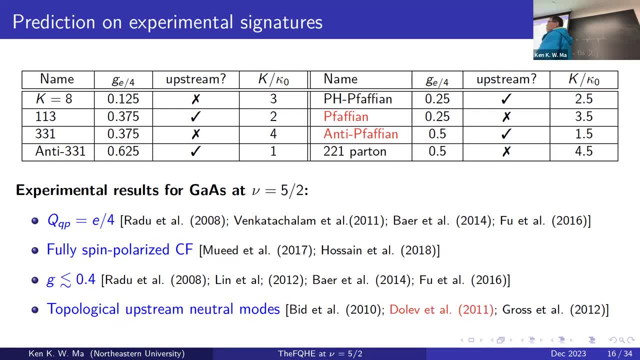 really tells you it's pH 5 or not. Yeah, I will discuss this in more details. yes, But if you really okay believe I mean the experiment is carefully done, okay, But let's say we really assume the edge is fully, firmly equilibrated. 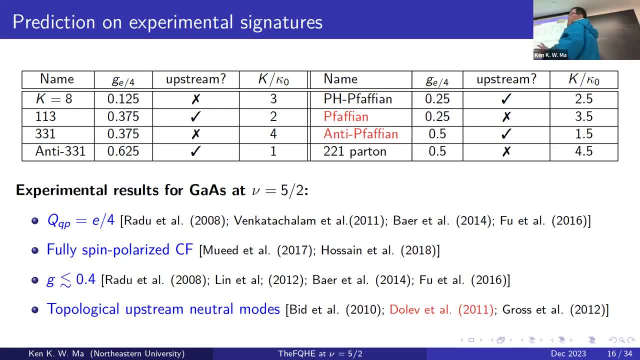 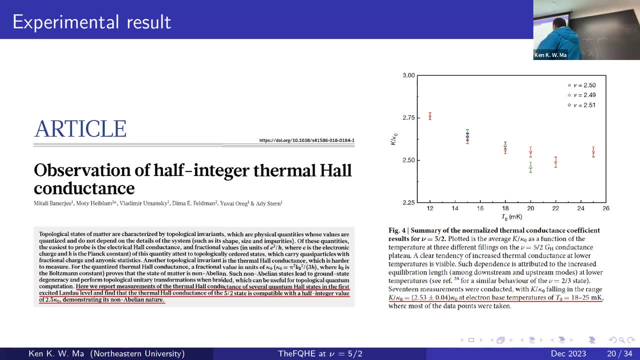 then that 2.5, you see, can only be explained by pH 5. But of course it's an assumption, okay, That's why people can always ask: maybe your sample is actually fully equilibrated, right? Yeah, So actually here. 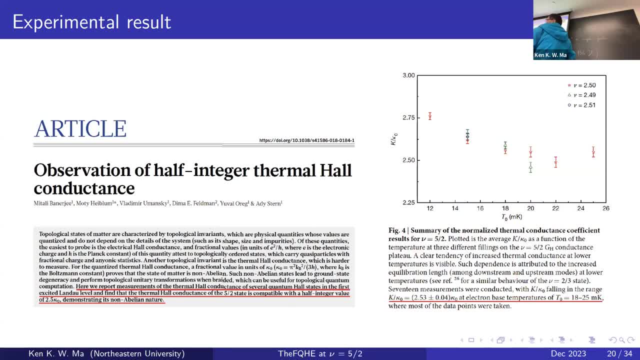 actually there are two features here. I'll just tell you one, okay. One feature is that 2.5 around 20 milliKelvin. Another feature is this thermal hot inductor actually shoots up okay when lower temperature. I will also explain to you why it shoots up okay. 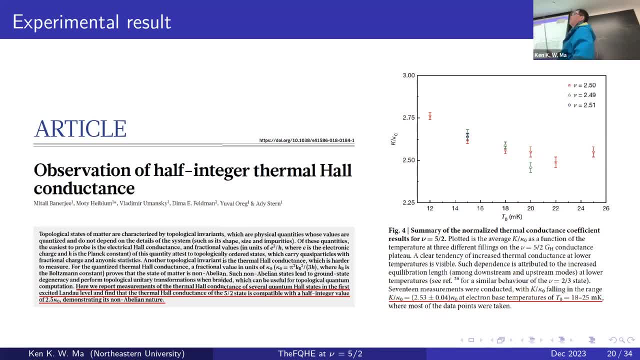 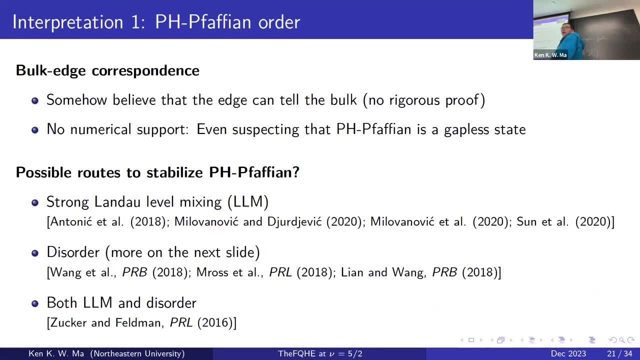 This feature is equally important. okay, to this. 2.5, actually, Okay. so what this experiment tells us? okay, 2.5 thermal hot inductor: Okay, first possibility is: if you believe the edge is pH 5, then how about the bulk? 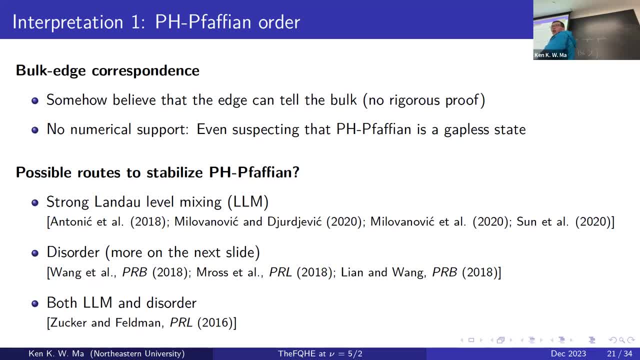 I mean, it's a topological system, right? We have bulk-edge correspondence. okay, If you believe in bulk-edge correspondence- no, mathematical, that was true, okay, If you believe in that, okay, then I can claim, okay. 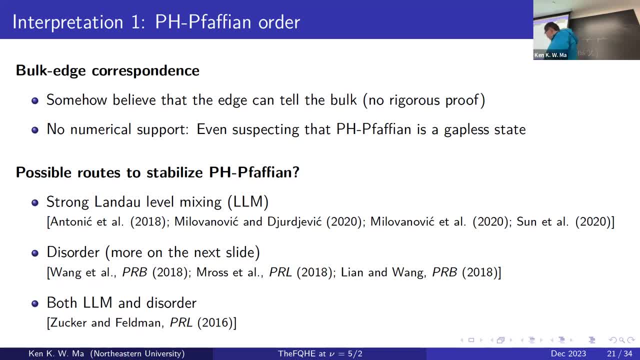 the edge is 5.5, then the bulk pH-Fabian, then the bubble is also pH-Fabian, Then end: okay, We solved the problem- at least one of the problems of 5 1⁄2 state okay. 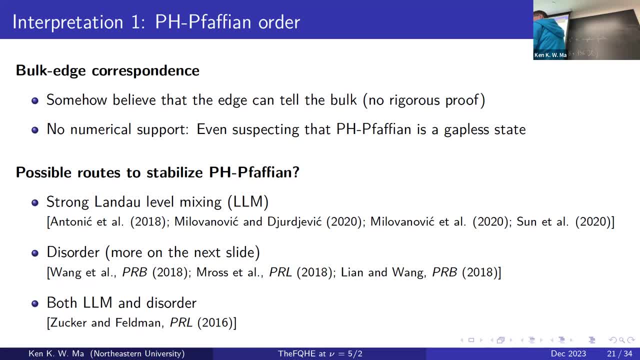 End. Then you may ask- okay, pH-Fabian, it is really the case, then- why people never see it, let's say, in numerical simulation? It's a good question for us, right? So that's why there are different proposals, right. 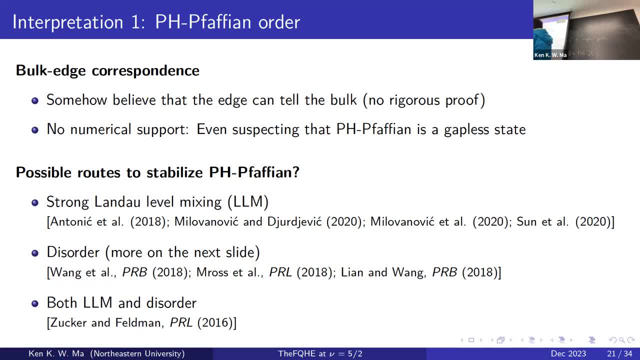 being introduced. One of the proposals is: probably it's due to the low-level mixing, let's say, because in numerics it's very hard for you to really treat LLM very, very well, okay. Another is: you know, in realistic sample. 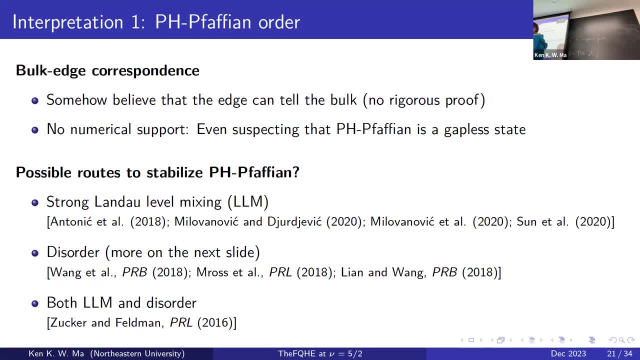 must have disorder, but in numerical simulation it's very challenging for you to really improve disorder. And then of course you may also think: okay, probably both LLM and disorder are important. And then of course you may also think: 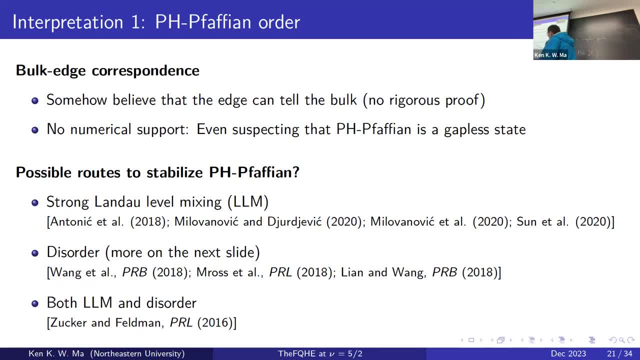 well, what's the best way to stabilize the pH-Fabian right? These are some of the proposals that people have introduced, okay. And then doing numerics- not totally possible, but challenging. okay, But challenging. I will also show you some more recent developments. 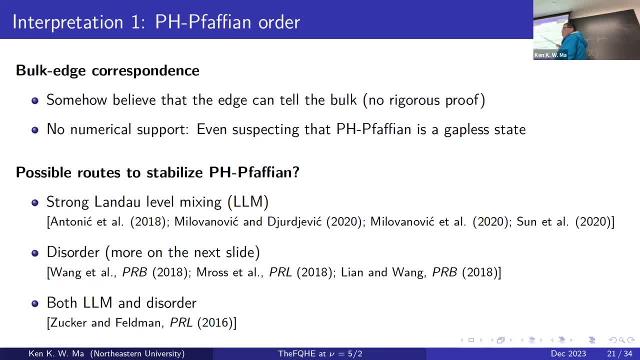 what happens, let's say in numerics. But this is one of the explanations or one of the interpretations of that 2.5 in Fermi-Hall-Dutton experiments. Now, okay, let's say the edge is pH-Fabian. 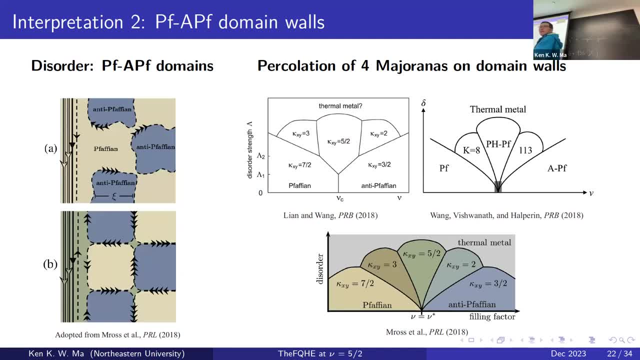 Does it really mean that the bow should be also pH-Fabian? It turns out probably not, okay. So there are three paper actually coming, I mean coming out, you know, the days are very near to each other- also in December 2018 or the end of November 2018, okay. 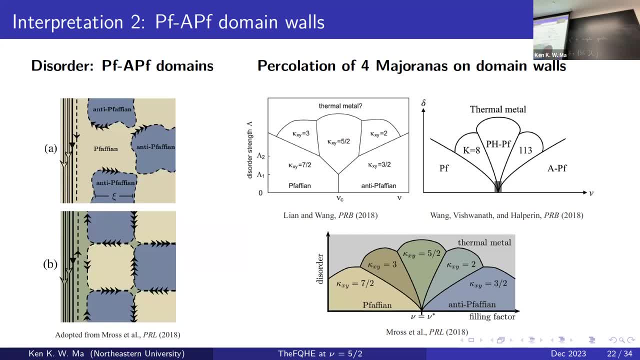 What they claim is like: okay, I believe let's say the edge is really pH-Fabian, But in the bow can I have something like this? Okay, let's say locally particle-hole symmetry program. let's say: 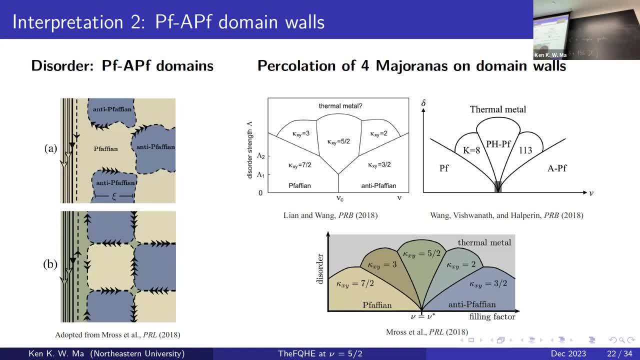 Let's say, I have different regions, okay, different domains, okay. maybe one of the maybe in this domain is, let's say, anti-Fabian, and then this domain is Fabian, okay, And I have all these Fabian, anti-Fabian domain, okay. 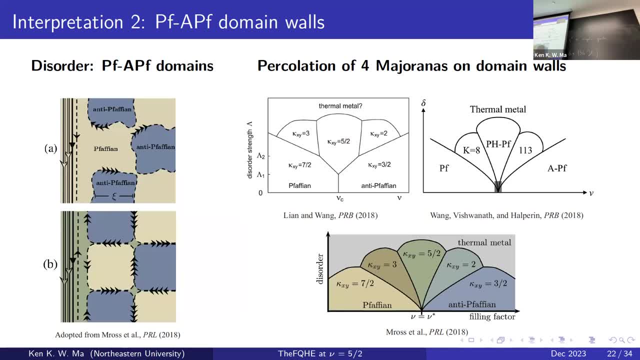 Then the consequence: I will now have four myorhinomoles, let's say running, Running on this domain wall, okay, And then, depending on the percolation, these four myorhinomoles, the edge can be in different phases, okay. 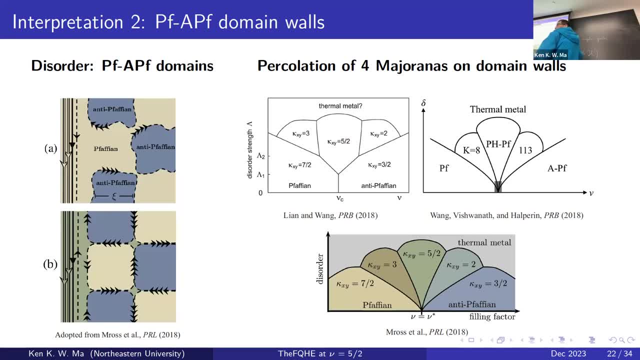 You can see the phase diagrams. they conclude a difference. But the message here is that let's say, if the bow, you have Fabian, anti-Fabian domain walls and then, depending on how, these four myorhinomoles- 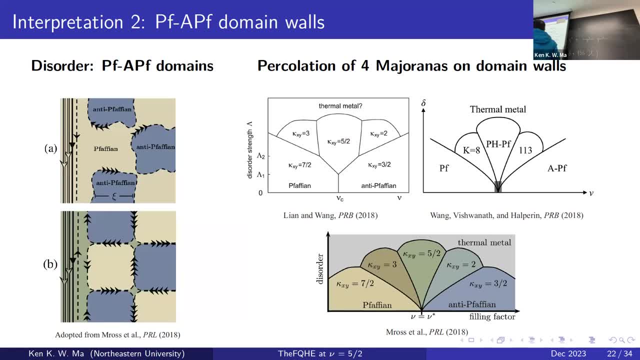 they percolate. This is what I said. Then there is a chance that on the edge you actually see Ph-fabian Right, Because the thermal horn that has only probably edge. okay, So this is the second interpretation. 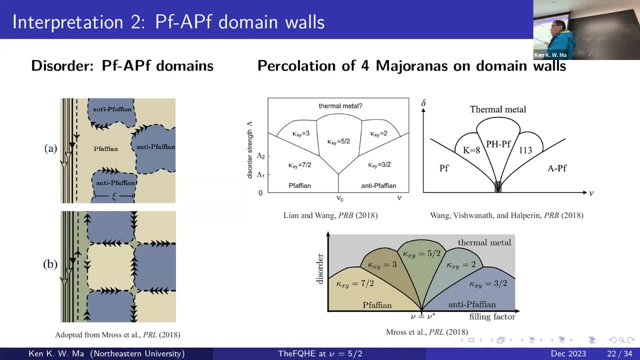 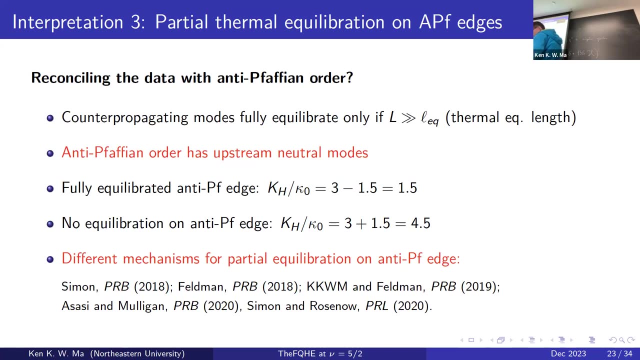 And actually Juven is the author of this paper, okay, So if you have any question about phase diagram, ask him. okay, Don't ask me Then the third interpretation is, as I as I said, the thermal horn ductance. thermal horn ductance. 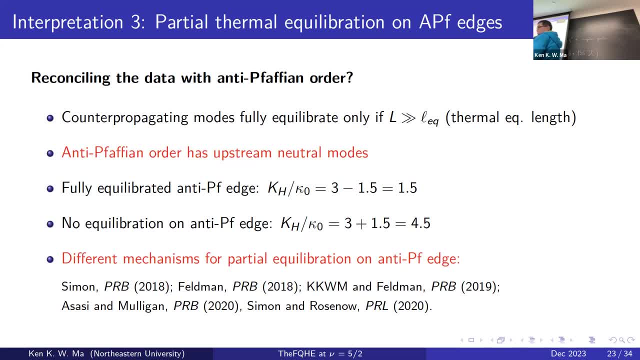 is proportional to the less than charge. But this statement actually is under the assumption that if you have counter-propagating, at-most you already assume these are fully, firmly equilibrated. How about if this assumption breaks down: okay, And then it also tells you that okay. 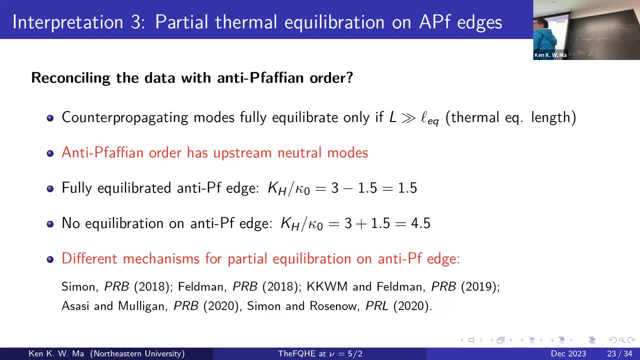 in numerics, the Fabian and anti-Fabian is usually okay. the more you know, have more support okay. So that's why people come up with different mechanisms. Let's say: can I explain that thermal Hall conducting experiment by having anti-Fabian order? let's say: The reason is that, if you can, 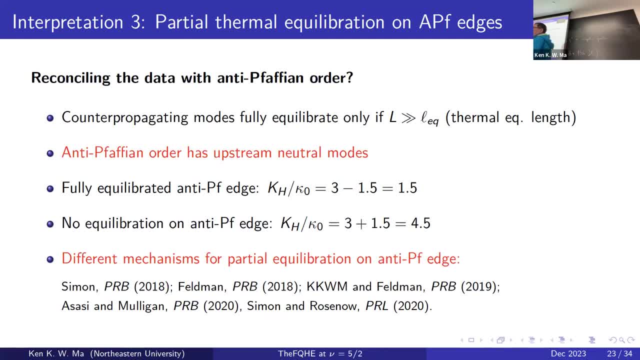 still record the anti-Fabian order. it has one downstream Bose mode and then it has some upstream modes, right, And then if let's say, if your sample is not long enough, let's say your sample is not long enough, then these two- I mean these kind of propagating modes- they don't need to. 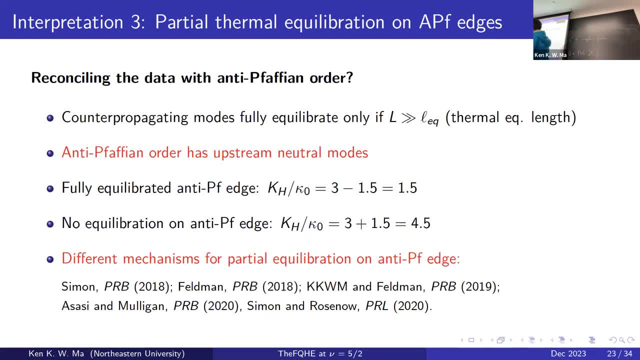 fully integrate. Then maybe can I use the black Fabian, Jeff, can I use it, Let's say, for anti-Fabian? so you have this one, okay, you have Bose mode, and then you have, let's say, 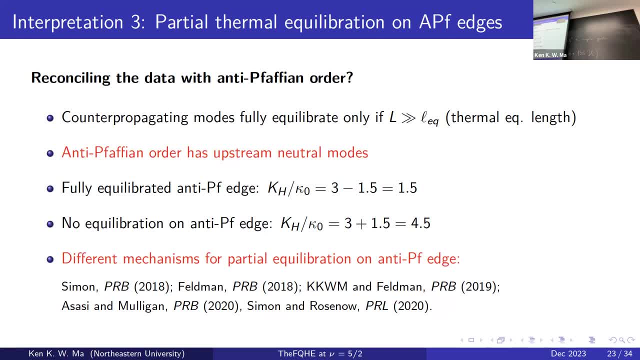 another. So if they are fully integrated you also have these two integer modes. okay, Let's say, if they are fully integrated, then what you have is like three minus one bar. then you get one half for C. okay, If you believe the X is fully integrated. But let's say, if there's no, 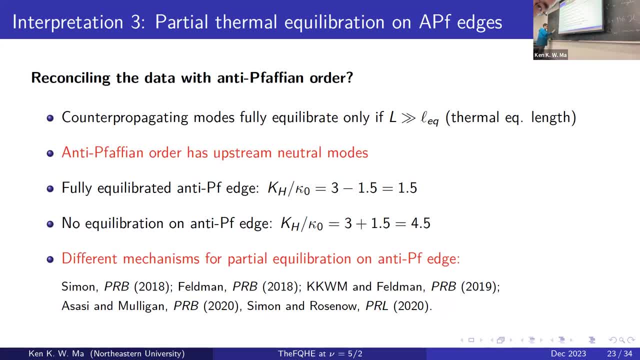 anti-deprivation. okay, then what you actually get is: so this one Can I drop here So that the audience can see from here: Oh, I see You want to use this one, Can I drop here? Okay, okay, you're going to need to drop there. 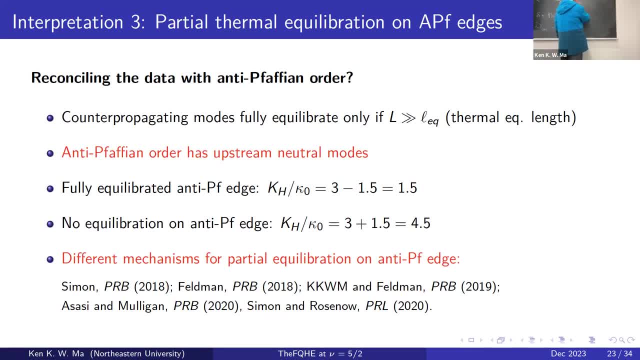 Yes, Yeah, I'm sorry about that. Okay. So let's say, for anti-Fabian: okay, you have. you have two integer mode coming from the two completely filled and out levels. okay, You also have another one for the half-filled and out level, and then you also have one upstream mutual modes. 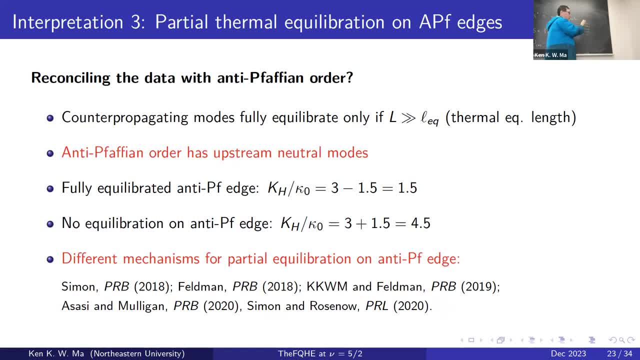 and then you have one upstream marginal, okay, And then if it is fully integrated, then you can calculate the less central charge. The less central charge is just one one one that is free, and then this one is one plus half. that is one one half, But if it is fully integrated, 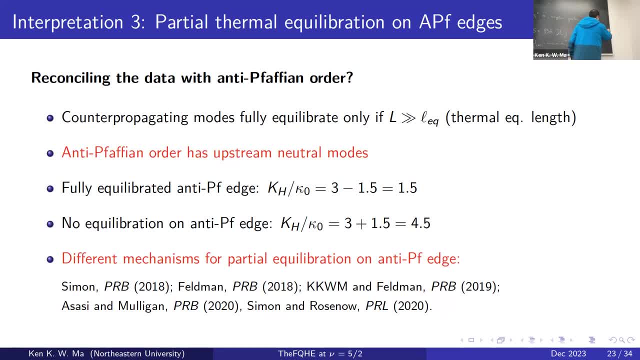 then you will have something like minus 0.5, that is 0.5.. But let's say, if they are totally locked- I mean there's low equilibration- then what you get is that you need to add them up. That's why it's 4.5.. So if there's, if, okay. 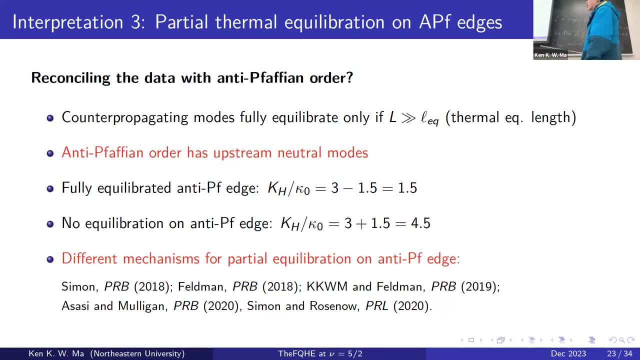 if there is low full thermal equilibration. actually you may observe any value in between 0.5 and 4.5. I mean 1.5 and 4.5. So why do you add them if they're not in the same frame? 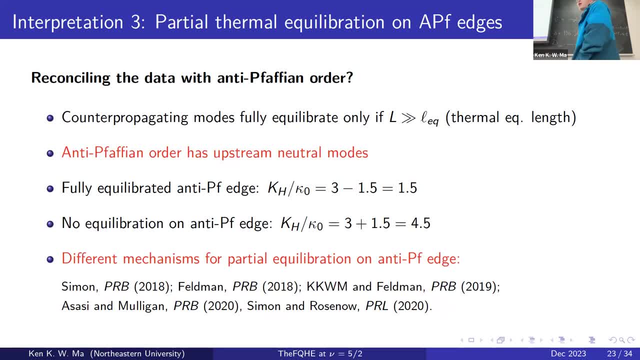 Hm. Why do you add them? Oh because, because actually you have two edges in the same sample, I mean in one, let's say in the sample. okay, you actually have upper edge and lower edge. okay, Energy always. 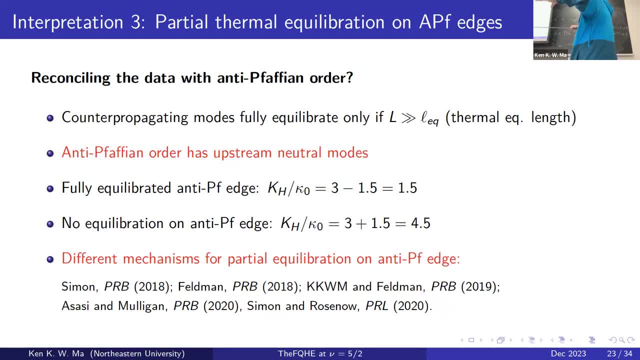 come from the hotter part to the colder part. If they, if, if, if none of these, I mean if they are not equilibrated, then let's say for the, for the upper edge, you have contribution from, let's. 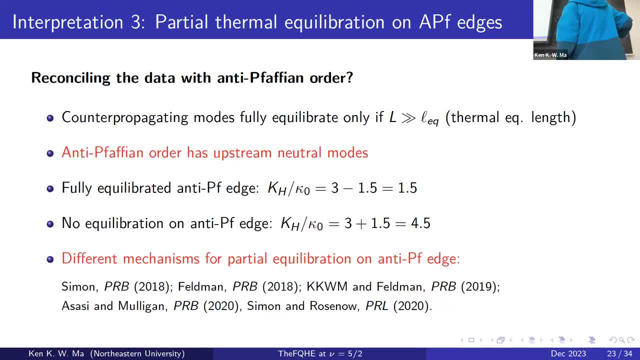 say this: free mode, okay. and then for the lower edge you have contribution from this. That's why you add them up. But if they already equilibrated, then the temperature of them are the same already. okay, That's why I use subtract. Roughly speaking, it's like that: 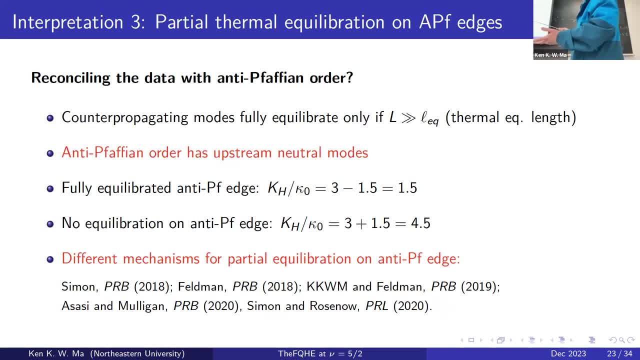 Is that okay? Yeah, So this is the third interpretation. It's like, okay, maybe your sample not long enough, not fully thermal, equilibrated, then I may probably explain it by antiphagia. Yeah, Yeah, And you see, there are different mechanisms to do it. 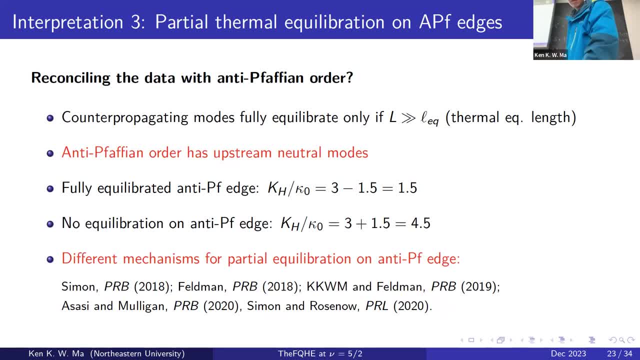 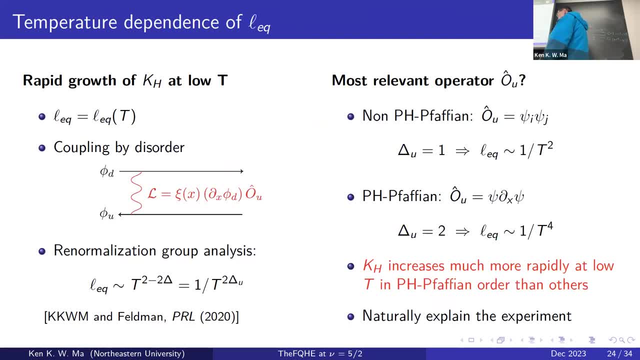 And then I also tell you, like, the second feature of the experiment is that not only 2.5 or 20 millikelton, if you go to lower temperature, okay, then you will see that K actually shoots up, okay, to around 2.7 or 2.8, okay, The reason is that. okay, the reason is that actually, 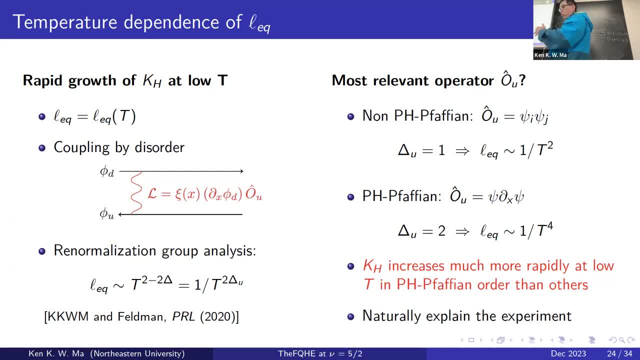 the length required for that kind of propagation. the length required for that kind of propagation because the thermal equilibration length requires actually the thermal equilibration length. okay, So even if I am talking moreDaniel佳麓基 기다� notes up K you'll see if these demonstrat esqu irrelevantius. 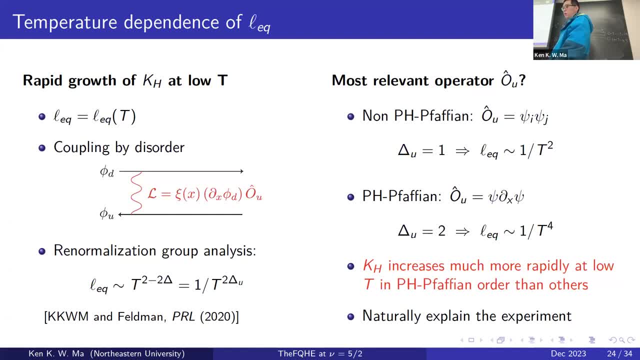 length required is actually longer. okay, Okay, Can you put this here? Okay, Can you put this here? Yes, Okay, Can you put this here? Yes, Yes, Yeah, You can choose respectively, just what you are. espera k, you need to place time. At the lowest one. Okay, Okay, Thank you for this great introduction. Thank you so much. If you like to see more technical and if you have questions, feel free to ask. at the end, abilities que es sucking by Courtney photo. See no questions or something. maybe I should, just because the next will be facing performance andarin or some specific 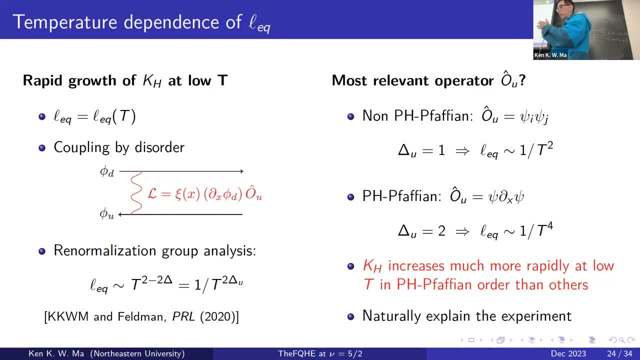 temperature, then it becomes harder and harder for you to have full equilibration on the edge. Now you can carry out a few theory analysis. I will skip the details. I will just tell you the result. The result is that if you look at the possibilities that I showed you before, 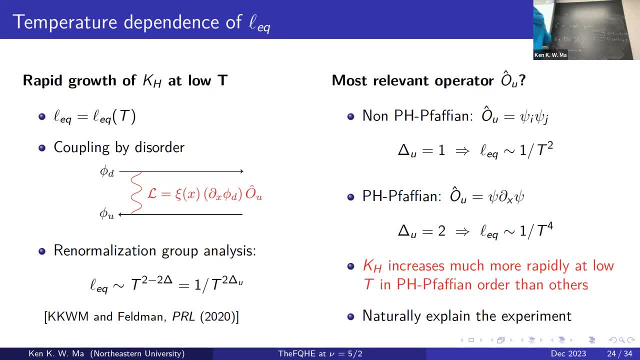 if it is a pH bargain, then the edge structure is very, very special. It has one downstream charge, both modes, and then one upstream, Marana. But you know, you want to couple them right. That's why the only thing you can write out is like: I always have the downstream mode contribution. 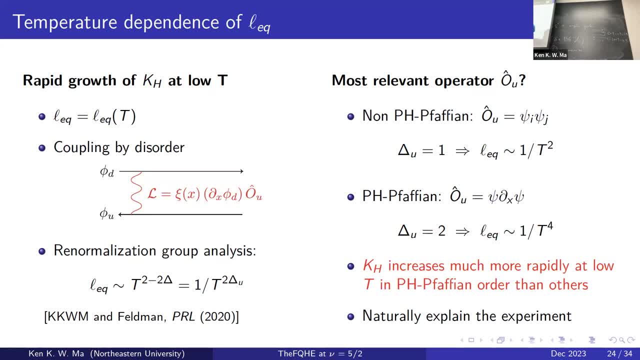 and then you know you cannot simplify the charge. What you have is the density. that's why it's hard to explain. But now the upstream modes. the operator describing the contribution of the upstream mode will depend on what is the edge structure. right? 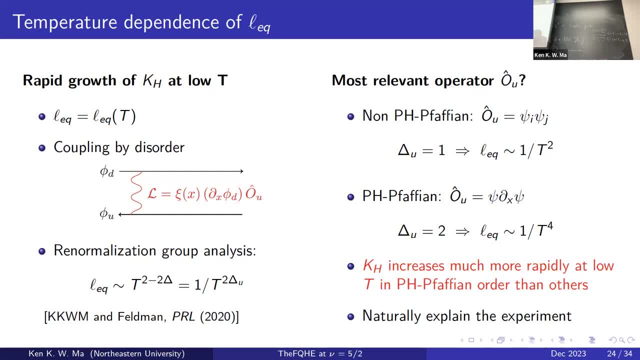 Let's say, for the pH, You only have one upstream Marana. okay, Then the most relevant operator that you can put here is log Psi. okay, Psi is not good because Psi is the fermionic. Any coupling term must be bosonic, okay. That's why you may think: okay, I can have Psi, times Psi. 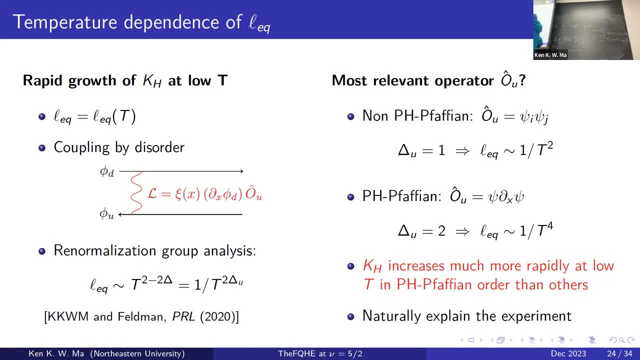 below Marana squared identity. That's why you cannot do that. The next thing you can do is actually Psi plus or minus Psi. okay, That's why the scaling dimension increases, because you have density. That's why you cannot do that. The next thing you can do is actually Psi plus or minus Psi. 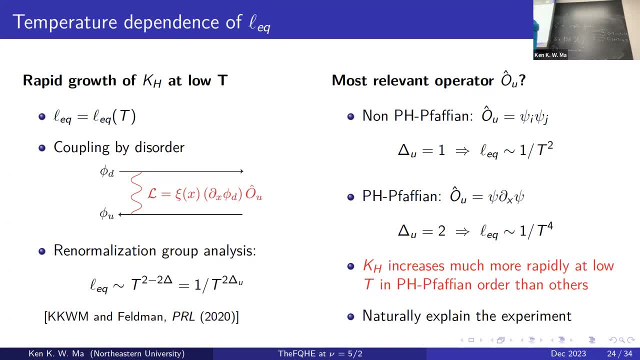 Okay, that's why you can do the logmasıgation group analysis, That's why you can do the work- análisis And you find that actually, if the edge is pH 5- 십° similarity, then the firing magification actually goes at 1 over T to. 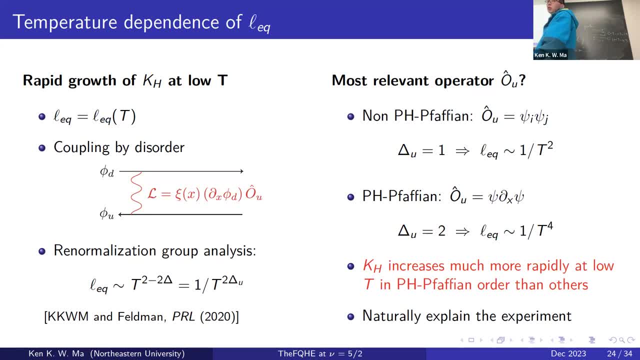 power 4嚴次. but for all other possibilities they they have more than 1, Marana. I mean, I only consider possibilities that have an upstream mode. okay, If they only have downstream mode, we don't have any useful for the migration. okay. so відő eks trung jomoànnhụ. 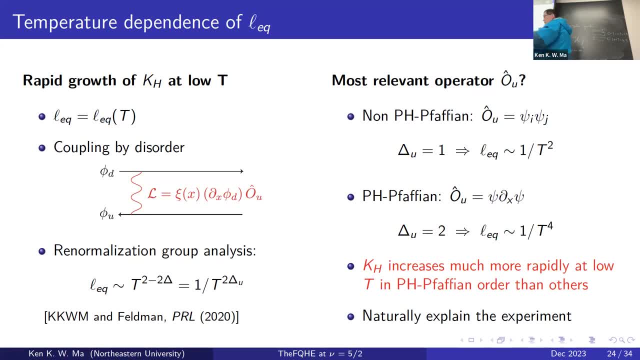 wechsel. we don't have any uhh ease to find information. okay, I only consider the possibility. li Chilei dạng el sẽ kem tiết đểist Kalimniмотрите at the low range toe d菜. I only concentrer the possibilities that mafingister à thermalилось foremeh. I mean, I only consider the possibility. 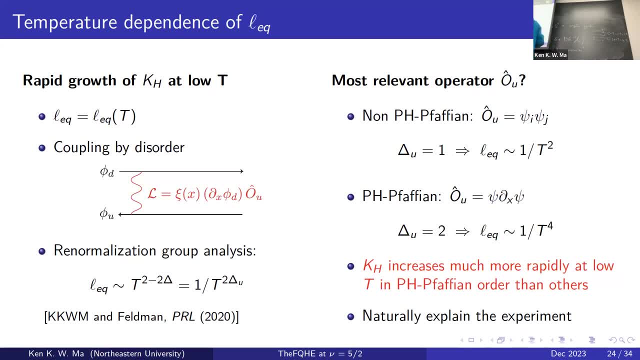 relative option modes. That's why, if I go beyond pH 5 and then consider other possibilities, let's say anti-Fafian, then this operator I can put is marijuana. let's say species. I times marijuana, species J, No problem, because this one they don't square to one. 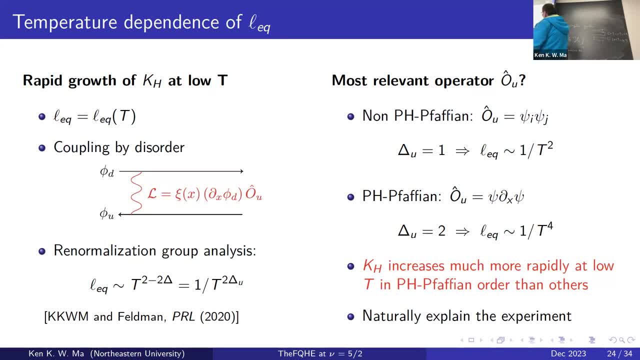 because they are different from our runners, right. And then this one, the scaling dimension is actually lower than this. okay, You can easily count. okay, this scaling dimension is just one, but this scaling dimension is actually two. okay, That's why, for the possibility that they are low pH, Fabian- 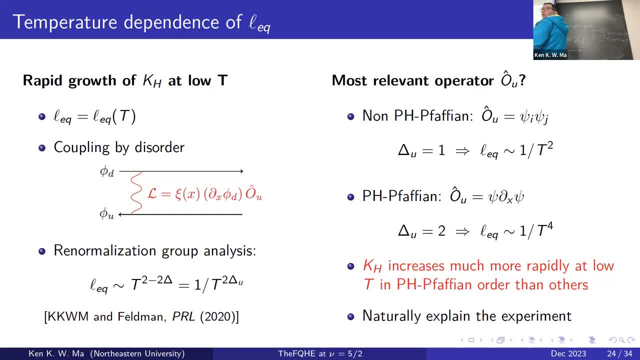 then below this length goes at one over T squared. And then this one: if you go to lower temperature right, it's clearly this length increases much faster. That's why you must have lower sample right. And then another thing is that if you keep your sample, 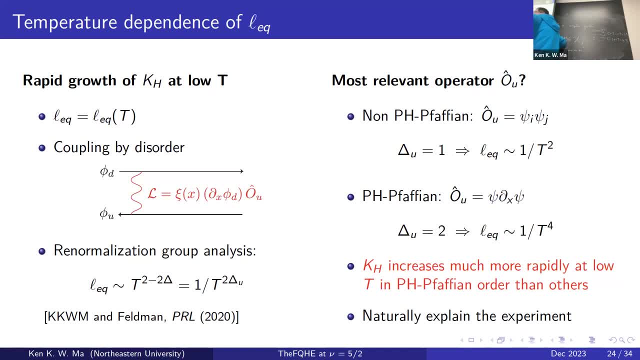 the length the same. if you go to lower temperature then this pH would go much faster than other quantum Hall states which have this LEQ scale. this one right And actually that grow in thermal conductance experiment at 5-R actually is much faster than other fuel reactors. 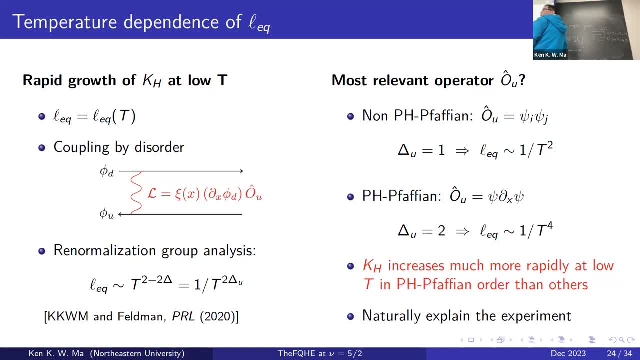 That's why it seems like 2.5 support pH Fabian. this growth also support pH Fabian, At least on the edge, okay, At least on the edge For the bulk, I don't know. okay, Different possibilities. 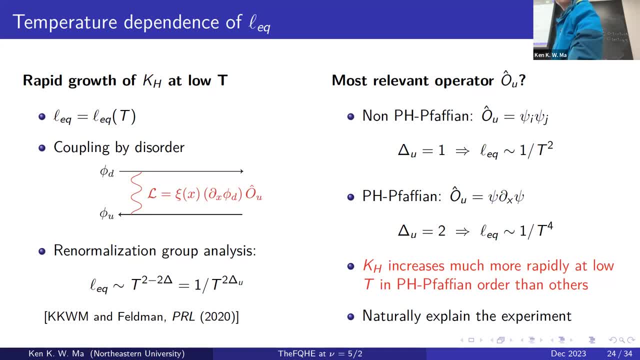 Is there any way to? Yeah, kind of some values at the computer scale of the experiment, of the simulacrate. really nice, Except value, I don't know, but I can tell you experimental value, Actually not in five, half, let's say, when people talk about two-thirds, because two-thirds is also a little bit special. 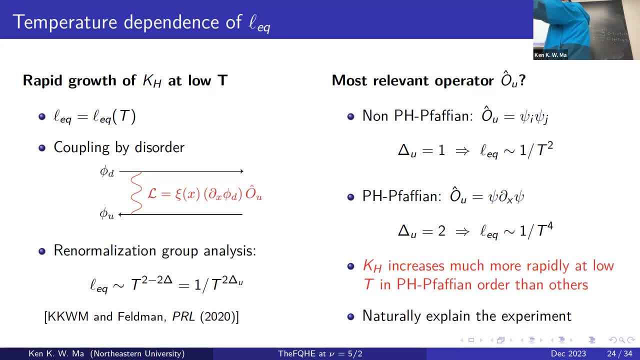 because they have one downstream Boltzmann, another upstream Boltzmann, and then if the number of downstream Boltzmann and upstream Boltzmann are equal, it's actually much harder to equilibrate than having different numbers of downstream options. And then in that case, if I remember, 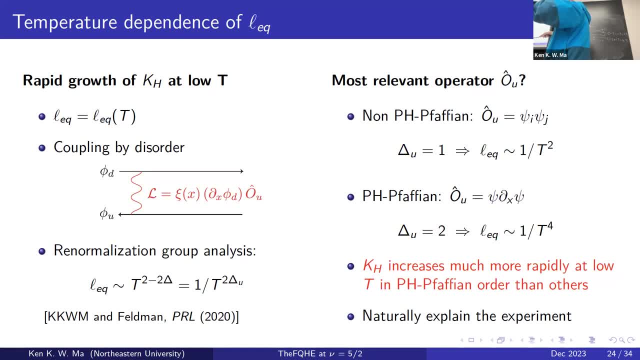 if I memorize it correctly, okay, in that two-thirds, that equilibration length is around 30 or 40 micron meter. I mean, it's like you need to. let's say you can plot out- I can't remember the exact data. 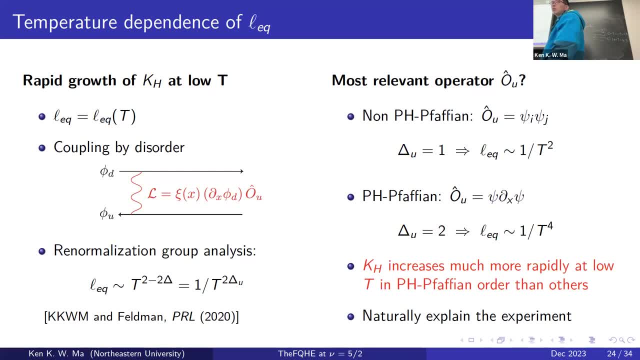 but yes, you can try to fit it out. yes, Is scaling also tested experimentally? It's not that easy because you also have other scattering inside, you also have other effects. but at least we can tell if it is really a pH-fogging edge we expect probably the growth is. 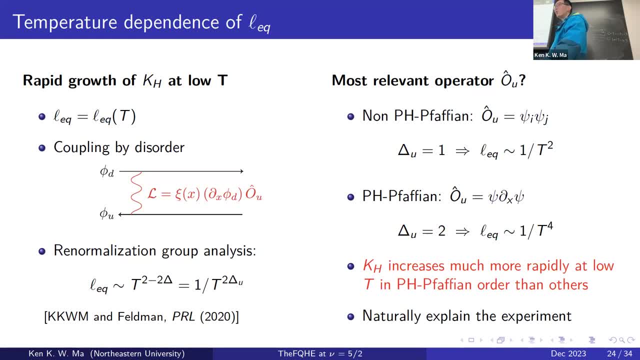 faster. We never really see one over T4 in experiment, we never. And another thing is like: you only see several data points, right? If it is really intrusive or not, I don't tell right If you just have five points or six. 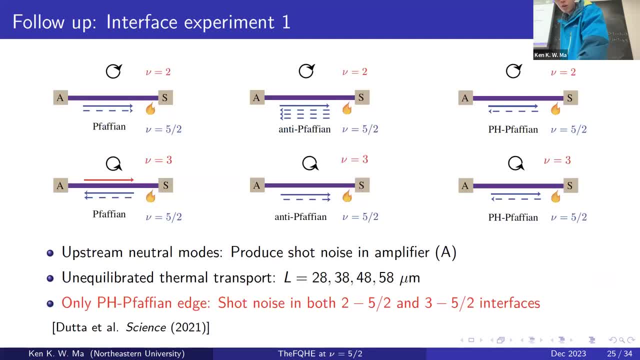 points right, Yeah, okay, so I tell you that it may be pH-fogging edge, but I also tell you different, other interpretation. That's why the Weizmann Institute group, they did some follow-up experiments. okay, The first follow-up experiment they do is like they consider putting. 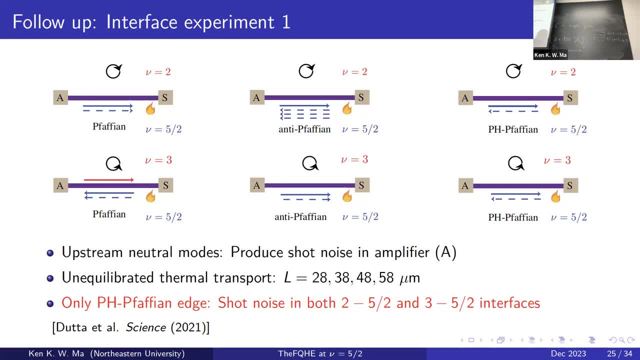 these new equals to tries. The first experiment they do is like they consider putting these new equals to tries. Okay, so the first follow-up experiment they do is like they consider putting these new equals to tries, or a little equal to three. column hall. 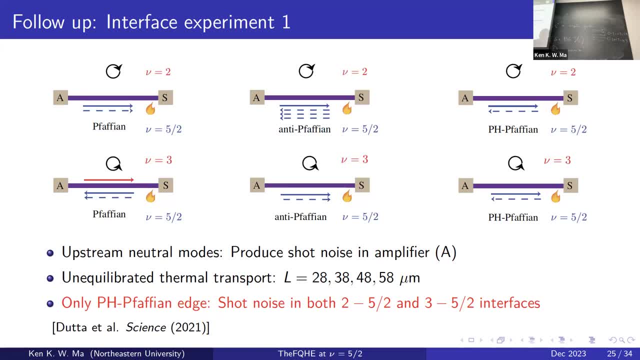 let's do this five-part and then, when they do it, then the integer modes are gap out and then what is left is something like that: okay, So let's say in this interface: okay, then we only have downstream. that's why we don't expect to have excess noise here. 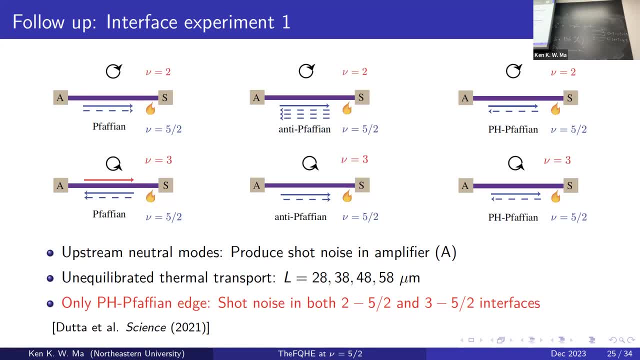 but let's say, in this three and five-field, then we have this upstream. that's why you expect to have noise, right, Because you pick up this one and then go to amplifier, right, Yeah, So what is the important thing here? is that okay? 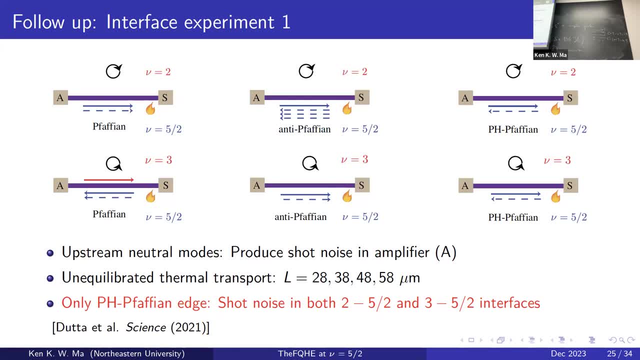 if you look at this, six speakers okay. if it is a five-field, okay. in this two and five-half interface you don't have short noise. but in this three five-halves state you have In anti-barking the situation is reversed right. 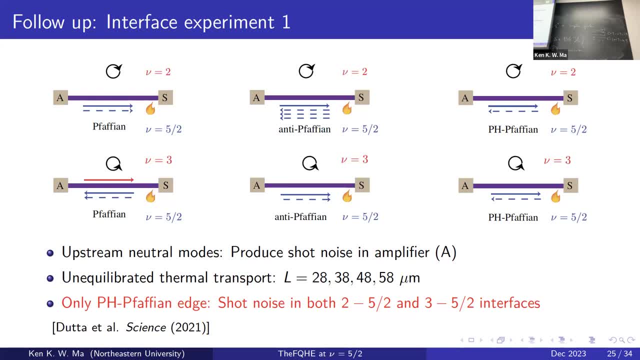 Because in this three five-halves you don't have upstream. that's why you don't have excess noise here, but here you have upstream. that's why you expect so much. But for PH5 and H, okay, there's special properties that are in both two-five-halves. 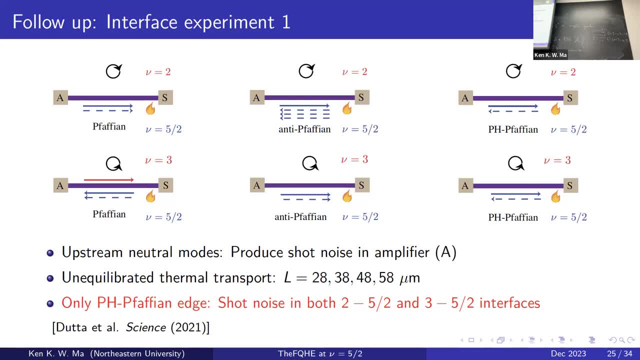 and three-five-halves interface that are an upstream. that's what you expect to have: excess talk noise, okay, being detected in both interfaces And actually it is the case in experiment. It is the case in the experiment, yeah. 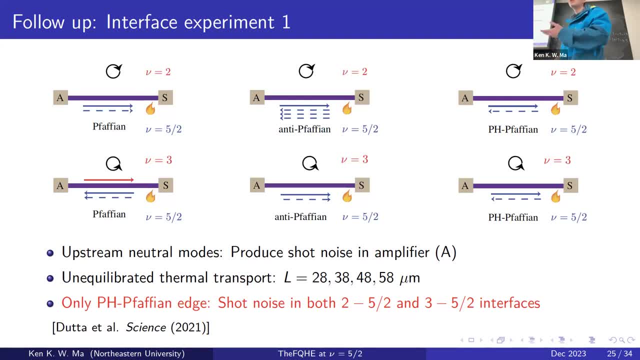 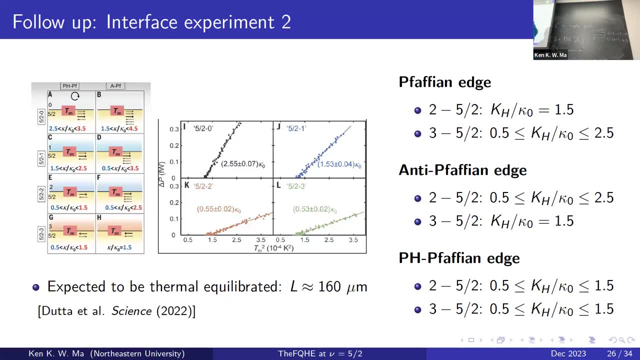 That's why another evidence: It's okay suggesting that the edge is maybe pH 500, okay. And then they also carry out the second follow-up experiment and then try to yeah, Yeah, and then they do the second follow-up experiment. 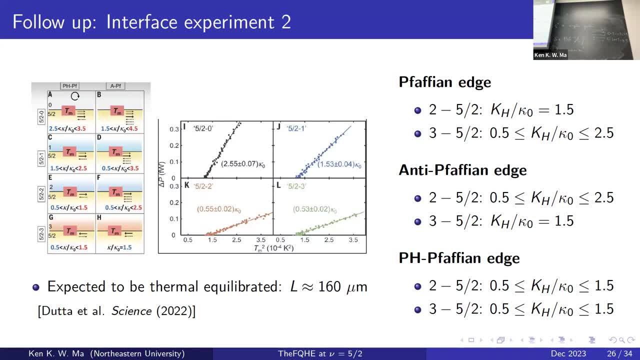 Same time it's running out. I will tell you what they are doing. is they now not measuring the noise? but it's measuring, like the thermal hall inductance or the remaining modes. okay, the same interfaces. right, It's still the 5.5-2 and 5.5-3 interfaces. 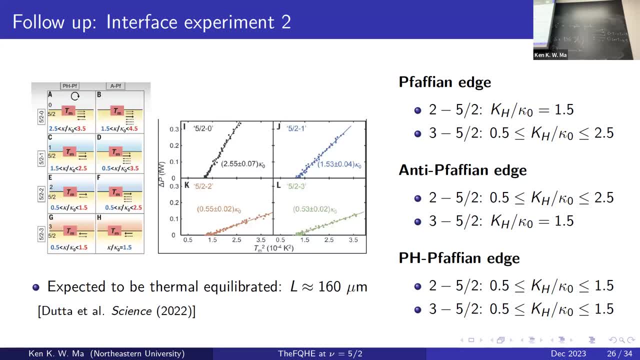 And then they measure the thermal hall inductances. okay. But now let's say, in the anti-phi field- okay, this one, you have a kind of propagating modes. That's why it may be fully degraded or nothing degraded, That's why it's a value in between. 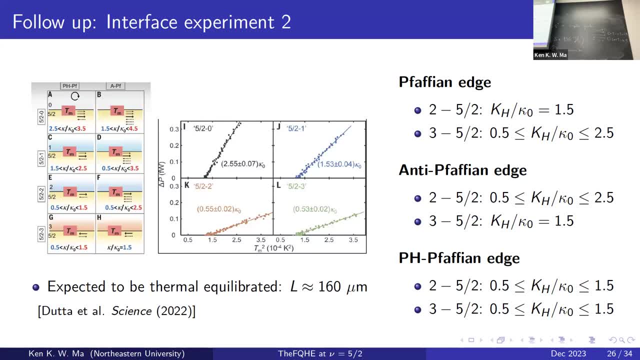 2.5 and 2.5 again, because you may have one minus 1.5, but in this experiment they cannot tell positive and negative value. That's why one and 1.5, when you subtract it is 0.5.. 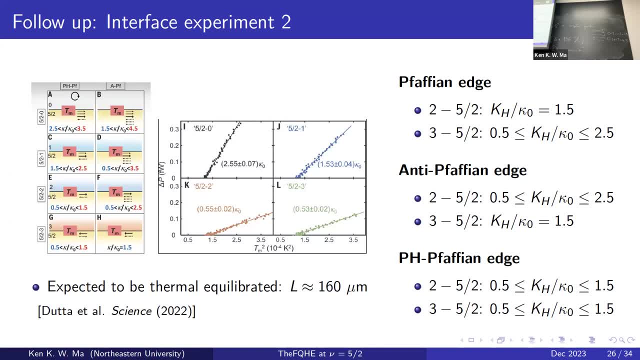 But if nothing degraded, then what you get is one plus 1.5, that is 2.5. That's why you expect to have any value in between these two. if the edge is anti-phi, let's say it's that way. 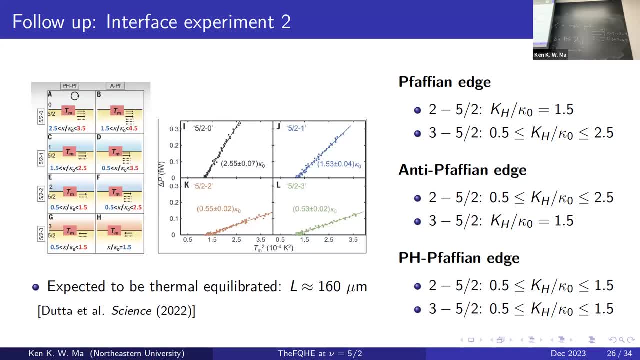 But if the edge is pH 5, then you expect in both interfaces, then you will have a bound, let's say from 0.5 to 1.5.. But for anti-phi, if you go to the interface, 5.5 and 3,. 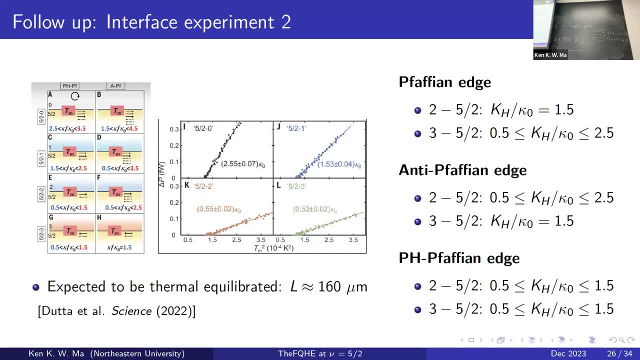 then you don't expect here to have this value. You will have a more definite value. that is 1.5, okay, But in experiment, what they measure? they measure in both 5.5-2 and 5.5-3 interfaces. 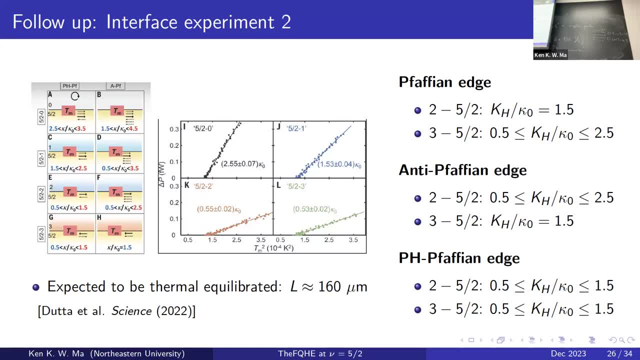 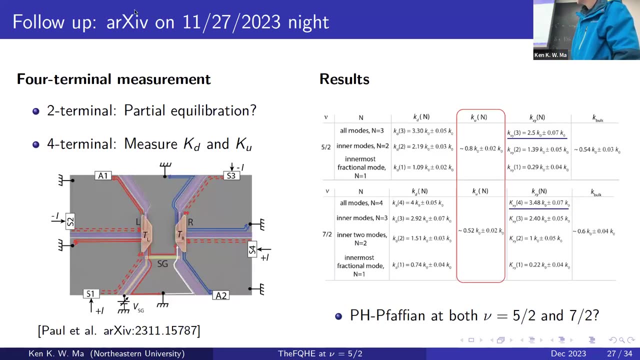 they get something in between 0.5 and 1.5.. That's why it's another signal that probably the edge is pH 5.. And then this one, I think how to close it. This one is like several days ago on archive okay. 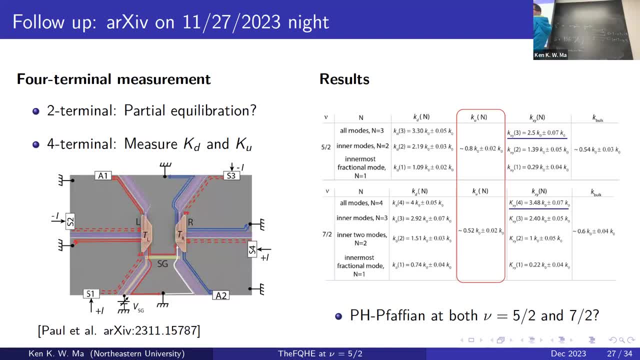 I'm lucky that I check archive every day, So it's archive several days ago. What they are doing is like four-terminal measurement, So now they can separate downstream contribution and upstream contribution for the thermal conductance, and then they measure okay. 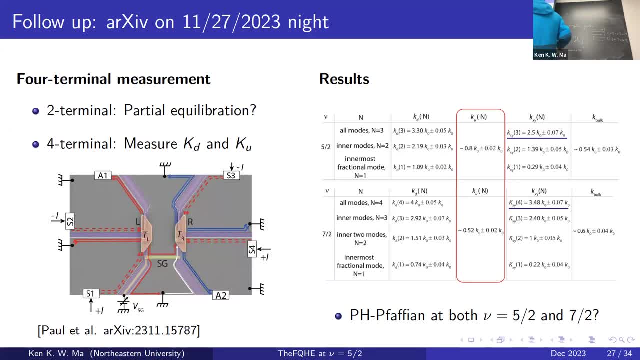 And you can see for the downstream okay, because all possibilities have three downstream mode. three downstream mode right. That's why you see three right. when they open, all the downstream mode is free, But now the upstream mode, what they get okay is 0.8.. 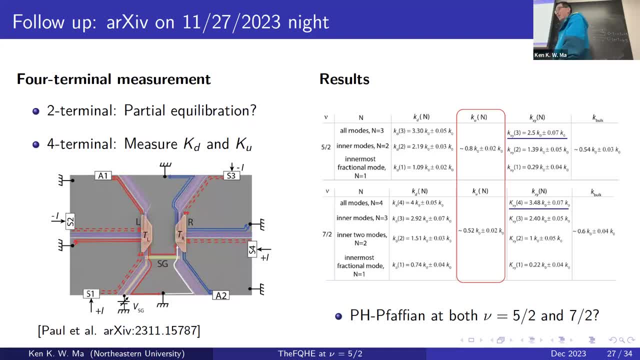 0.8.. So, and they have evidence that probably the edge is pH 5 here. They also do …. they also did the same experiment at Führenfaller's seven-half. okay, They also see how it will create the edge of pH 5 here. 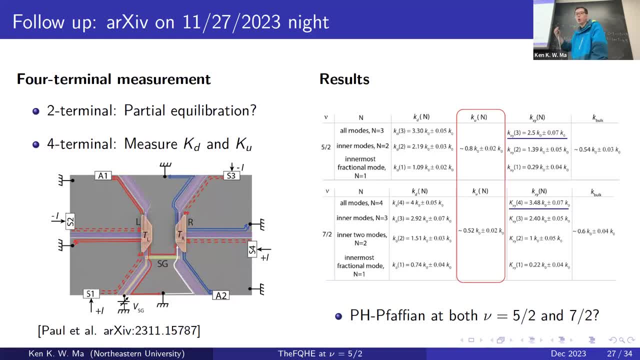 Yes, because seven-half- it seems like people discuss it rarely- compared to five-half. So, however, it's even crawler. they'll find that, at least in this experiment. yes, but there are some bulk contribution they need to take care of. yeah, Yeah, but I think the message is like: it seems like there are, there is an increasing 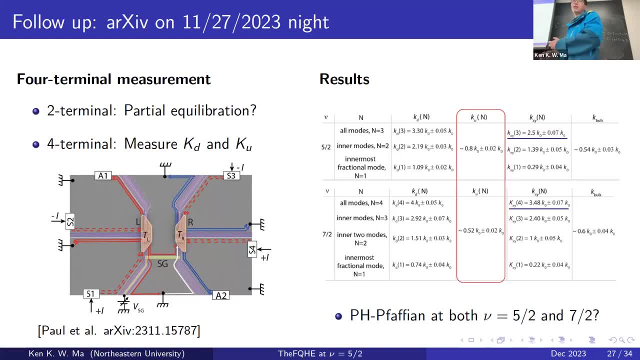 number of experiments showing that the edge, okay, is more like pH 5 here. That's why we probably need to you know, understand it better, why it is the case. But don't ask me about the bulk. okay, As I said, there are different possibilities. okay, That's why it goes to the last part of my 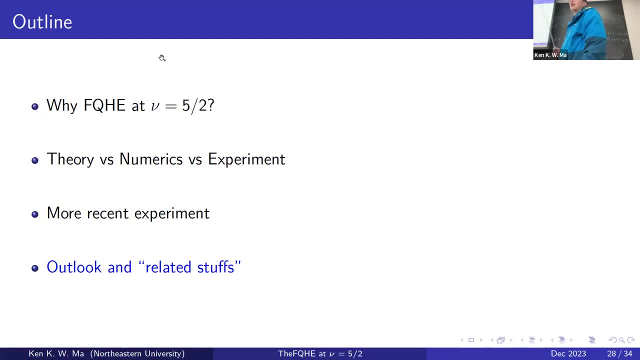 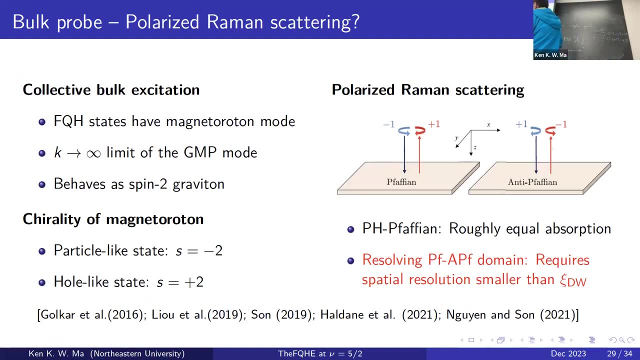 talk What can be done. okay. Let's say, if you want to pin down the ratio of the bulk, okay. So what can we do? Let's say one of the possibilities is to use a polarized round-line scattering. It's like you send a photon and then you get another photon out. 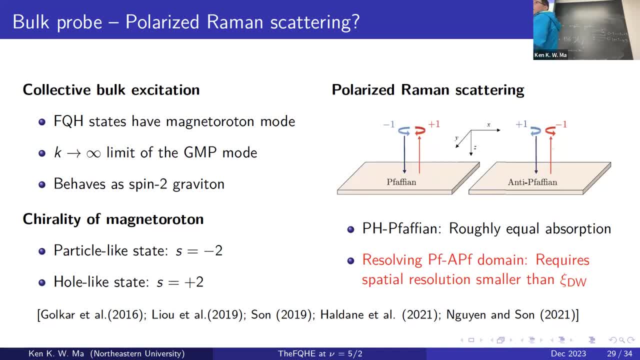 So in quantum physics we talk about the bulk. There is a collective excitation. It's called the Gerven-Madonna-Pasman mode. This GMP mode is neutral and it's more like creating a pair of quasi-particle and quasi-hole. 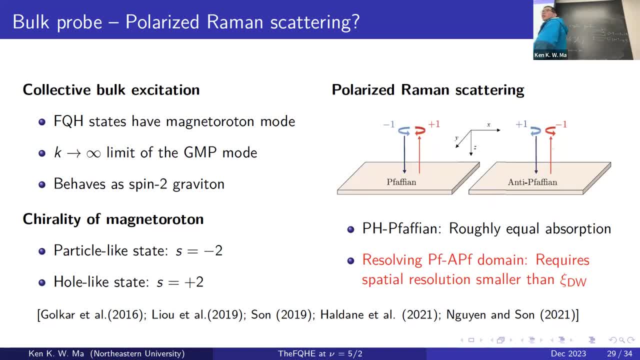 So, depending on the ratio of your fundamental state, let's say, if it is a Fafian state, then that GMP mode in the long wavelength limit is more like a chiral graviton okay, Graviton okay With a chirality negative 2.. So if you want to excite it, let's say by this Raman scattering. 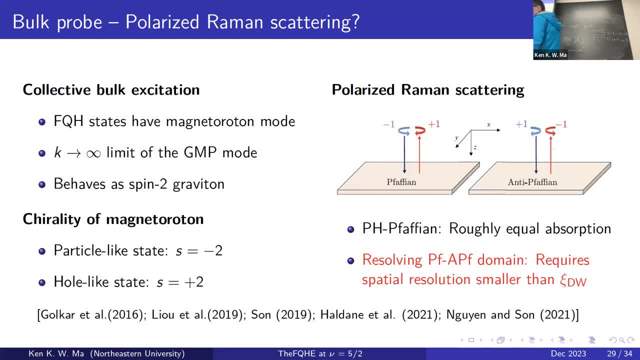 what you need to do is you need to send. you need to send a photon, okay, With polarization negative 1.. And then you need to get back a photon with polarization plus 1.. That's why you transfer a photon with polarization negative 2, such that you can excite. 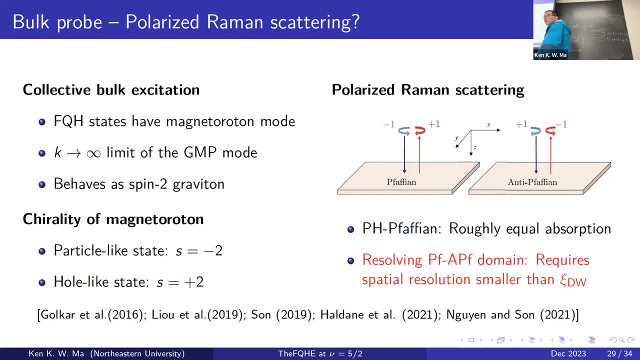 this negative 2 graviton okay, But in anti-Fafian, because anti-Fafian is the particle-hole conjugate of the Fafian. that's why that GMP mode in the long wavelength limit, okay, That's graviton, The chirality is actually plus 2. That's why 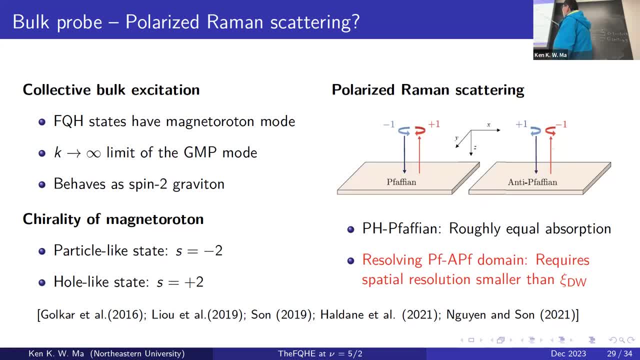 if you want to excite this, okay, then what you do is you send a photon with priority plus 1, and then you will receive a photon negative 1, such that you transfer a plus 2, right, Such that you can excite this plus 2 graviton, okay. Okay, here is a pi over k equals 0 limit. 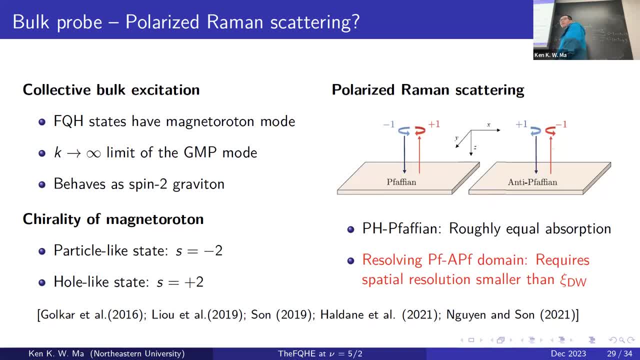 Yeah, it's a pi over. yes, yes, yes. Long wavelength limit okay means that you know it's too high with a lambda right. Yes, yes, Yeah, that's that's why it should be 0.. 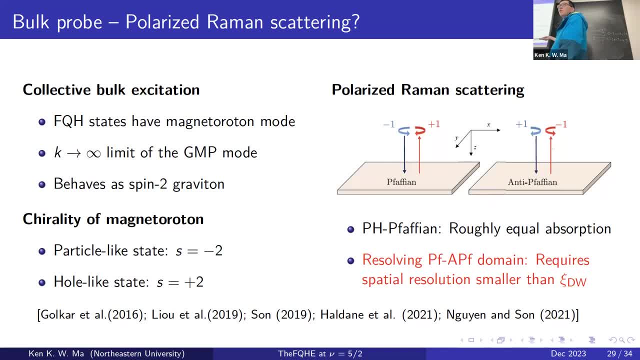 So how about pH-Fafian, pH-Fafian? well, you may either see both peaks or you don't see any peak, right? Because it's not particle-like, it's not hole-like right? That's why it should not have. 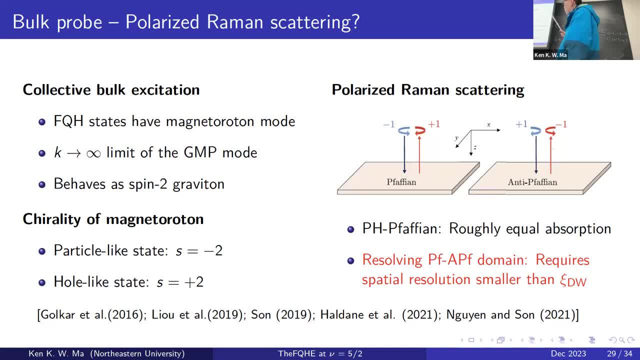 any light chirality for the GMP mode. okay. That's why, if you do this kind of experiment, you shouldn't see a particular peak, let's say plus 2 or negative 2. You may see two peaks or you see no peak. okay. So then you may ask me: okay, how about can I use this one to probe? 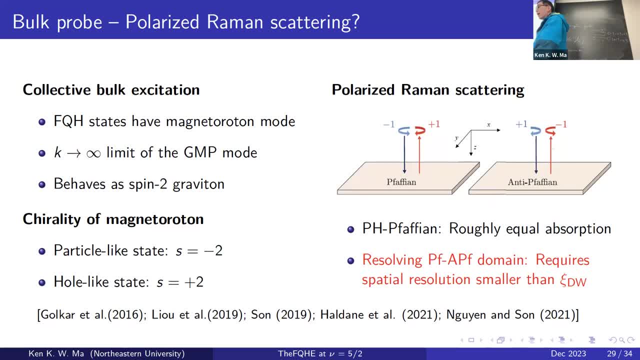 the proposal that has Fafian and Ni-Fafian domains in the bulk. It is possible if the wavelength of the light that you send in is smaller than the size of the domain, right? So that's why this one, if okay, if people can do it. 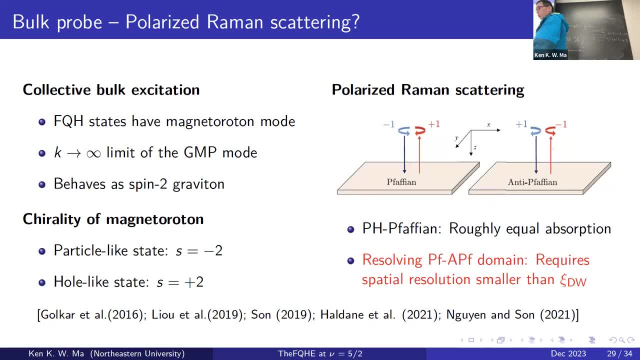 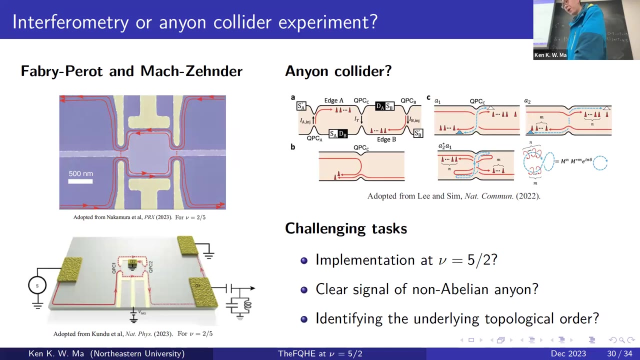 then probably it's a way to you know to tell you more about the bulk. okay, Numerically, yes, I think. I think, yes, I can show you the paper. yeah, I didn't predict that. yes, yes, Yeah. and then another, maybe related direction is: can you do interferometry? 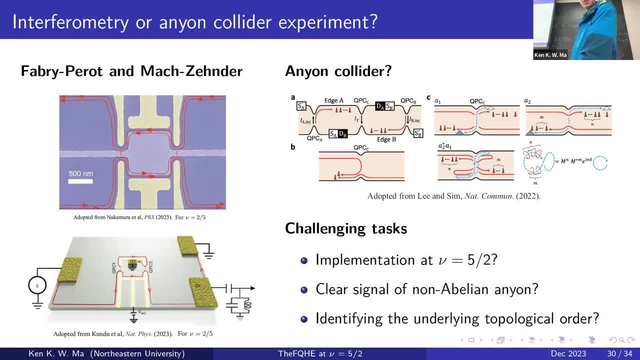 But of course this was very, very challenging because you know, recently let's say people have do some N-neon collider and then see some more direct evidence for N-neon statistics, let's say in the Laughlin state. And then let's say the group Mind Manifold at Purdue. 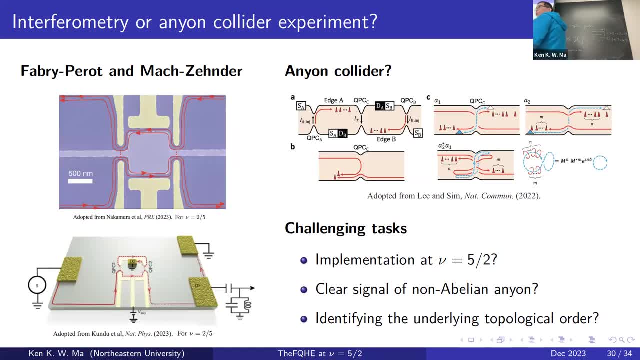 they do a 30-per-watt and then they get a better signal showing one-third and two-fifth okay. And then let's say, in Weizmann Insecting Group they do another kind of interferometry experiment- it's the Max-Zehnder one- and then they do this two-fifth okay. 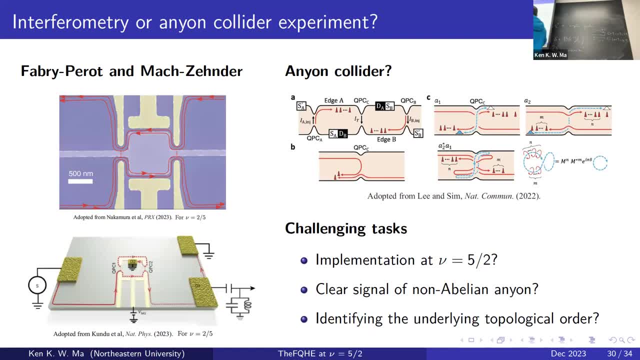 Not five-half yet, okay. Not five-half yet, okay. So maybe eventually they can do it, okay. And then this one is a theoretical paper that shows that the so-called Fennel factors are different if you have NF-F-N and H-F-N. yeah, But I will skip the details, but just telling you that. 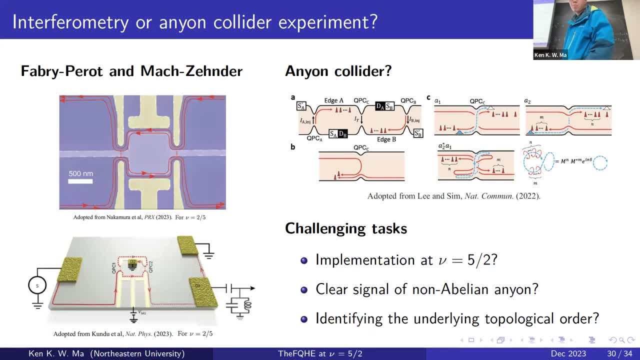 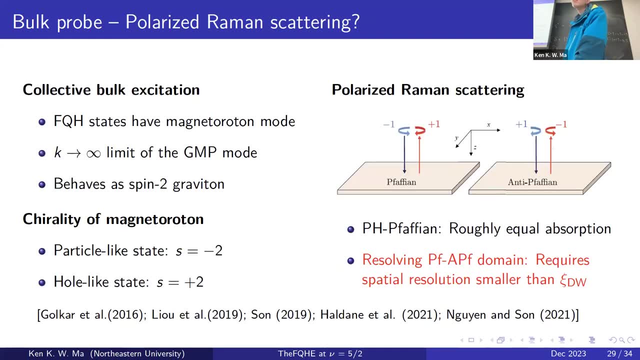 yeah, if you are interested, you can go to this paper. yeah, Yeah, go on, You can try. Yeah, k goes to zero. yeah, k goes to zero. yeah, Yeah, long wavelength limit right. That's why two power over lambda, right. 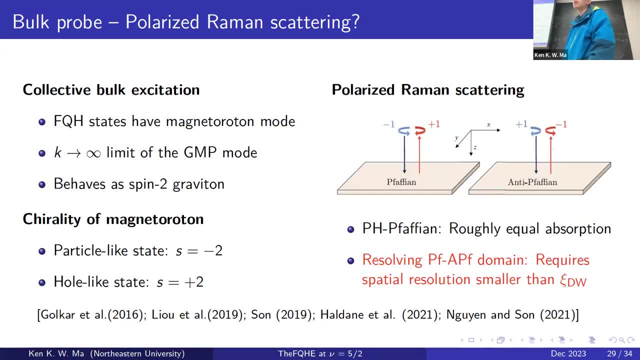 Yes, it's been to excitation. yes, Sorry, No charge, right, Because it's like a neutral, it's a collective excitation. it's more like you excite one quasi-particle and one quasi-hole. that's why it's neutral. 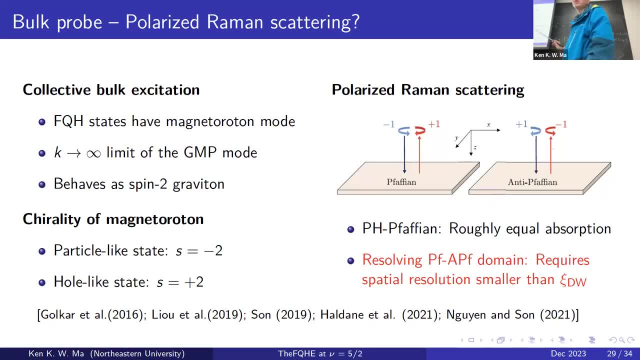 Okay, so you are more expert in that right. Yeah yeah. GMP- yeah Okay. What's the condition that graph is going on? Well, I see, it's not the graph that's showing up, it's like 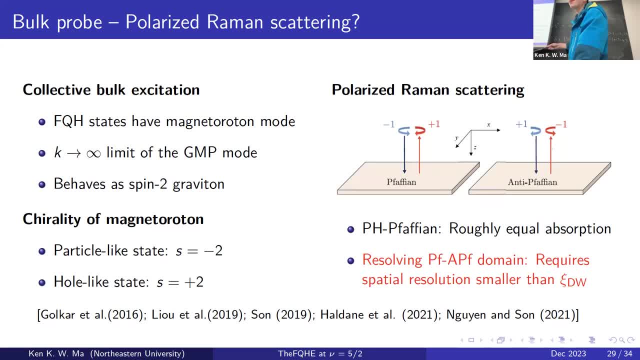 it's like if you look at, let's say, the absorption spectrum, something like that, which block pit, will you see if you use a different, different polarization of photon when you shoot it there? Because what you want to do is that you 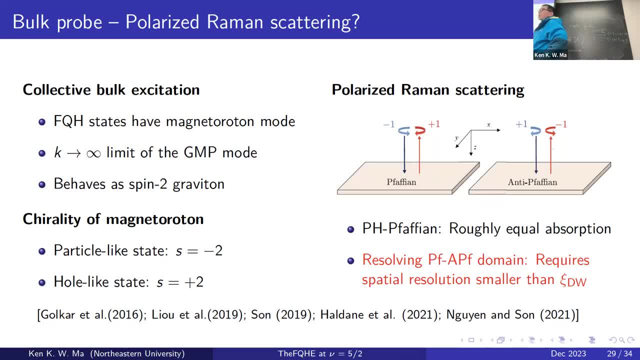 want to excite this graph at one right. Let's say, if the graph at one is priority minus two, then you want to transfer a photon polarization minus two. That's why you send minus one and then you want to receive plus one, such that you transfer minus two to excite this. 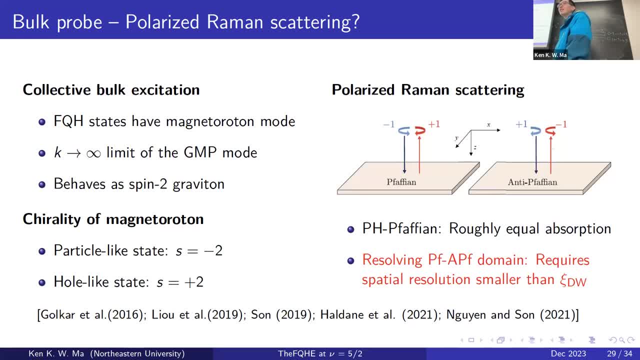 While you are asking another thing, sorry, Okay. so if you were going in any, any, any fundamental space, for example, oh this one, this one, okay. here I focus on far-framed and anti-far-framed. 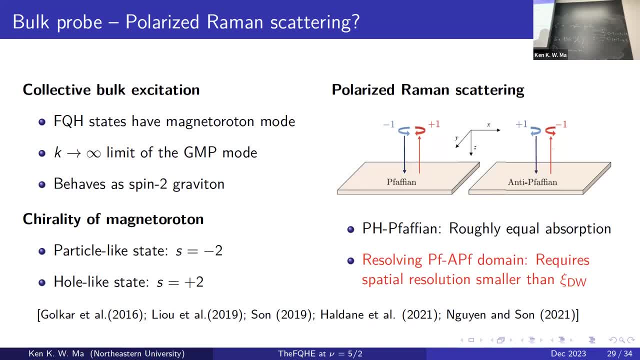 okay. so this one is for far-framed, this one is for anti-far-framed, but in general this also holds. let's say in the Laughlin state, that field length factor: one-third. okay. the GMP mode in the long wavelength limit it behaves at chirality negative two graph time. 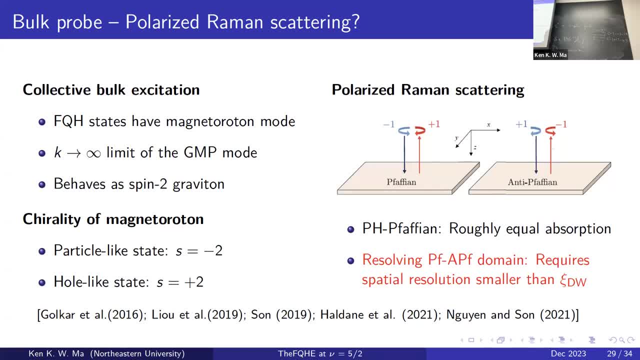 But let's say you take the particle conjugate of that new new equals to one-third, we go to two-thirds. then that GMP mode, okay, in the long wavelength limit it behaves. let's pass two graph points. yeah, generally holds. 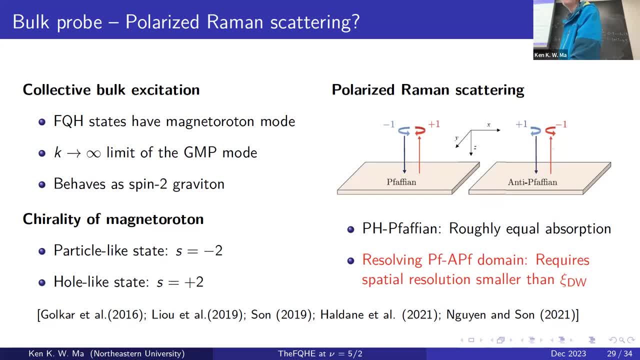 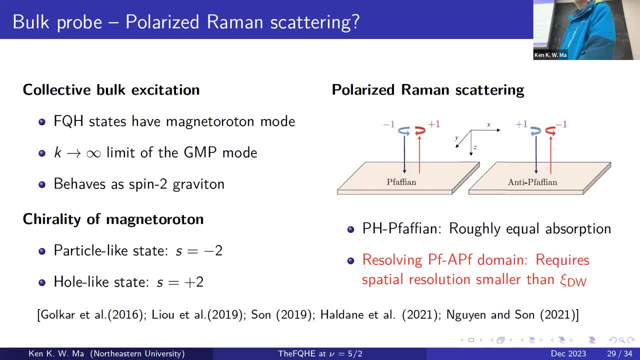 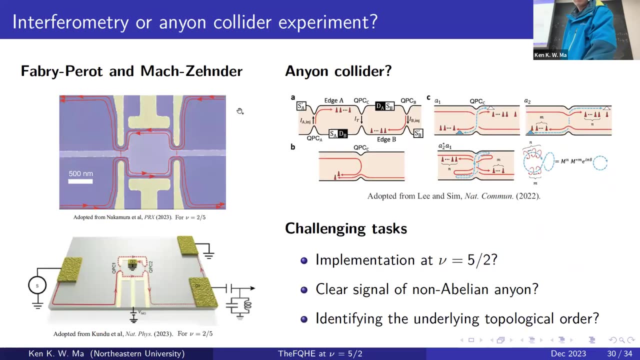 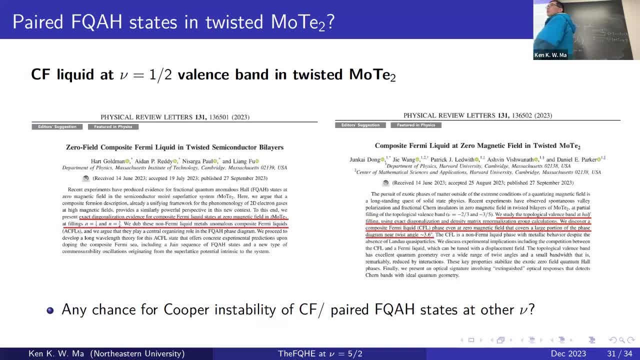 one in quotation marks. okay, so recently I'm very interested in twisted TRIST-MOTE2.. The reason is that there are two groups of people- okay, one of them is actually the audience- and then they show that. actually, if you look at this TRIST-MOTE2, they have a fusion factor of, let's say, one half. they have a single-field composite fermion, but it's also a composite fermion electron. 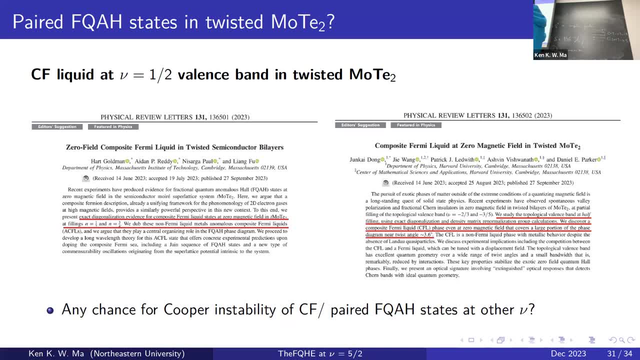 So I want to ask a question is: is it possible to have similar physics, let's say, in gallium acetylene? Is there any fusion factor? Let's say, if you pop up in higher chain bands, I don't know. 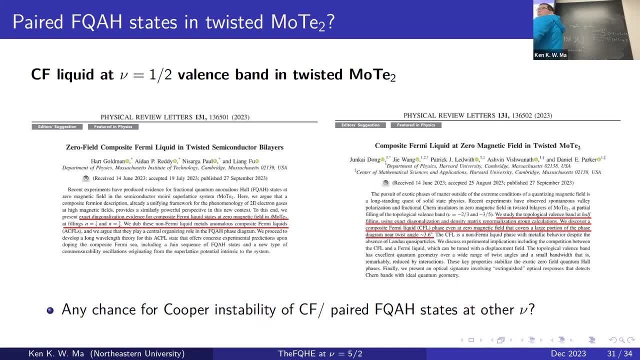 okay, just guess, Is it possible to also have Cooper instability? And then, is it possible for these kind of composite fermions to pair up and then show you some non-linear fractional quantum anomalous force state Possible? I don't know, I'm not an expert in this direction, but I find this: 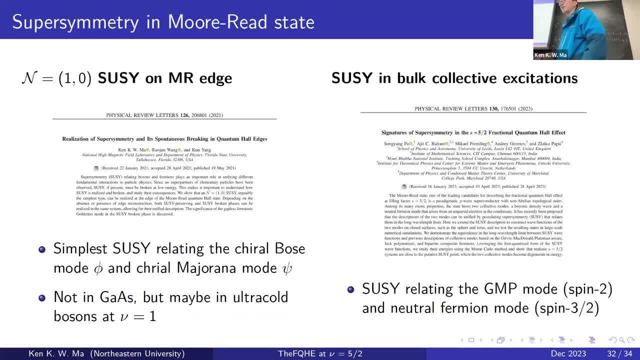 question interesting. Another one: as I spend most of my time okay of reviewing things, I think it's fair enough. I just spend one slide okay for advertisement of my results. okay, So let's say we talk about Morbid Edge. Actually, this morning we discussed this. Actually, you can utilize supersymmetry on 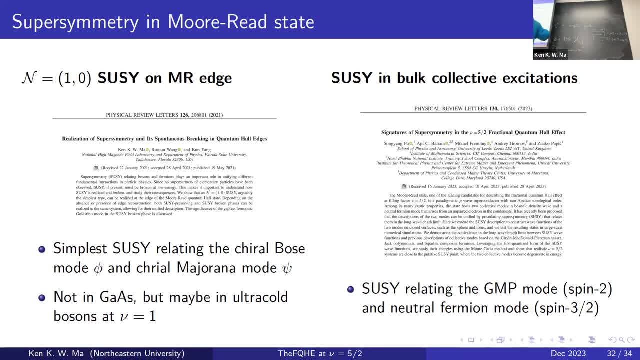 the edge, Another group of people. they also show that, let's say, you focus on Morbid State and look at the bulk, the GMP mode and the neutral fermion mode. They are also supersymmetric powers. okay, So it seems like five-half state or its related. 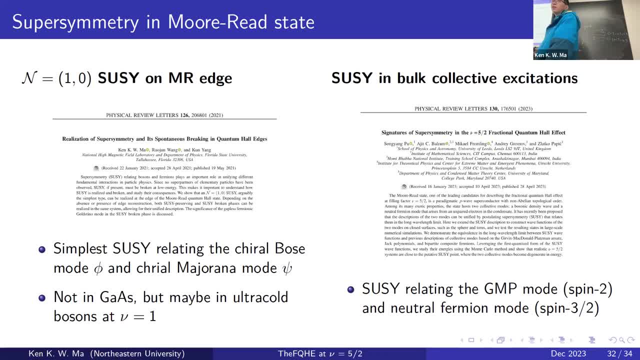 topological orders. there are very, very rich physics, right. You have gravitons, you have anions, you have non-Libyan anions, you have supersymmetry. basically everything, okay, Basically everything. Yeah, maybe you can also have a black hole, information paradox, okay. 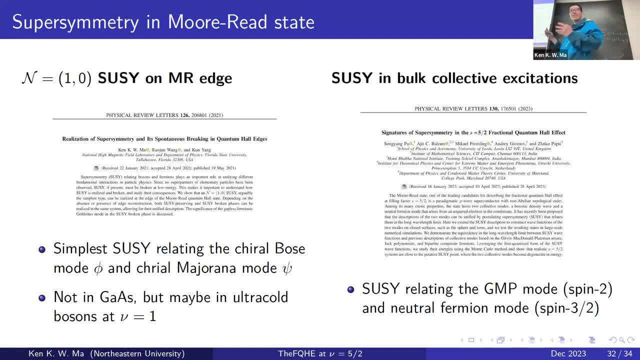 which I actually wrote a paper. but I don't think I I don't think it's a good idea to advertise my work too much, and then if I need to advertise everything, probably you need to invite me three times where to give free talk. okay. 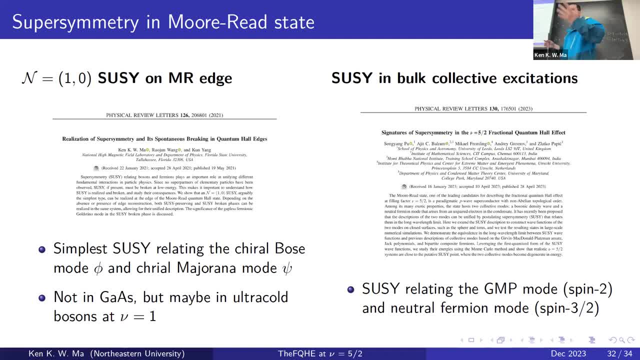 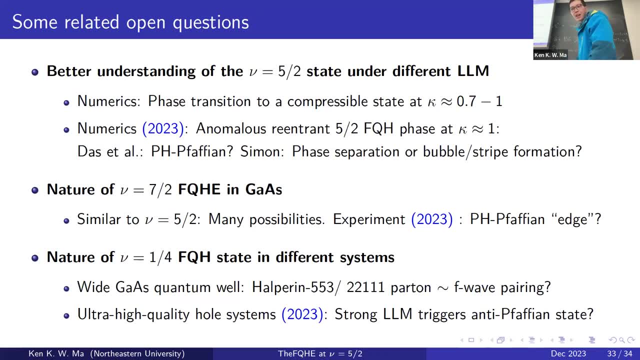 If you invite me, I will come, because I have free lunch and free dinner. so Okay, yeah. and then another greater question is like in the numerics, as I said, okay, when you increase the Landau level mixing parameter, actually there is a phase transition, they observe. 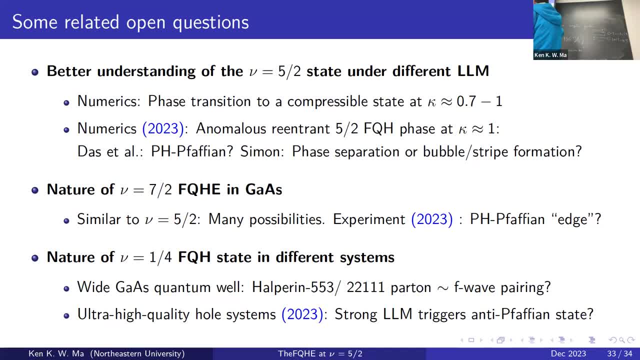 and then, Let's say, at a Landau level parameter around one, they see a anomalous threshold, compost state. claim: anomalous state, okay. Then they also claim okay, because these kappa is about one. you see the state that really describes the experimental cell. 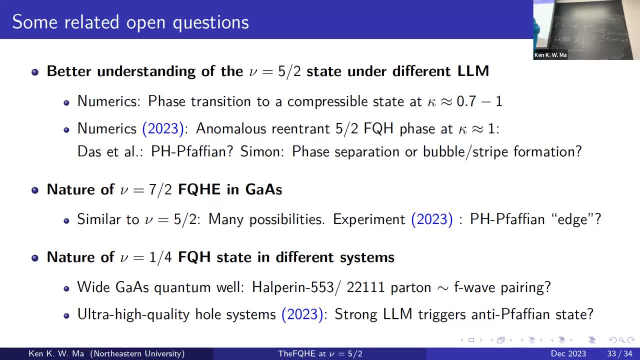 If that's true, is that anomalous state corresponds to pH 5-ion or anti-5-ion 5-ion domain. So this is this is one of the conclusions they made, and then after that, Steve Simon put a comment. 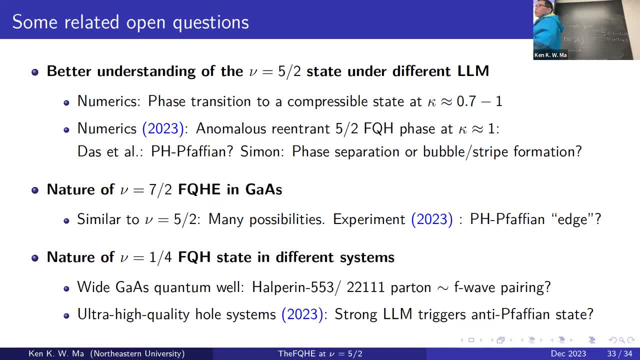 probably this is just like phase separation, or bubble, or striped formation. okay, Which one is correct, I don't know. yeah, but I just want to you know, introduce you that they are still developing, you know, developing investigations. And then for the ratio of 7.5, as I also 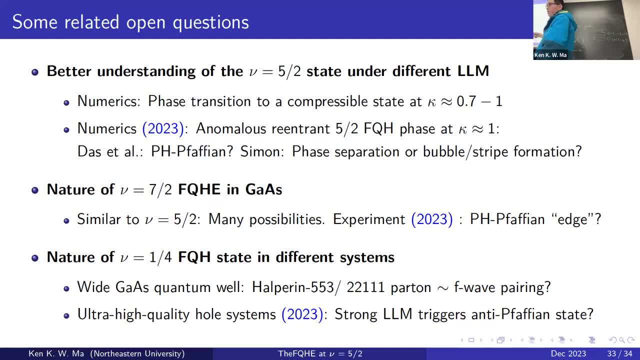 tell you is, but also told you is that several days ago, that experiment suggests that probably the edge is also pH 5-ion-like. okay, So then we can also ask the same question as the 5-half. actually, what happens there? 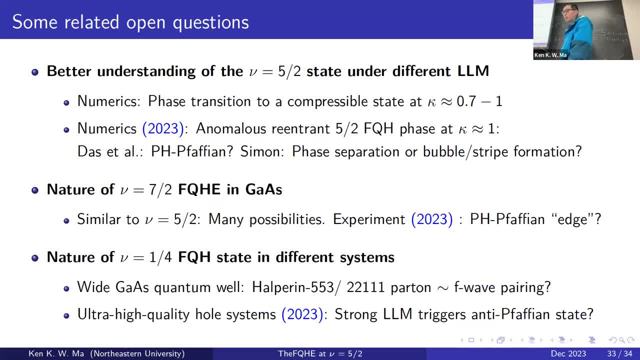 right. And then not only, not only, 5-half is the even denominator of threshold compost state. we observe actually one-fourth, okay, One-fourth, in different materials, Let's say in garden arsenide, if the quantum well, is not Y actually, you see, kappa state. 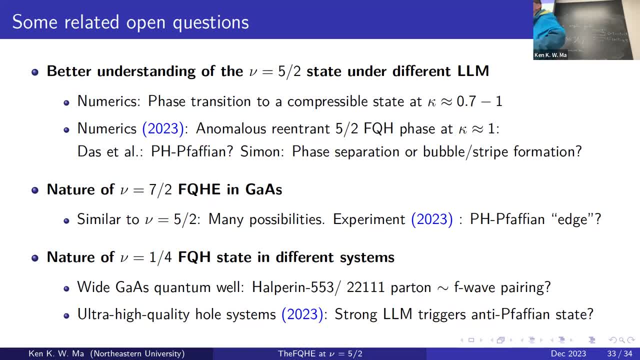 the quantum. well, by and large, Y is Y- tame amount. So you see the kappa state, and then again it's very similar to 5-half state. you have different possibilities. One of them, let's say the hypon 553, and then you also have different possibilities coming back. 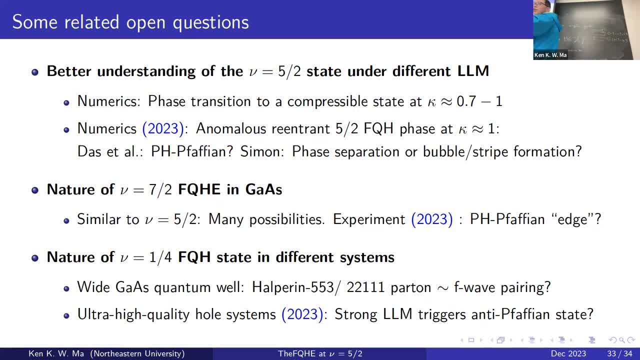 how we pair out those log: two flux composite fermions by four flux composite fermions. That's why you may also get 5-hipn and have 5-hipn give 5-hipn, etc. And then numerically 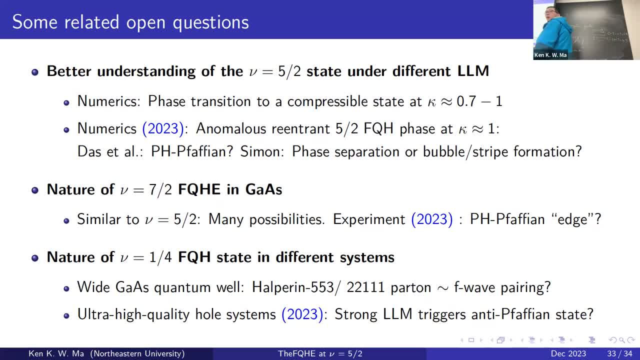 people find out. probably it's more like this part, constant state, you see all these things. When the adiabatics say like multistate, and that I would also say: you know, log, two components and the other things, That's different. Yeah, yeah. So at this point stopped them off. 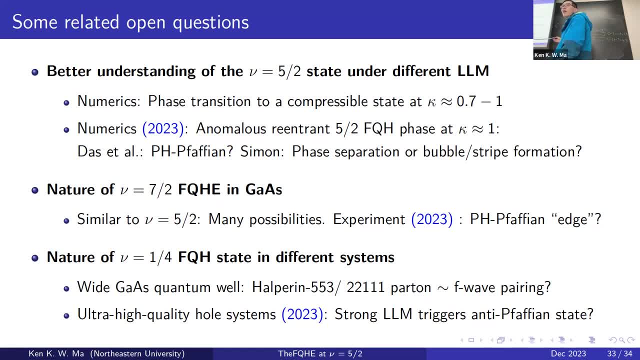 is the F-wave pairing state, But for the 5N, as I said, it's like P-wave pairing. For pH 5N it's also P. And then again several days ago- okay, several days ago- they also observed another system. 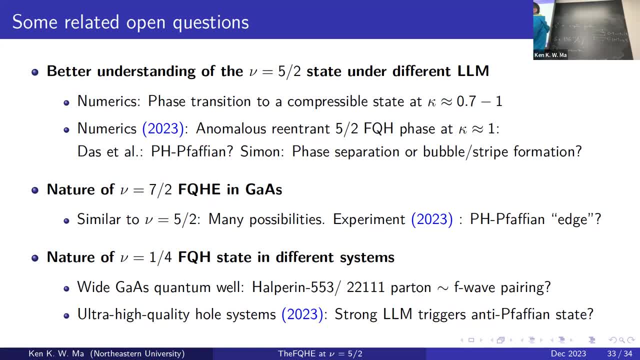 that has one-fourth flexible compound, but now it's locked in Y-guided SNRI quantum well, but in ultra-high quality whole system, okay. The quantum well is locked at Y, okay. And then there is a numerical paper, I think by Jalinger-Jing group, okay. 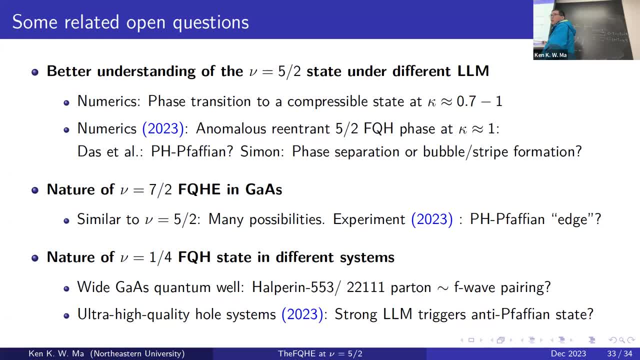 suggesting that probably this strong landau-level mixing. why is this strong? Because the defective mass of the whole is actually much larger than the defective mass of the electron-guided SNRI. That's why the landau-level mixing is much stronger. That's why in that numerical paper, 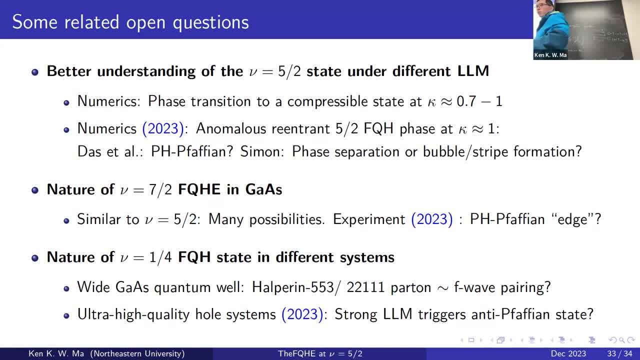 they proposed probably this stronger landau-level mixing. may favor say F-wave pairing, state something like that? Yeah, So you see, there are still many questions that you can ask, right? Yeah, So I am completely overwhelmed, Yeah.